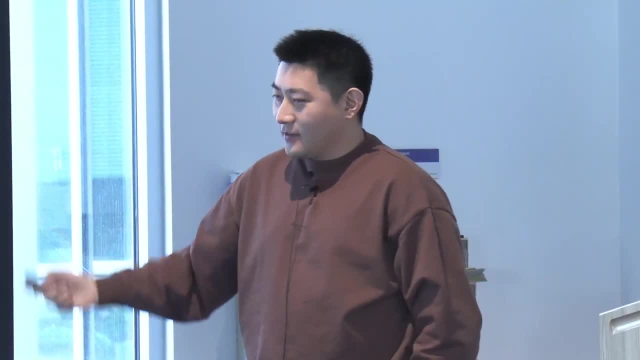 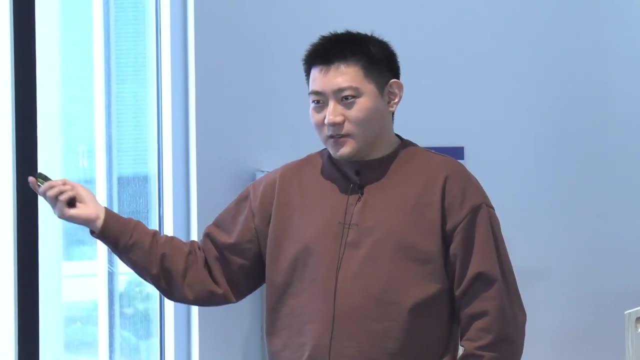 Then they might go into more details. I passed the border at late night So they might ask you like, why people starboard? So I said, okay, let me tell you a secret key for this. So I first met a lot of people in the community that was working on this, because this wasn't 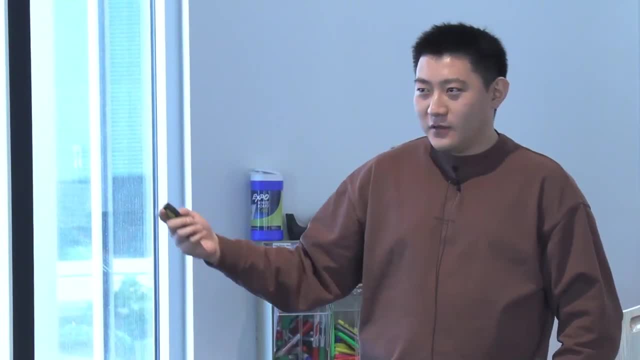 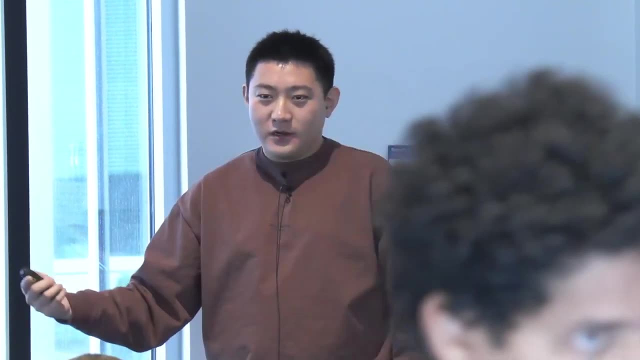 available until 2009.. This is a fairly new field. I was kind of lucky to get into this field in 2012.. My advisor picked this new area and that was just the beginning of this thing, And ever since 2009,. 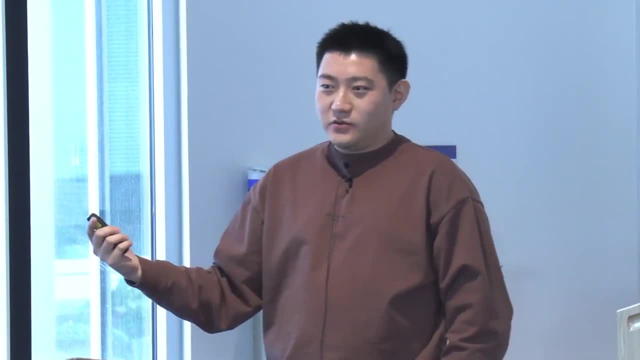 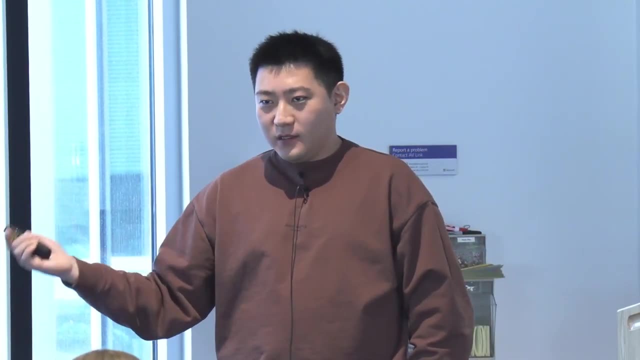 we've witnessed like one order of magnitude every year, kind of Right now, we have 10 to 9 times speed up compared to the first construction in 2009.. And these thanks to- and they will ask you: what do you work on? 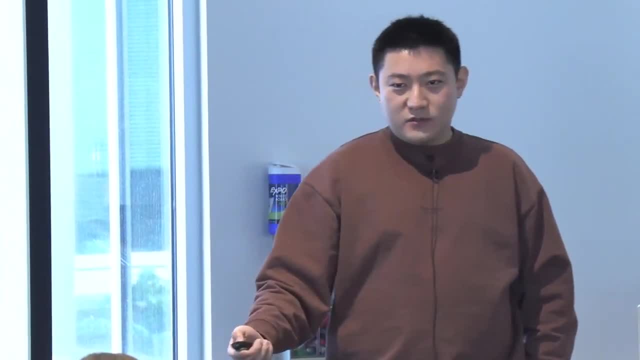 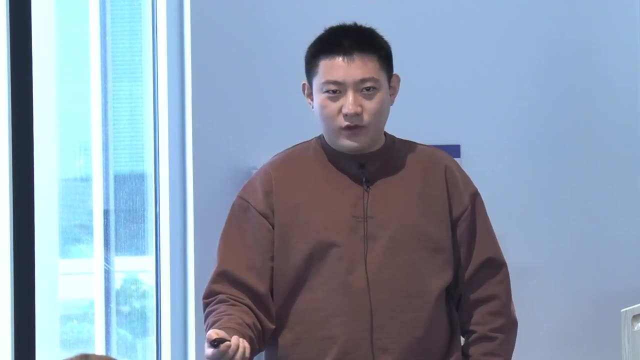 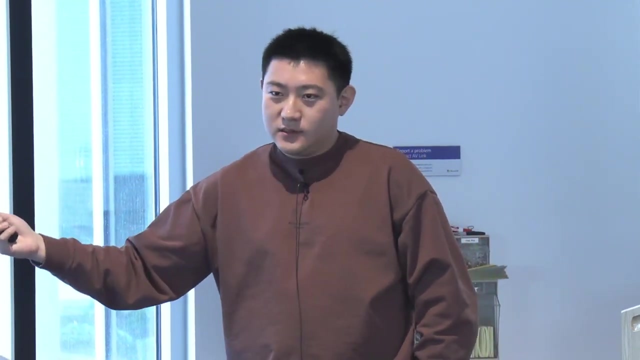 What does all the researchers work on? We brought up new constructions, new schemes, theoretic improvements, even optimizations on the hardware, targeting special hardwares, and we bring the slowdown down to 10 to 3 or 10 to 6. There's a slight difference. 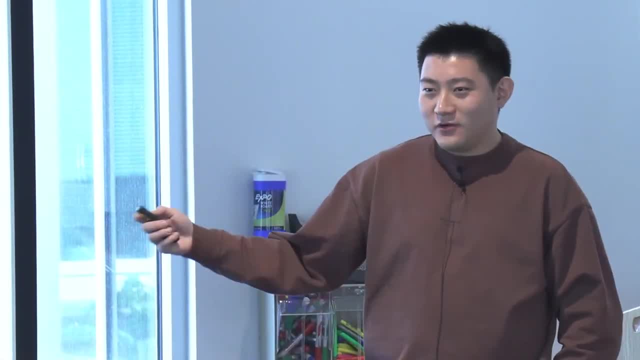 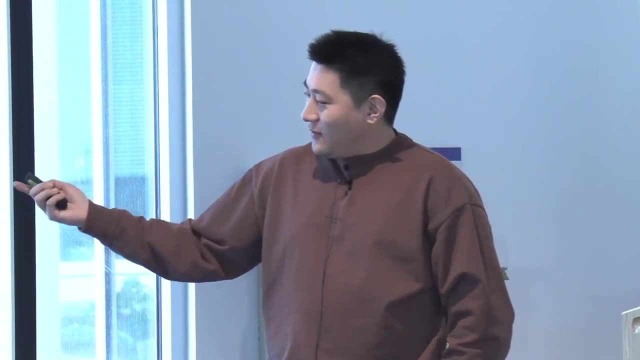 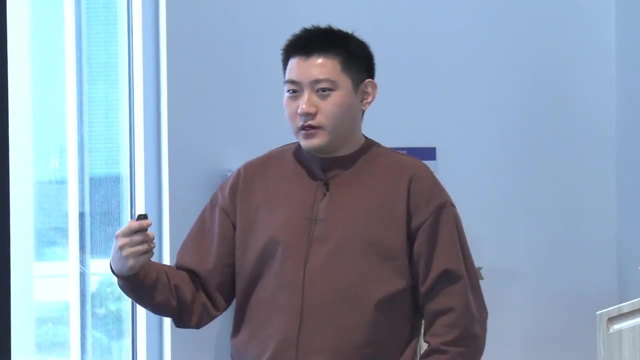 depends on how you use HEE. Maybe you are a bad programmer, or if you didn't understand it well, then you get 10 to 6 times slowdown sometime. The final thing is the target application. scenario is: HEE has a killing app for online secure storage and computation. Good example is that you want to keep your DNA data secret, but you still want to use some of the services. let's say, find your relatives and you can just upload the encrypted version of your DNA to the database and they provide matching those service for you and return you the result. 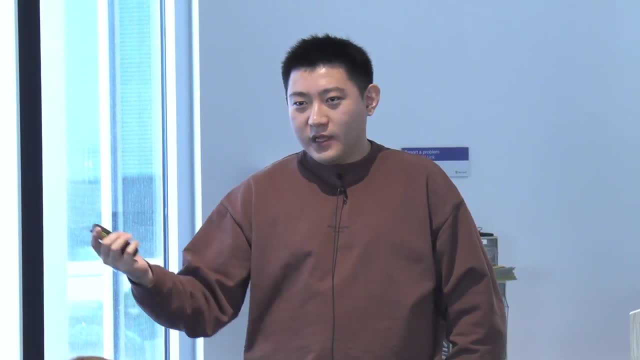 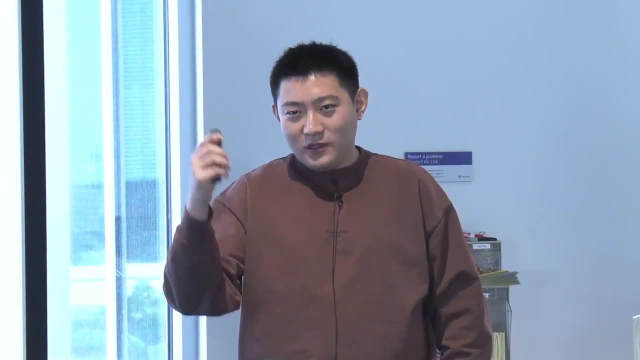 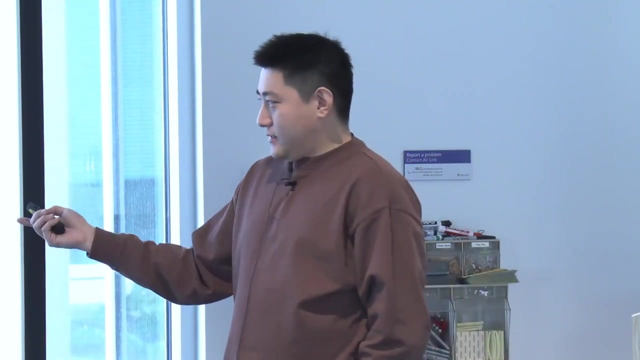 Even whether you have relative or not, you get some result encrypted back. only you can see the result. Maybe someone get empty result, maybe someone get the full list of relatives. they are all encrypted. The service provider knows nothing about it, So this is the ideal scenario. 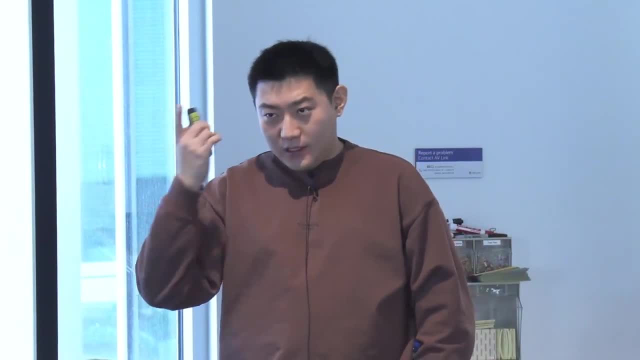 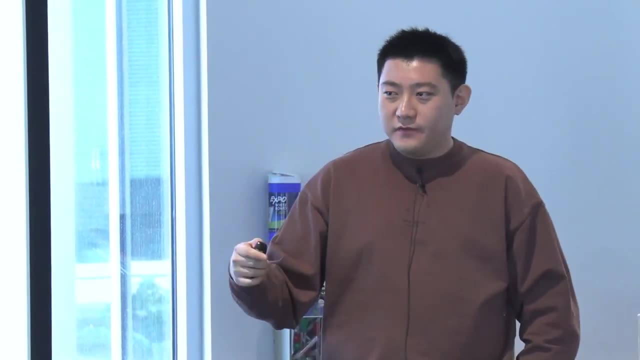 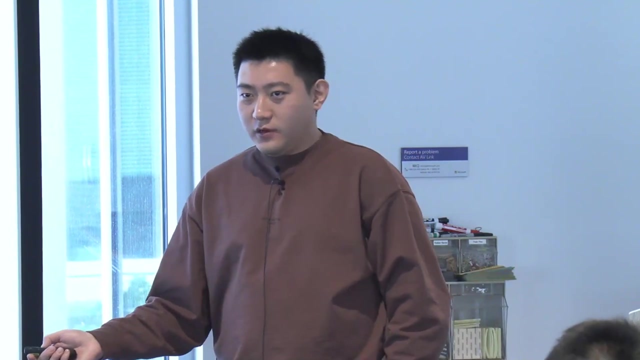 and there might be some real-life application of these. and, for example, if you want to follow the IDASH competition, it spells I-D-A-S-H. They focus the test on genomic data. sometimes There might be some good solutions and there are papers to follow up. 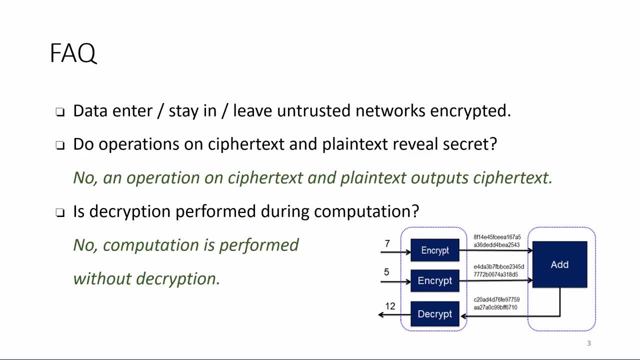 So here are just very frequent questions we got. Let's say first, we assume that there are two zones. One is a safe zone. Let's say, when you do decryption it requires a safe environment. For example, your laptop, That's where you hold a secret key and it's considered safe. 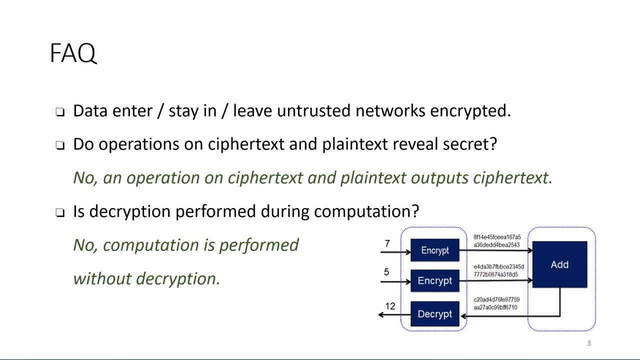 All the data outside the safe zone should be encrypted. I mean, encryption doesn't have to be done by yourself. It can, because there are public key encryption that use a public key. so I can do encryption for you, every one of you. But data outside that safe zone are always encrypted, even the results. 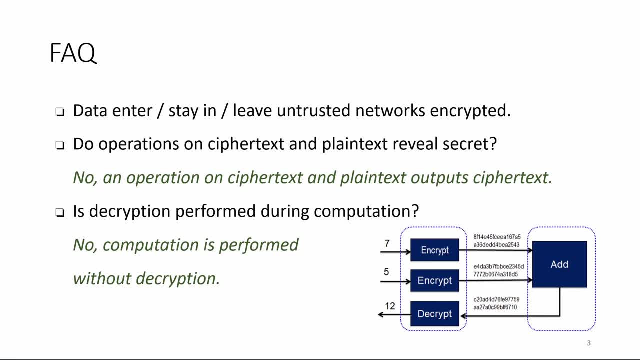 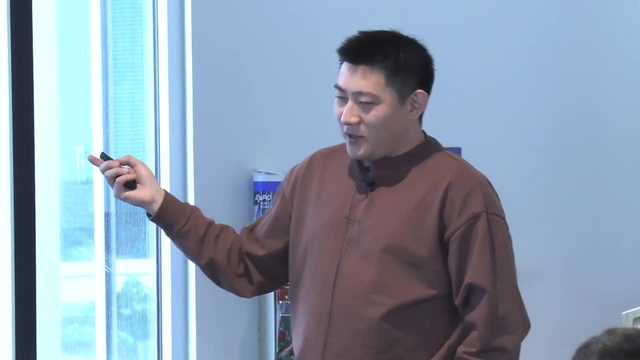 You can see, even if you compute on encrypted data and on unencrypted data, the result is still encrypted. It's like a virus. Once you get encryption there, everything will become encrypted, which is good. Computation is never done. You don't need a secret key to do encryption. 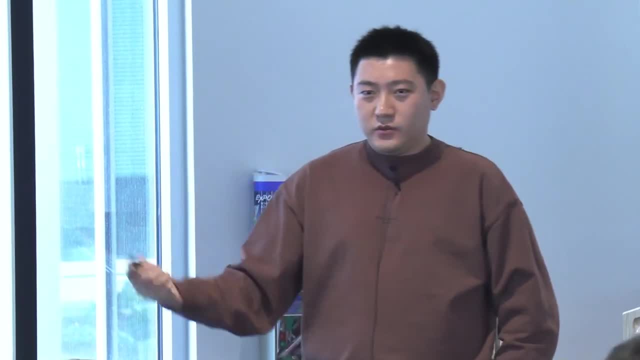 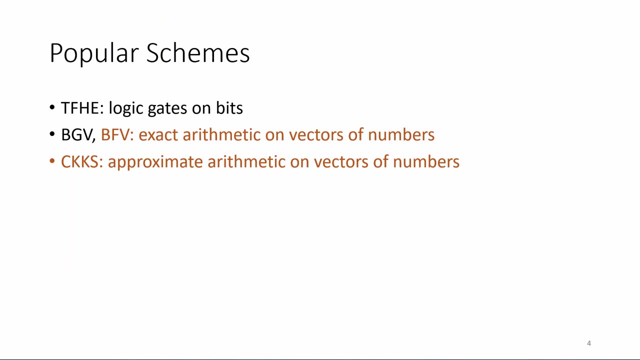 Without a secret key you cannot do decryption that ensure the safety of your data. There are a few popular schemes. These are the most efficient schemes nowadays. I think some of you have worked on TFG related schemes. They focus on logic gates, on bits. It's like redesigning logic circuits. That's one scheme. Then we have BGV and BFV. They perform exact arithmetic on vectors of numbers. So first it's better than just a single value. It's perform vector of values and then they give you the exact result. 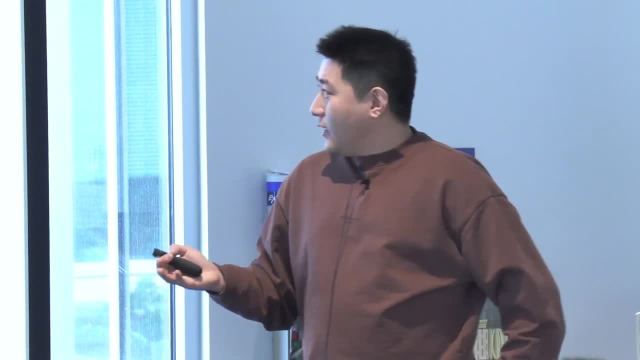 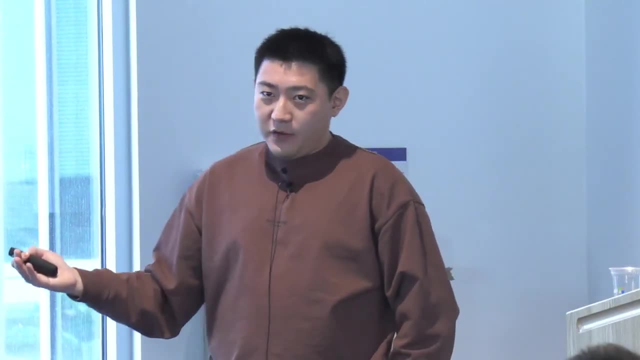 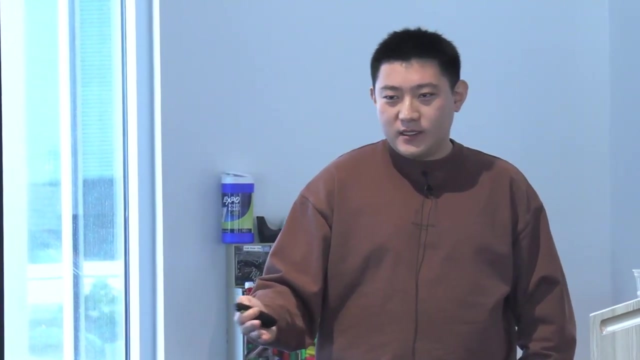 You don't see any error. You don't see approximation. CKKS is a new scheme we'll introduce in the next session. It does approximate arithmetic because at some time you don't want to keep the full precision. If you're in banking, you want to calculate the whole assets of yourself. 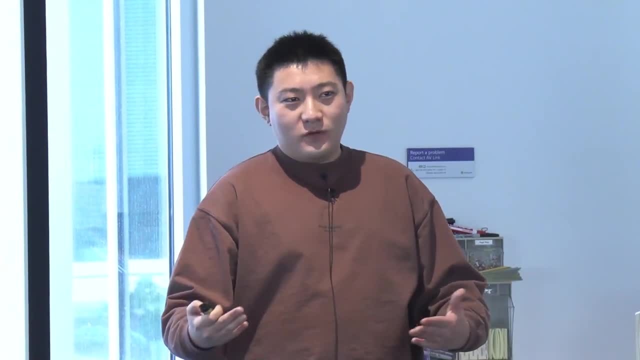 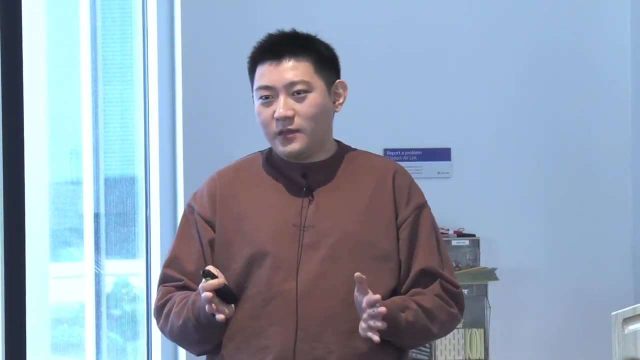 you want to get the full precision. But what if you're doing, let's say, some floating-point arithmetic? let's say you're doing a training or inferencing, you only need maybe eight-bit precision. then CKKS is a better choice if there's approximation involved. 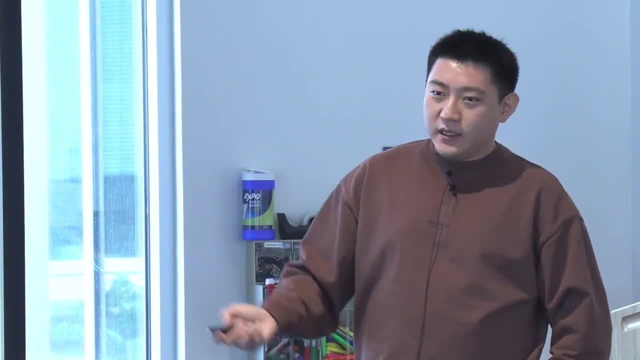 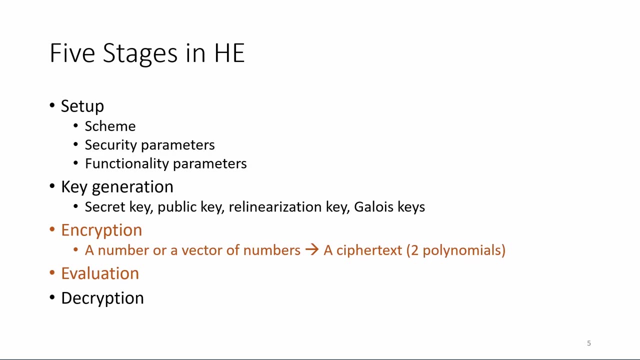 Microsoft CCO implements BFV and CKKS and those two will be the ones we are going to focus on. So there are usually five stage in HE. You can see that in every paper covering HE. So the first one is to set up. 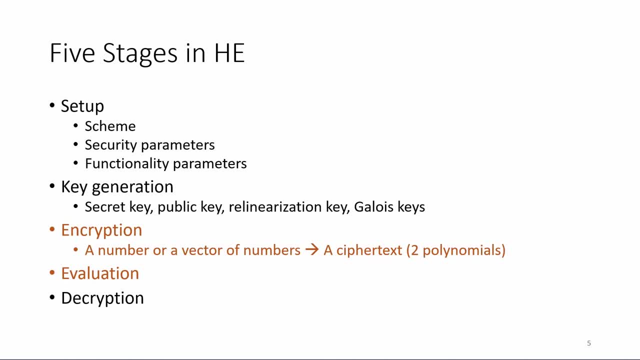 Here I lay out everything in the order when it happens. So first thing is to set up. you need to choose the scheme, you need to choose some security parameters and there's some performance parameters for functionality. Actually, I uploaded these slides to GitHub. 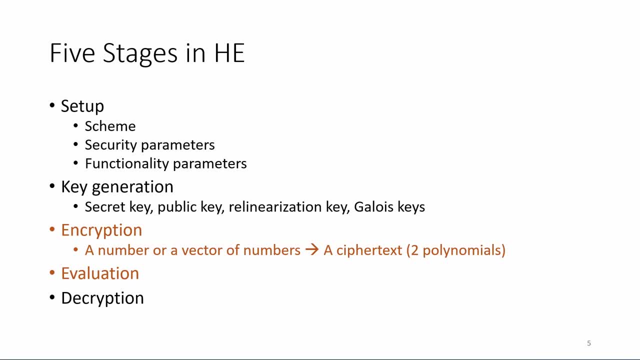 so I will show you the link afterwards at lunchtime so you can download or look at it anytime. Probably this will apply to all the following slides in our technical talks. Then, after you set up the parameters, you can do the key generation. 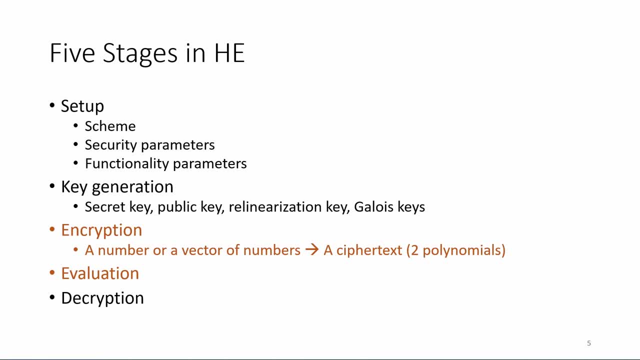 Here. this secret key is the one that you need to protect it. The other three are generated from the secret key and they are all considered public, So you can send these three to anyone and they can never compromise your data. These two are required for computation. 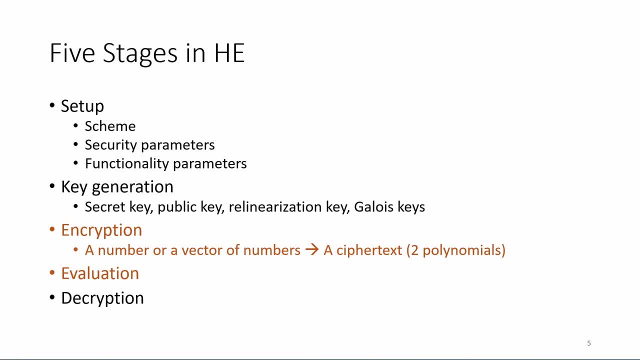 these public key can be used for encryption. Secret key can be used for encryption and decryption. Then next step is to encrypt your data. So here in high-level view, we encrypt the vector of numbers. I'll go into more details about what the numbers look like. 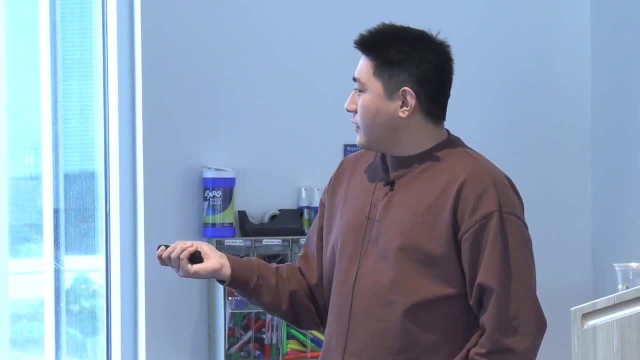 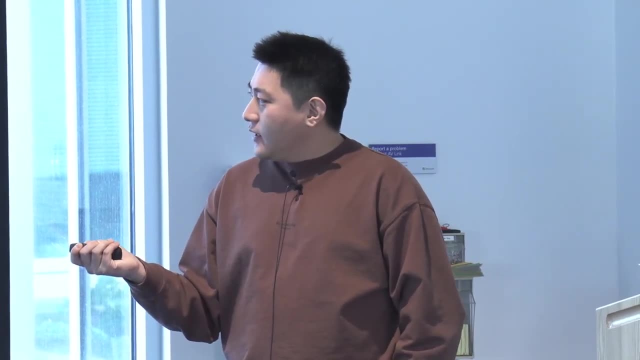 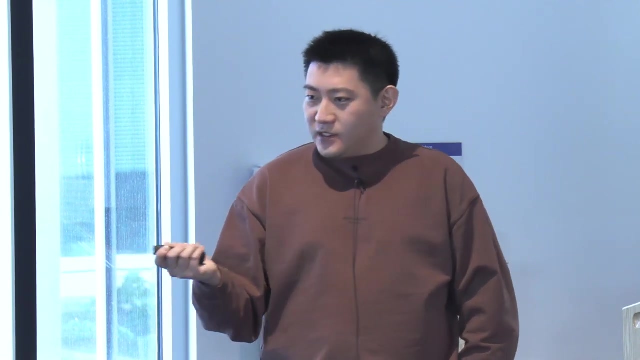 but just a vector of numbers, many of them, and it becomes a ciphertext which is two polynomials. I'll get into that right after this slide. So we want to start with encryption evaluation stage at the beginning. Evaluation is where you really write your program. 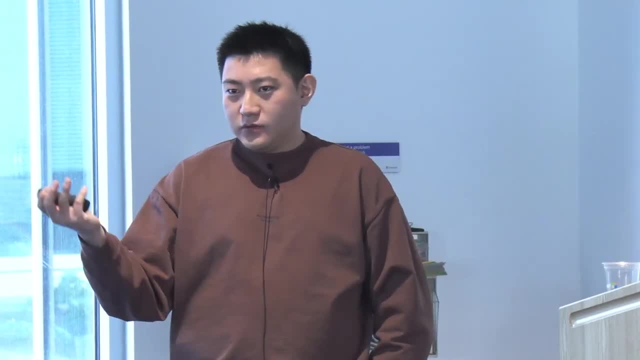 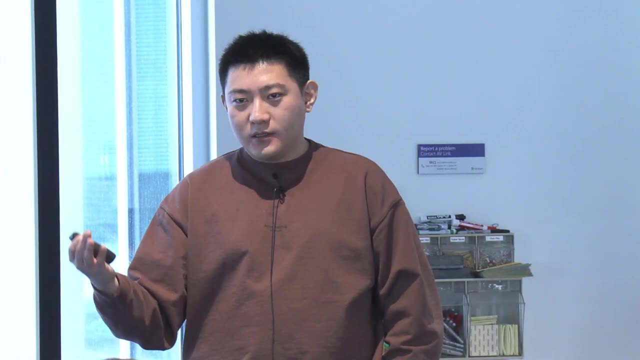 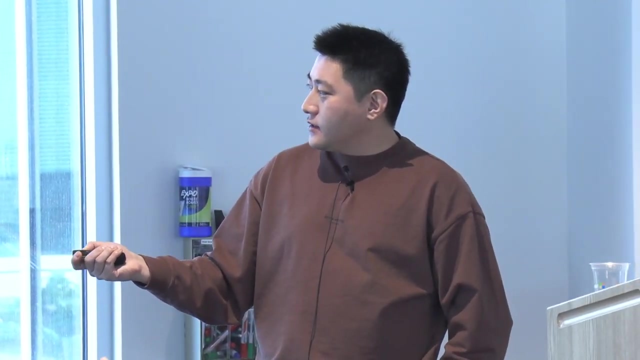 So let's say I give you a test to do like some evaluated algorithm using homomorphic encryption. or let's say I just give you some simple test like a polynomial. evaluate the polynomial. You can write it down with homomorphic encryption. and these all happens in evaluation. 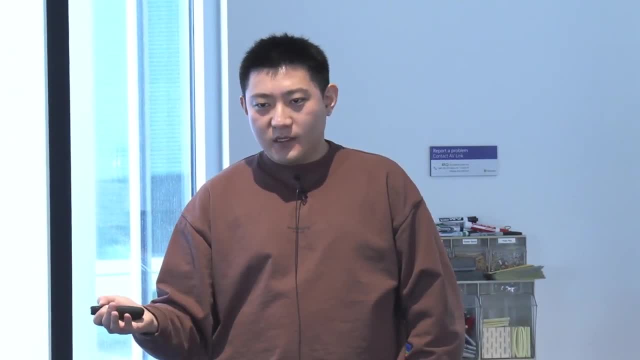 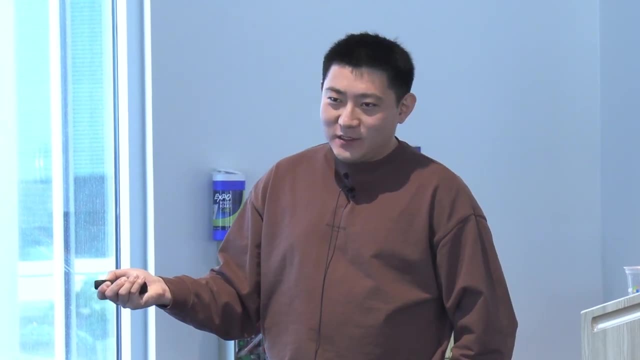 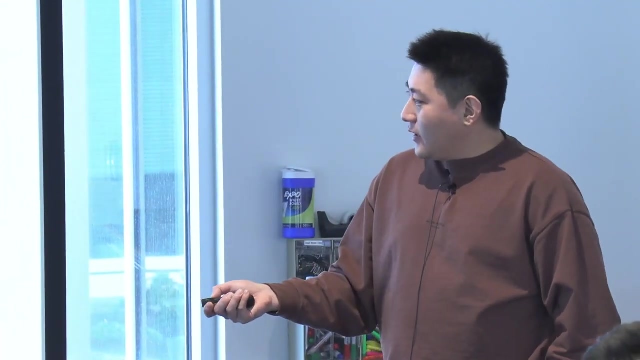 In other way to say, is just the computation on secure data, and this is what really matters. As you can see, it happens on the fourth stage, but we can get started here, because it's more intuitive to define your algorithm, how to write the code. 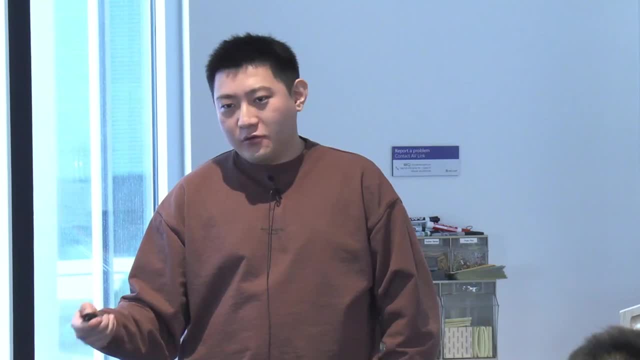 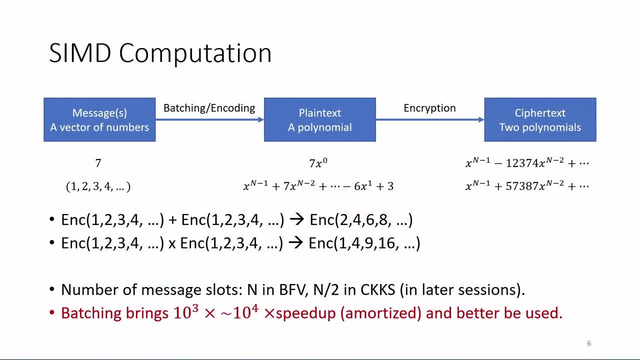 At last you decrypt your data. after computation is done, you decrypt the result, So let's get into the encryption. So I need to introduce this SIMD computation. A lot of you probably know SIMD. a lot of you don't. It's single instruction, multiple data. 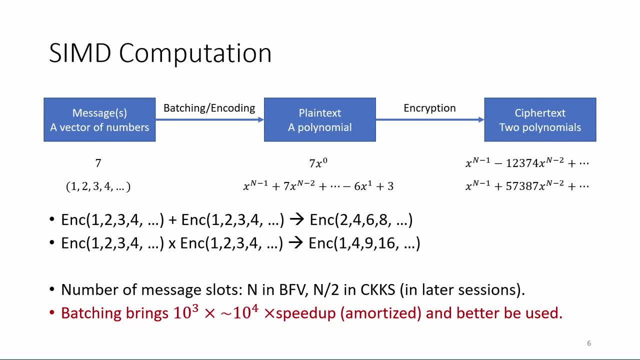 That means when you issue a single instruction or operation, it applies to all the data independently. So it's the cut: single instruction, multiple data. We use that in Home Open Encryption. Then you have a message. For example, the message is a vector of values. 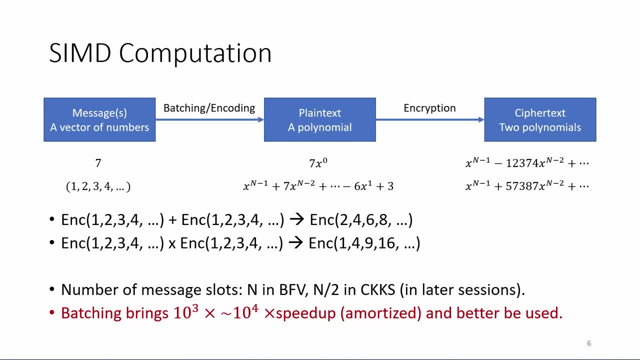 one, two, three, four, a lot of them. There's one encoding happening here that gives you a plaintext. Remember, the plaintext is a polynomial. For example, encoding of one, two, three, four can look like this: It's a polynomial, This is a plaintext. 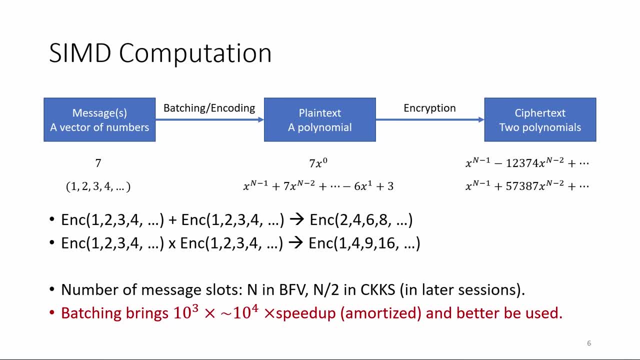 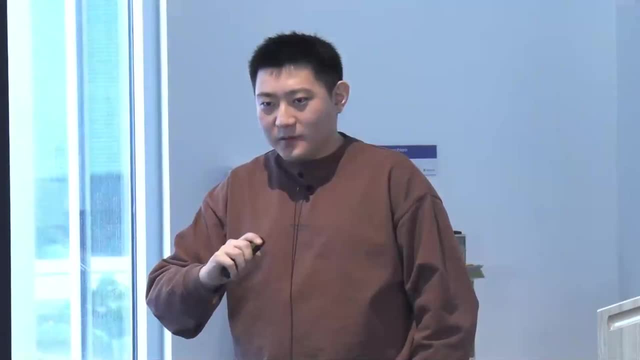 I need you to remember what is message, what is plaintext and what is ciphertext. Ciphertext is the output of the encryption. So here is what security really got guaranteed Before this encryption. everything are just plaintext, like in clear state. I give you the plaintext. 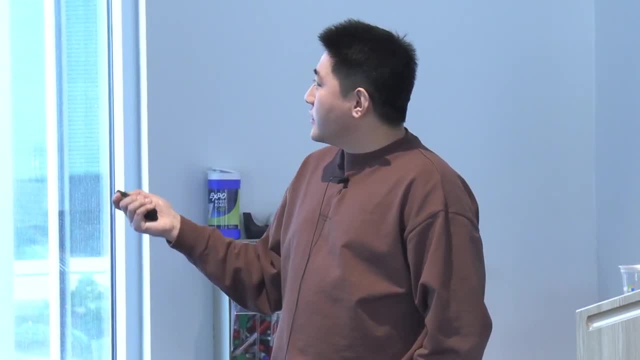 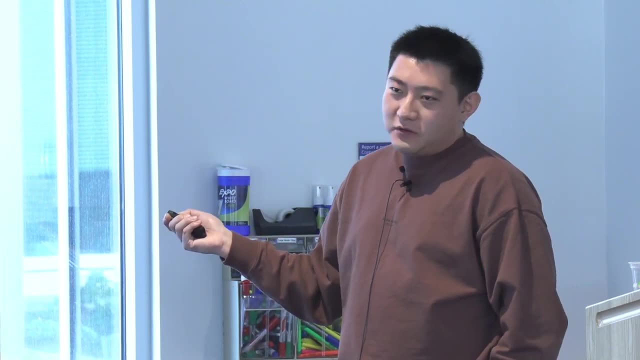 you know the decoding algorithm. you can get it, you don't need a key. But here is where security starts to matter and the ciphertext will have a random looking. It's totally meaningless. You don't see anything, You don't get any information from it. 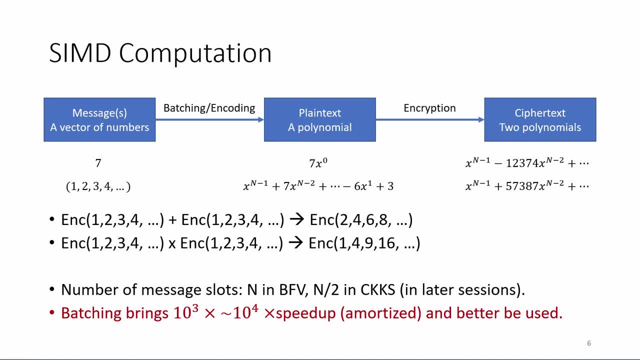 Suppose you are just encoding a single number. it's just become like constant polynomial. this is just seven and still the encryption give you a random looking polynomial. You cannot really distinguish whether you are encrypting one message or a lot of message. 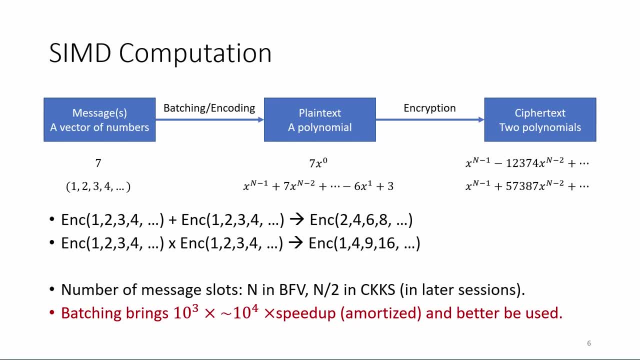 because the ciphertexts are always random looking, And how do we do the computation? So you have one, two, three, four encrypted. You have another one, two, three, four encrypted. I want to do an addition. The result will be the encryption of two, four, six, eight. 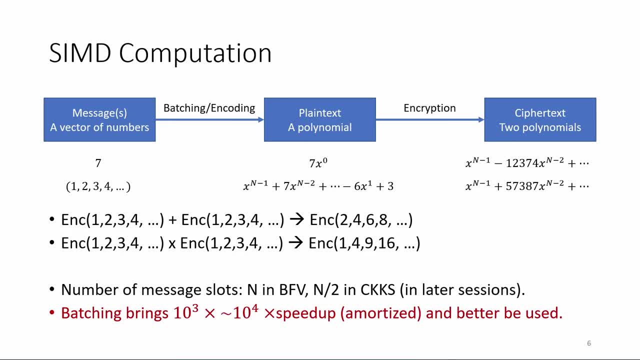 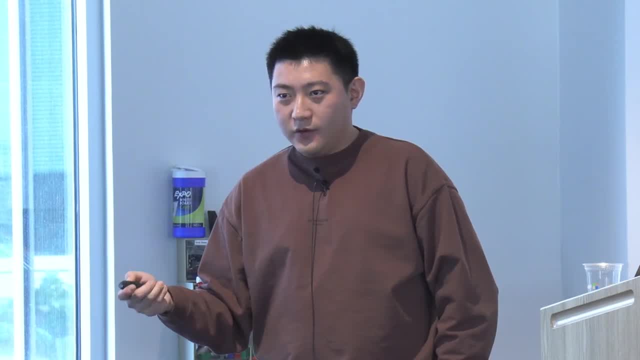 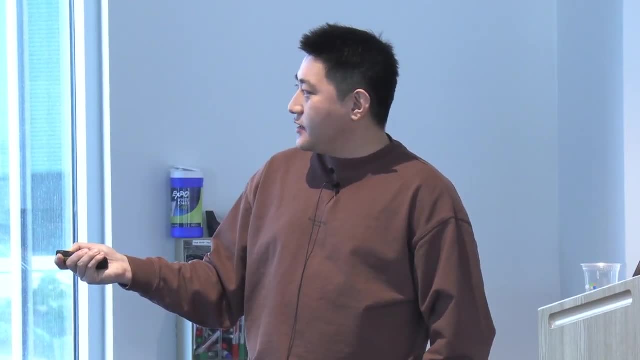 The addition is done coefficient-wise, element-wise Same. with multiplication it becomes one, four, nine, 16.. So we are clear on how the computation on vectors are done here. Homomorphic encryption just preserves these addition and multiplication. So you can see we are operating on ciphertext. 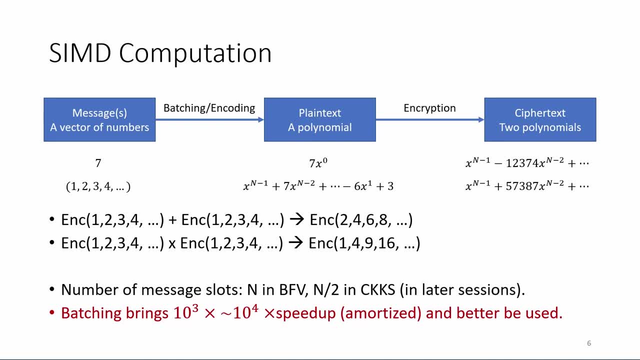 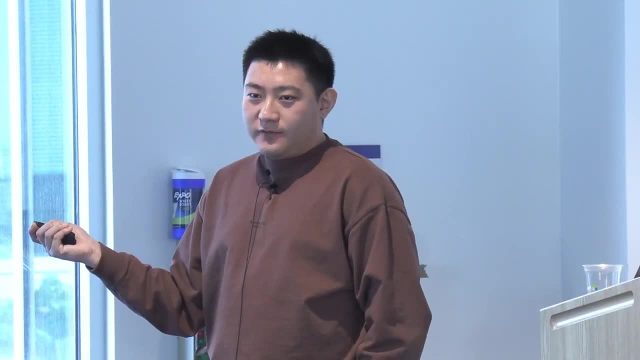 but the arithmetic it's done on a plaintext. We will get into more detail about what's the number of message slots. So a high-level idea. it is related to the degree of this polynomial: The higher degree you have, you have more message slots. When you are having more message slots, you have more parallelism and one operation here operates on thousands of messages slots. That gives you a 1,000 to 10,000 times speed up amortized timing. This is what matters in the last stage. 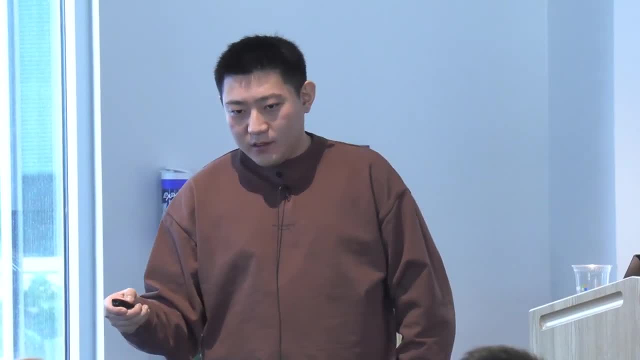 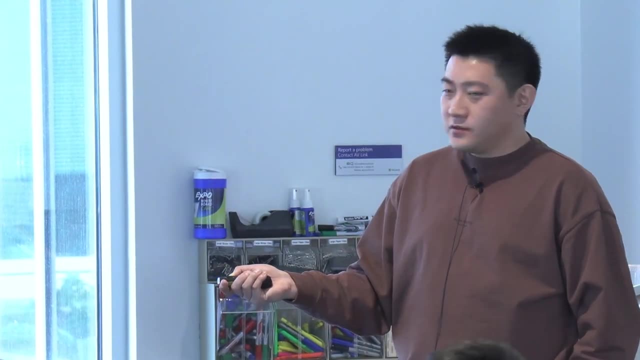 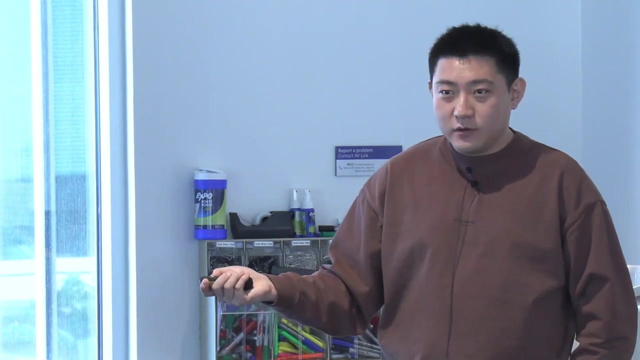 When I say the performance is 10 to the three to 10 to the six, that three orders of magnitude gap is introduced by these. You should always use these whenever possible, because otherwise you get a slow program and it's not efficient. So this is the first step. 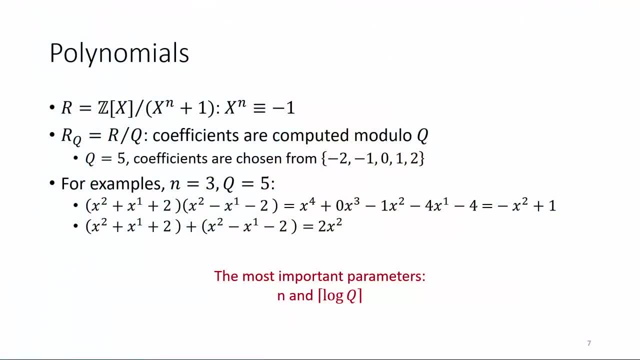 Next slide. So enough on the plaintext and message side, and let's talk about what are those polynomials. You need these in the following slides. We try our best to match the notations. So let's define what's the polynomial ring. 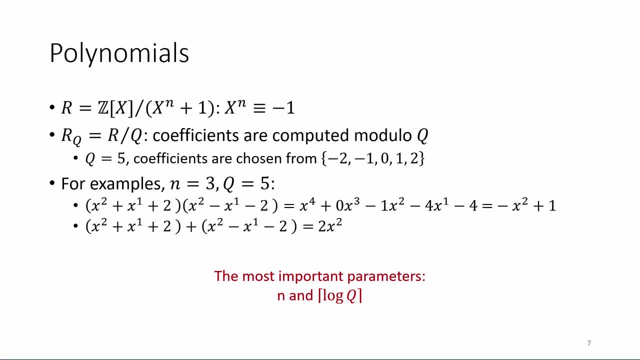 We use this ring in Home of Encryption. So it means a polynomial whose coefficients are chosen from the integers and the polynomials are computed: module x to n plus one. So it means: in this ring, in this r, all the polynomials have degree, at most n minus one. 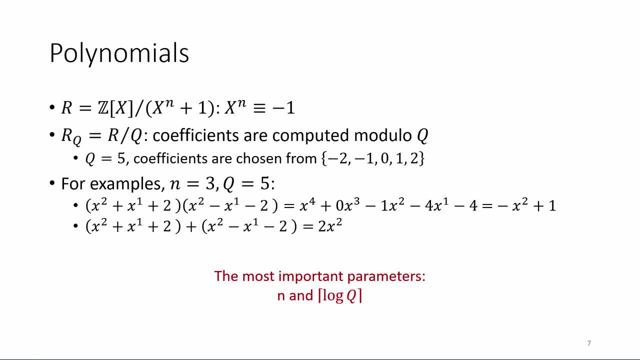 If you ever have a term which is x to n or x to n plus one or x to n plus two, it will be reduced. module x to n plus one, For example, module reduction x to n equals to minus one in this ring. 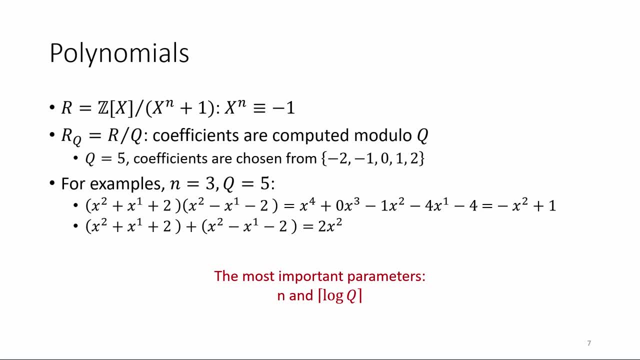 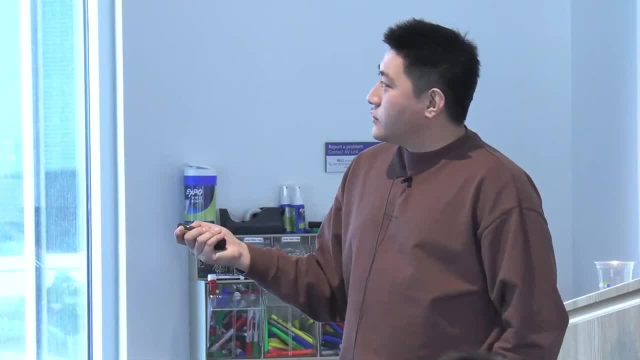 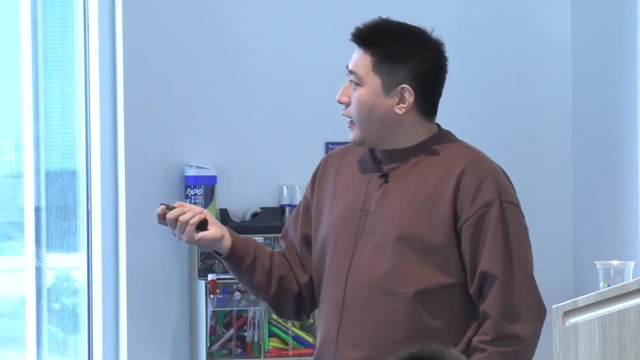 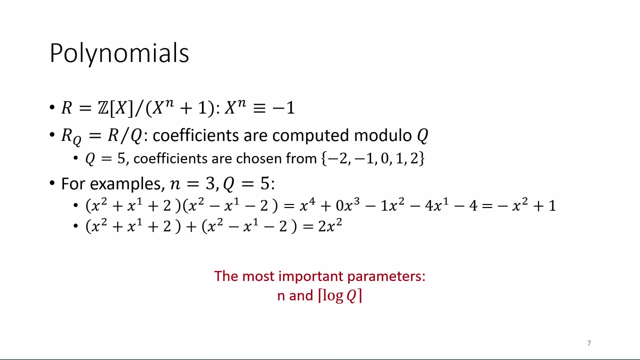 You just wrap around and flip the sign. So x to the n plus one is minus x. Well, x to the two n becomes one. So this is the basic polynomial arithmetic in the ring. Then further we have this quotient ring that the coefficients are now computed. module q: 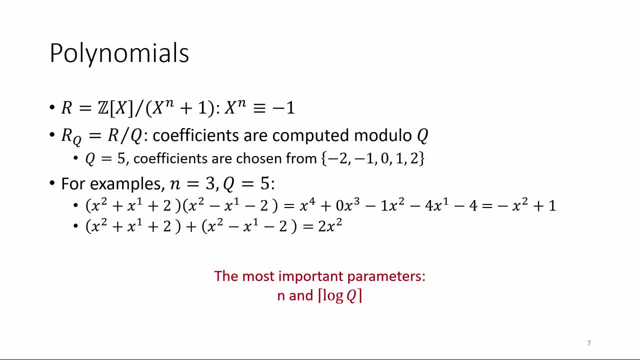 So your coefficients are no longer just an integer. They are represented with a set of integers. For example, let's say q equals to five. as an example, Coefficients can be chosen from these five numbers. They are zero balanced, which is good. 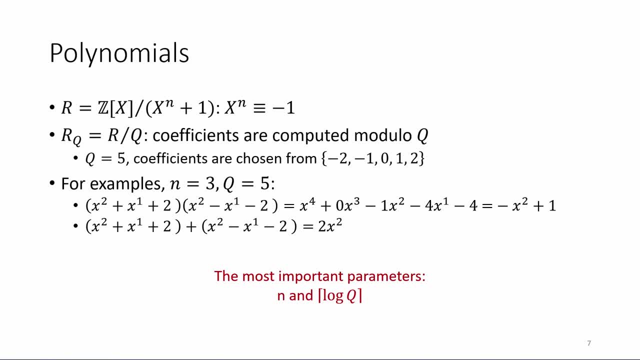 and the computation are done. module of five, For example. let's say you have two plus two, you get four. but four is not an element of this group in this set. So the image of four becomes here: It's minus one in this arithmetic. 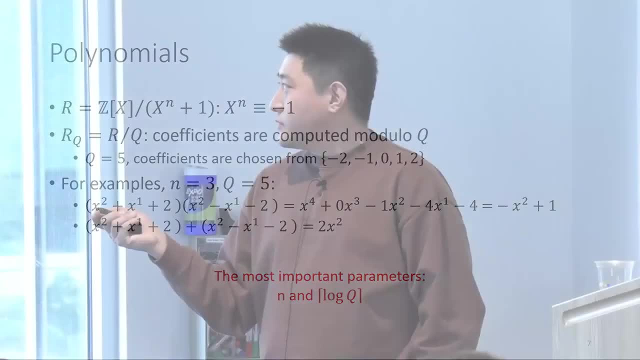 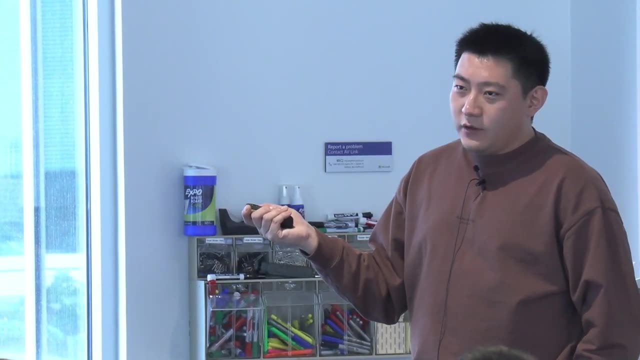 So everything is done. module of five. but you just mesh them into the correct element. You can also think these as from zero: one, two, three, four. You can use those five numbers too. just it's not zero balanced. It might be easier to understand. 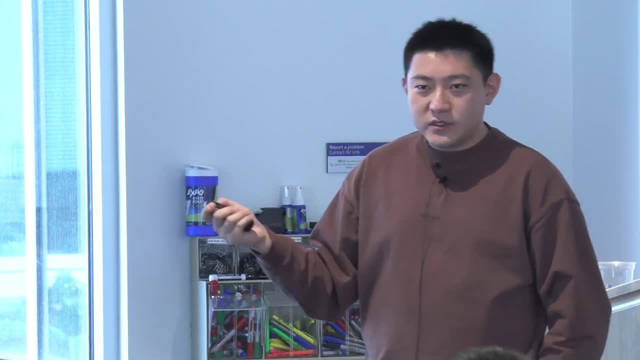 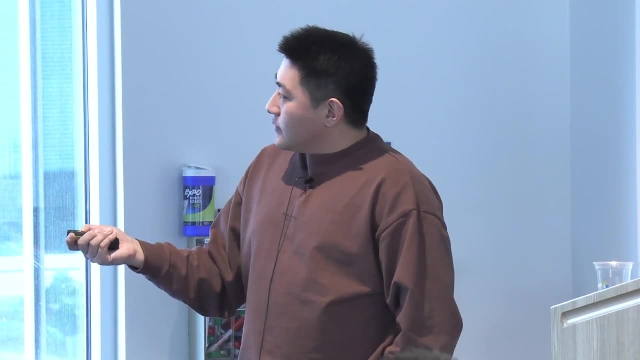 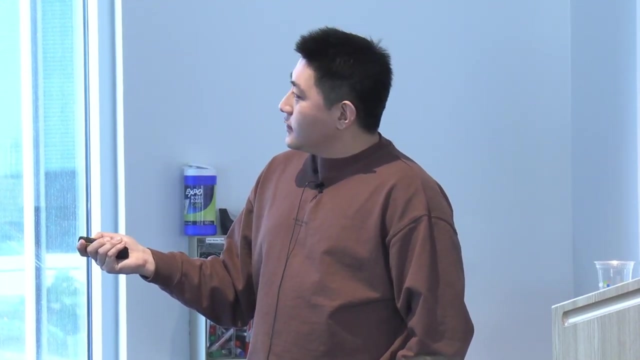 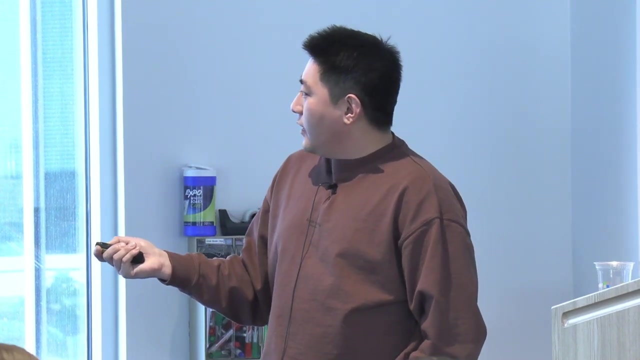 but it's not zero balanced, So we don't normally use that unless to do efficient programming like writing a code. So here is a short example on the polynomial arithmetic: modulo x to the n plus one and modulo q. So assume you have r five and a degree n equals to three. 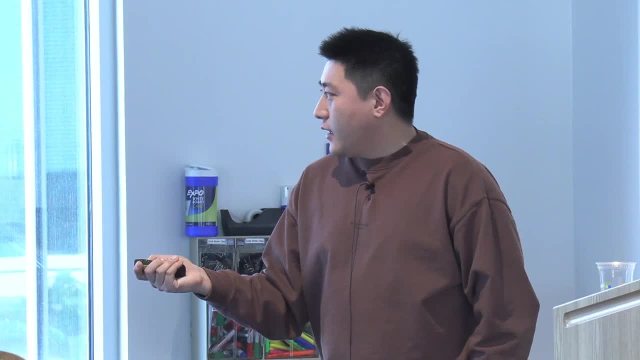 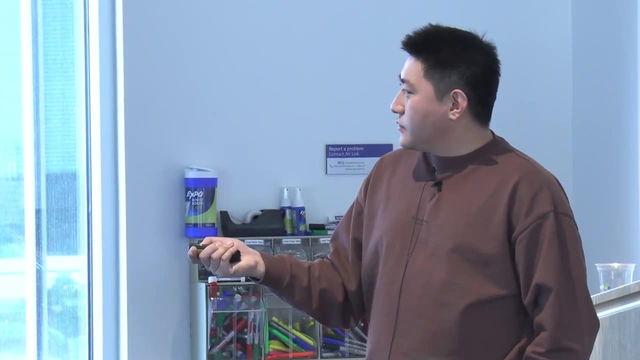 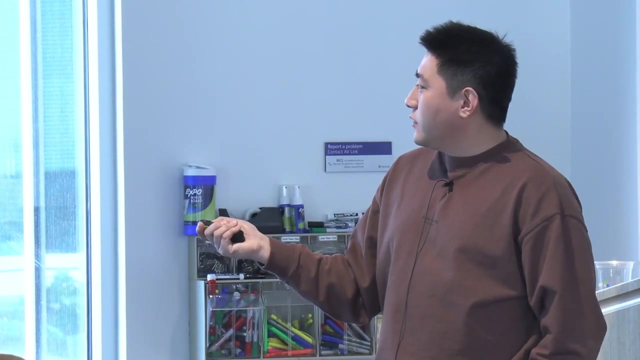 Here is the arithmetic. If, for those of you who haven't like getting to this part, you can try to calculate this thing Basically, you just multiply them term by term. you get this high-degree polynomial and you start doing a reduction. 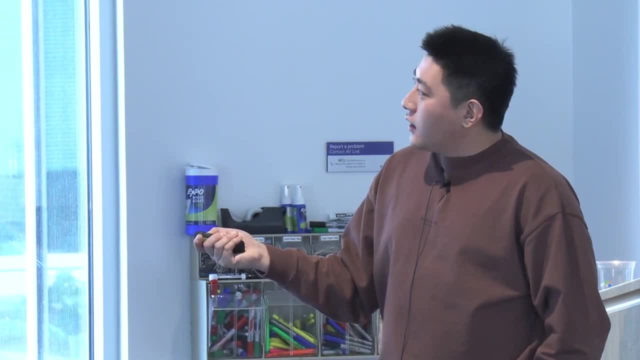 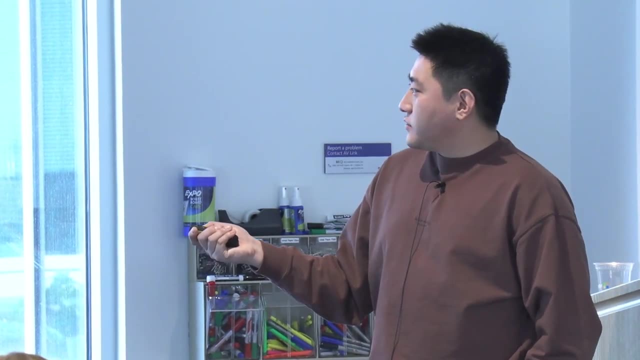 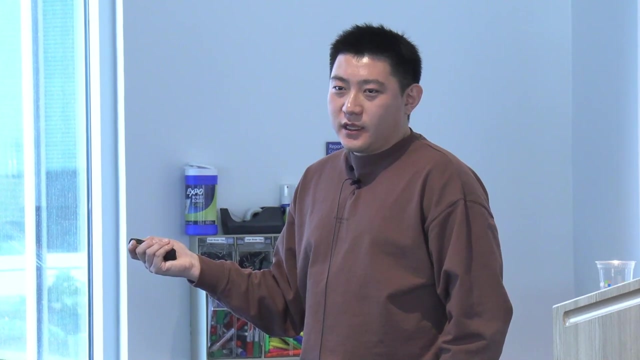 Let's say: x to the four goes to minus x, X to the three goes to minus one, but the coefficient is zero, so it's disappear. Eventually we'll get minus five, x, and modulo five gives you zero. The end result will be just minus x squared plus one. 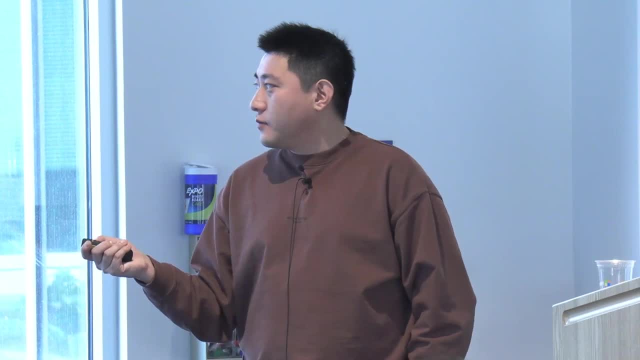 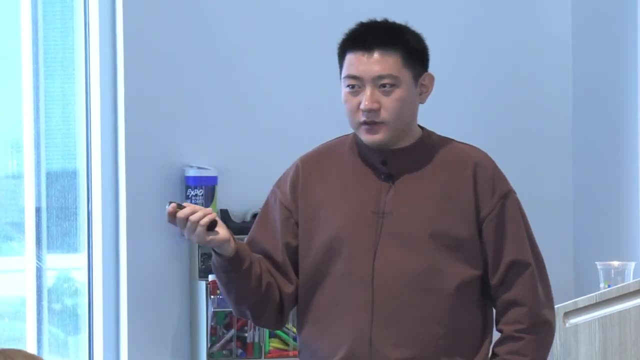 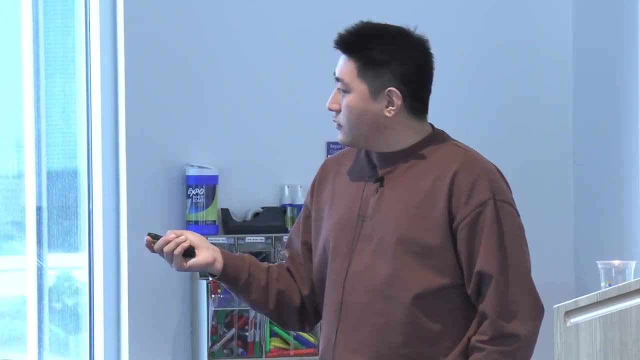 This is the basic way how to do polynomial multiplication and polynomial addition in RQ. We will see R and RQ a lot in the following discussion, like: if there's a multiplication, it follows these rules. If there's addition, it follows these rules. 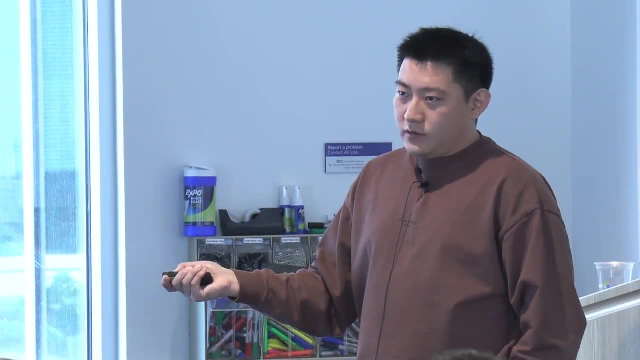 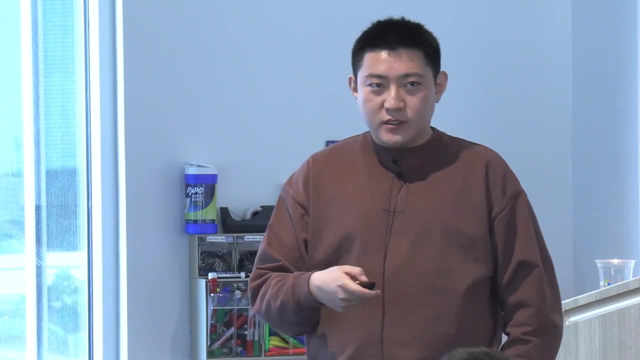 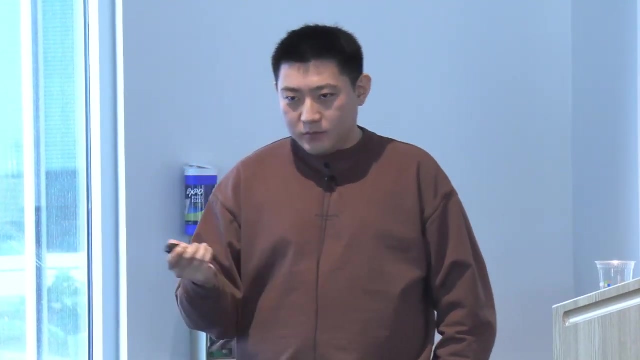 The most important parameters are n and log q. So the size of this q and the degree those two defines your security. As Christine has mentioned that almost all the efficient schemes based on the ring learning with error problem is mathematical problem and we try to parametrize the security level. 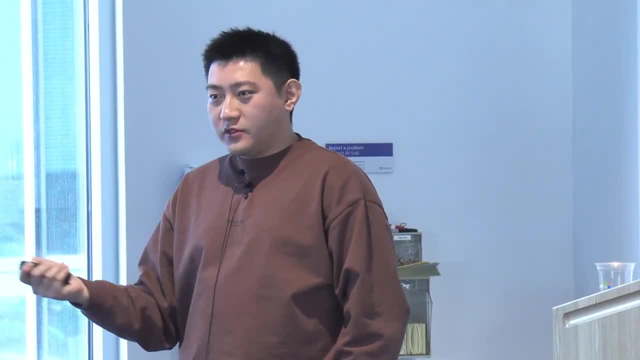 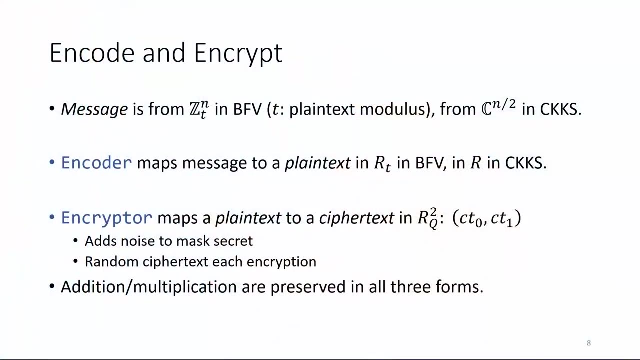 Let's say, for 128-bit security what parameters you should choose. By parameters we basically mean n and log q. So let's get into how the decoding and the encryption is done. First. I'm taking BFE as example, but just for you to understand how it works. 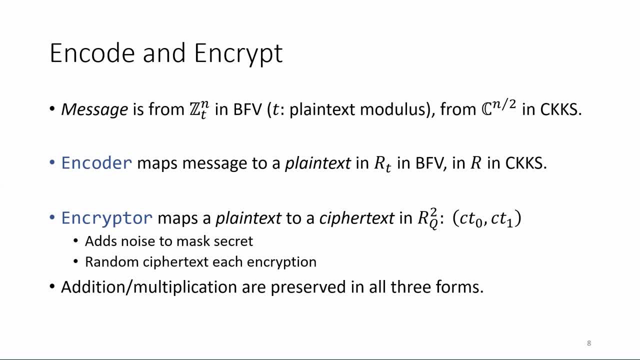 So your message can have a certain form. Your message can be chosen from complex numbers or it can be chosen from integers, modulo t- T is your plain text, modules, They say. normal computer works on integers modulo 2 to the 32, which is a single word size. 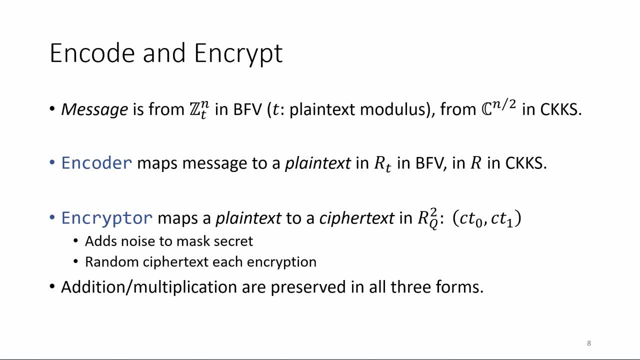 You can think this is just the plain text modules to the 32 or something else. It's a vector. it's always a vector for efficiency. What encoder does is it maps these message vector to a polynomial. If you are using BFE, which we have, messages modulo t. 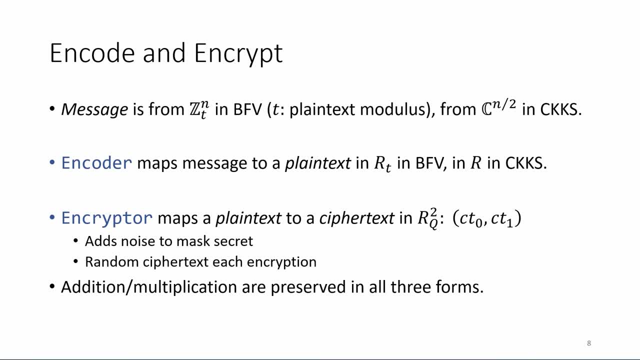 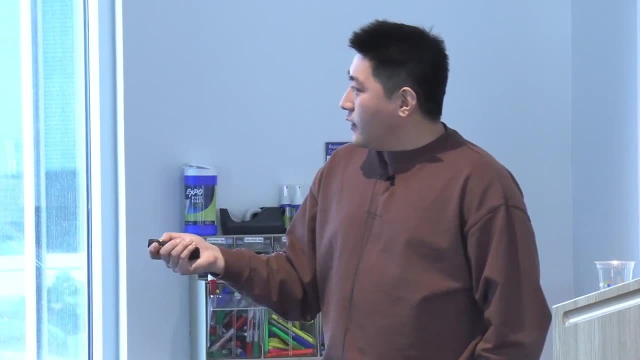 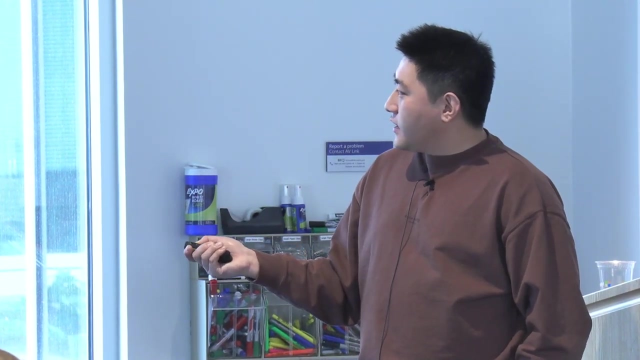 then your plain text will be modulo t as well. If you are using CKKS, you will have messages chosen from complex. you get just a polynomial in CKKS, Some they might have larger coefficients, And here the encryptor maps these plain text polynomial into a ciphertext. 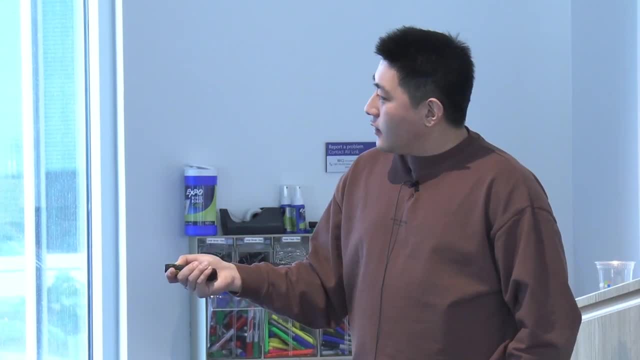 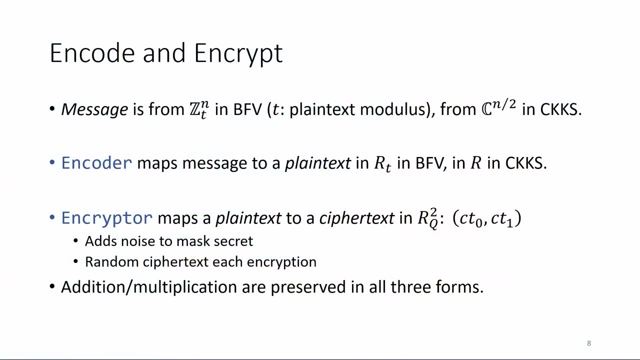 which is a pair of polynomials. What it does is actually adds noise to mask the secret, which is the message or plain text, And then it randomized this ciphertext after each encryption, So that encryption of the same plain text give you different ciphertext always. 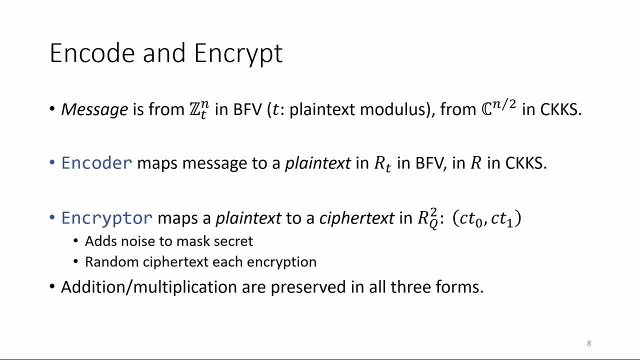 Otherwise you, just you can read the message anyway. So this is how to make it secure. And addition multiplication: these two operations are preserved in all three forms: Message, plain text or ciphertext. You can do addition multiplication on all three of them. 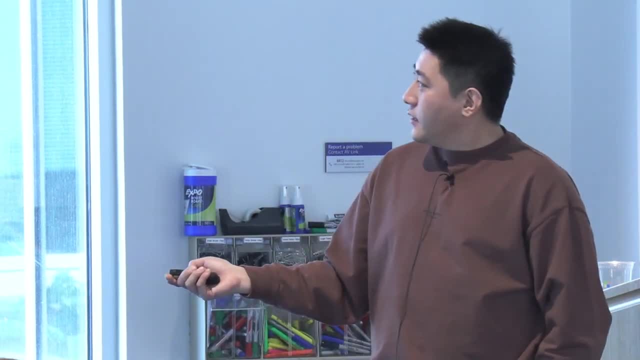 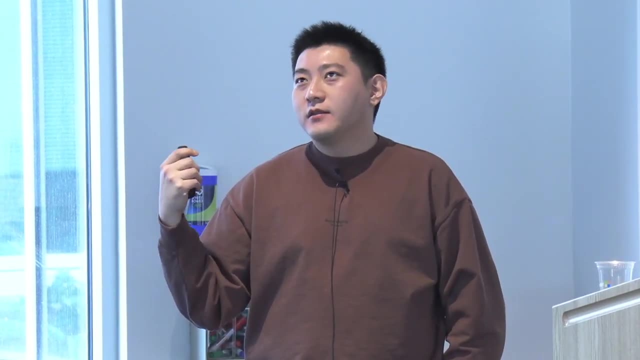 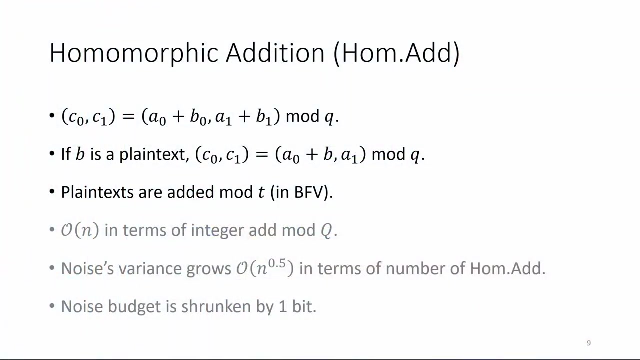 They always preserve your computation. This is what Christine mentioned by the computation commutes with encryption, And what operations we can use in homomorphic encryption? The basic one is addition. So addition is simple, Since you have two ciphertexts, A and B. 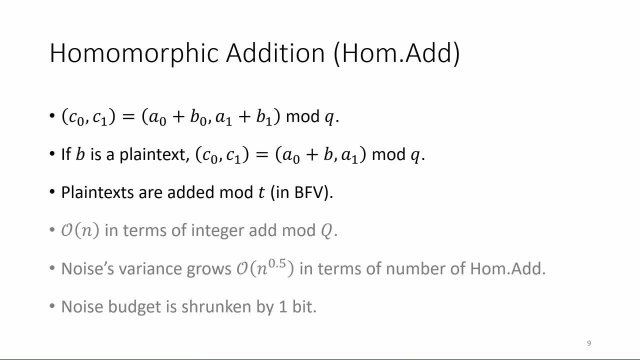 you just add each polynomial together. Let's say you add A0 with B0, add A1 with B1, you get the result C0 and C1. This is your addition result. This is how the polynomial works, So homomorphic addition is done. 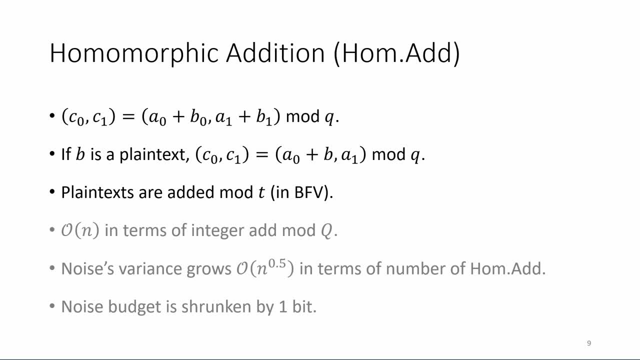 And if you decrypt this message, if you decrypt these ciphertexts and decode it, the message is the addition of A and B. So it's quite simple for addition And in a case when B is a plain text, you just add B to the first part. 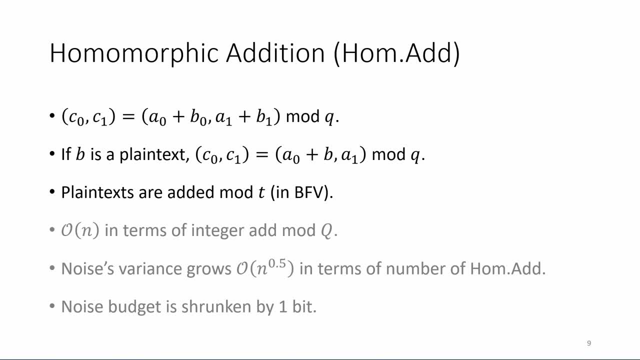 which is even faster, just half of the complexity computation. These actually have code examples in SEAL. Kim will explain that later. I think you can see from the code that we have multiply and multiply with plain those functions in SEAL. that very understandable. 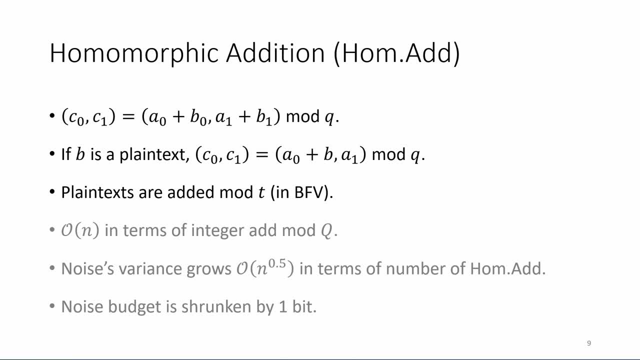 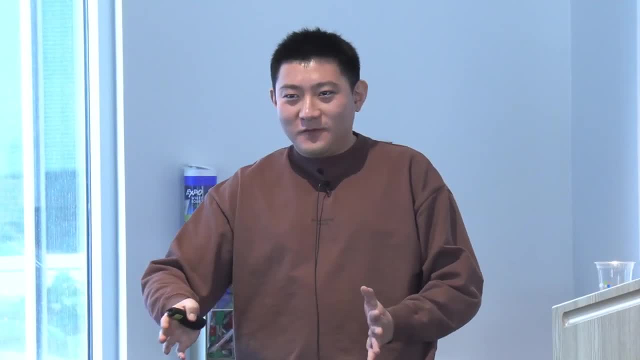 And plain text are computed modulo T. if you're in BFE, I just want you to know that these plain text operations are not what you define. You add 1,000 with 2,000, you might not get 3,000.. 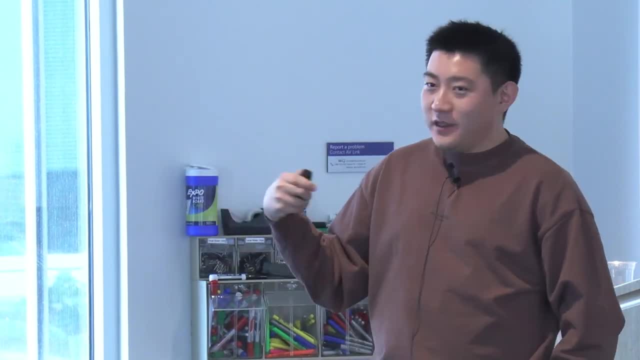 It's defined over this modulo T, or defined in this way. It's defined over this modulo T, or defined in this way. It's defined over this modulo T, or defined in this way, Or defined in the serial case. how much precision you want to preserve? 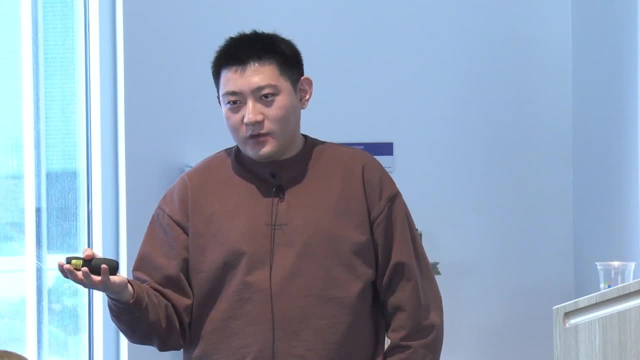 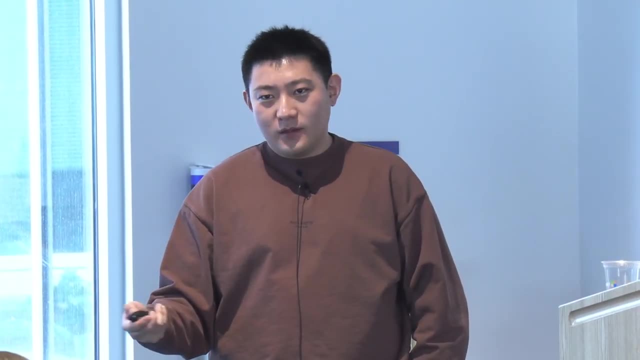 For example, if you are doing modulo 1,001 production reduction, if your T is 1,001, you add 1,000 with another 1,000, you get what you get: 999, something like that. 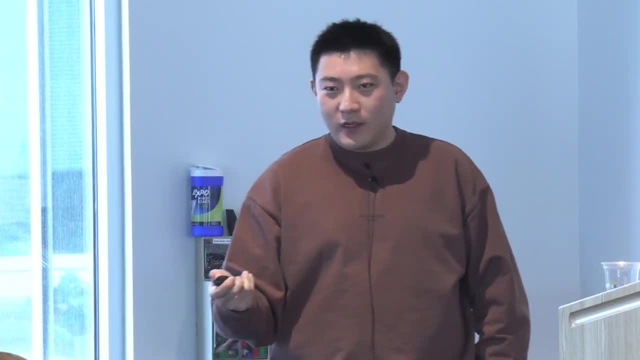 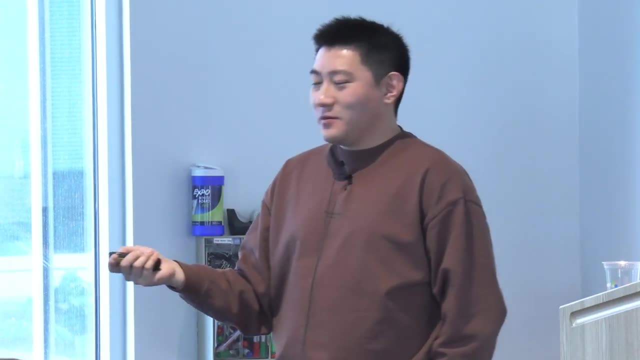 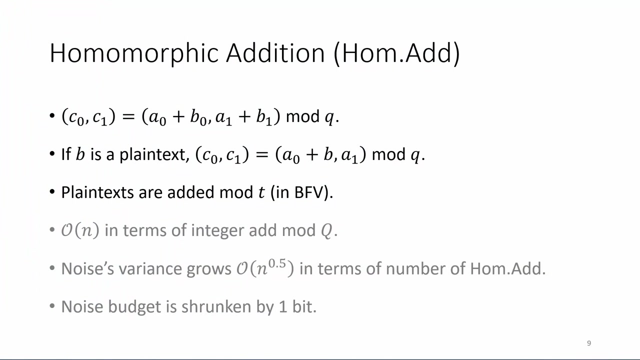 you get what you get: 999,, something like that. So remember that there's mathematics, not just plain addition, it's modulo addition and modulo multiplication. These great idea and readout stuff are just for future reference, if you want to refer back to these slides. 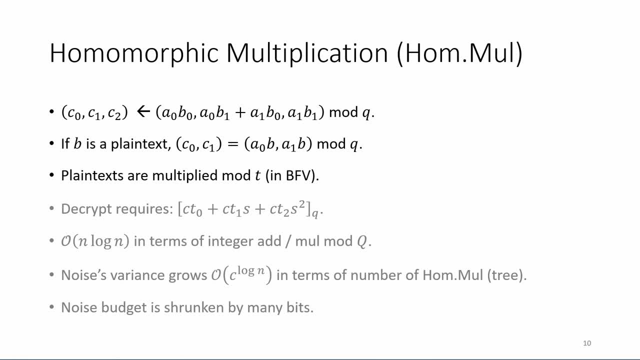 They explain the cost of these operations in terms of polynomial degree, those things. Here we also have homomorphic multiplication. It's a little bit more complicated. Multiplication actually give you three polynomials. as a result, You can see all A0 and B0 are used in this computation. 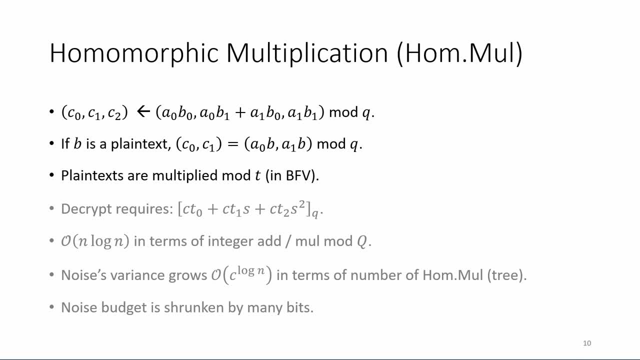 You compute the three parts and this is your result. This is ciphertext- times ciphertext. If B is a plaintext, it's much easier. Just multiply B to both parts. that is done. You still have a two-part ciphertext. However, this becomes a problem when you have three polynomials in ciphertext. 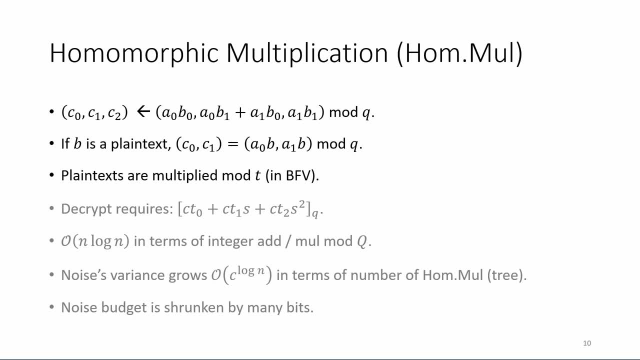 If you want to do another multiplication, what do you do? There will be a lot more computation and end up with more polynomials in the new ciphertext. We don't want to do that. We want it to grow because when your ciphertext get larger, at the end 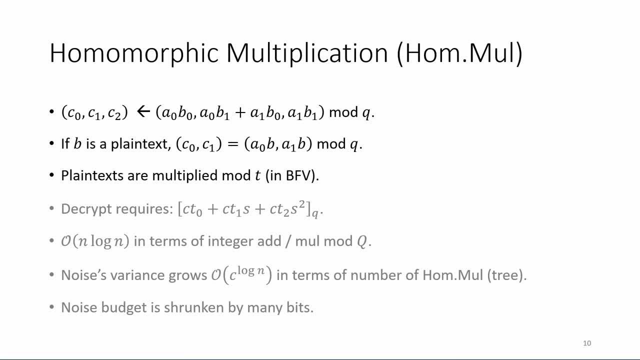 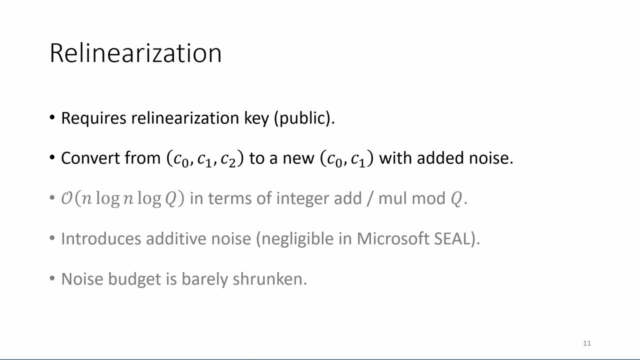 you get a huge result as the return result. You don't want that, So there's a step called linearization follow-up. This also have a function in seal. You need to call it. What it does is very simple: It just convert these three polynomial ciphertext to a new ciphertext with just two polynomials. 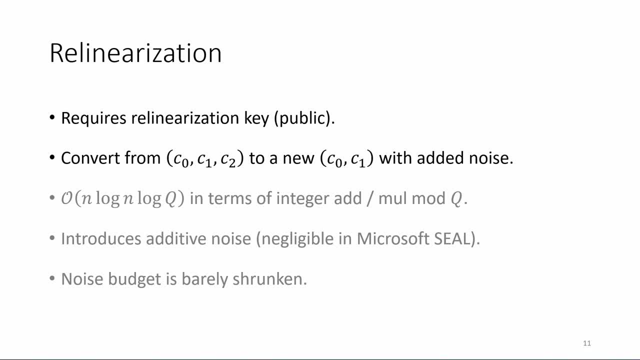 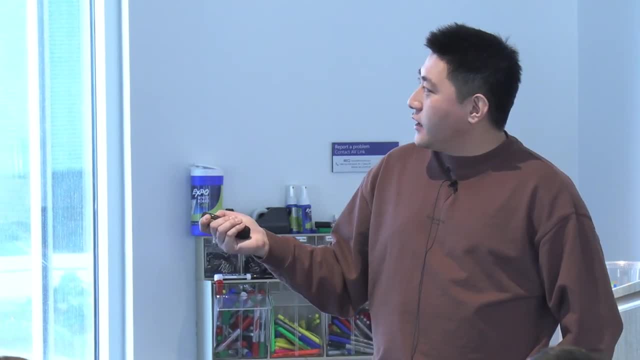 It's just a tool to convert it. You can think of it this way. It's very simple: You just call it, It converts it back to the two polynomial shape And it requires a linearization key. And this is just a public key. 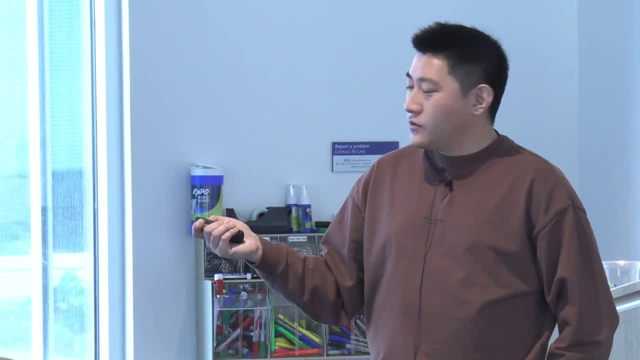 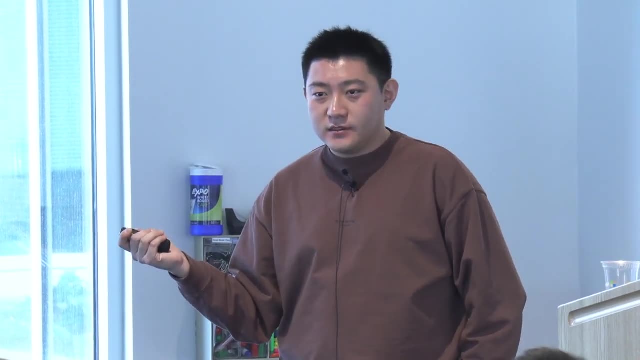 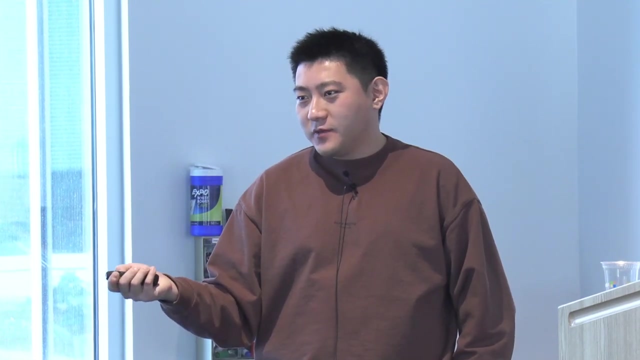 If this is done during key generation, you can send it to anyone. Anyone doing the homomorphic multiplication can have this key And we will need this key to reduce the ciphertext. So so far we have three steps, three functions, And actually those are five functions because it also involves ciphertext, plaintext multiplication. 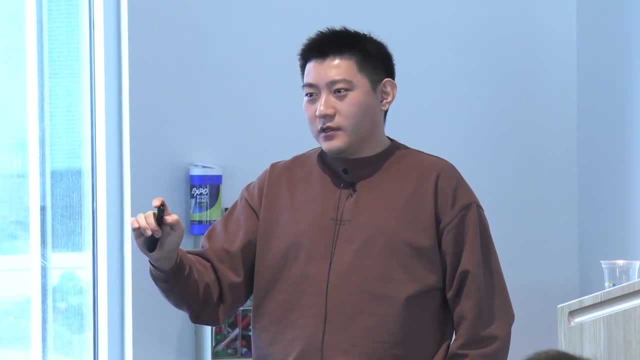 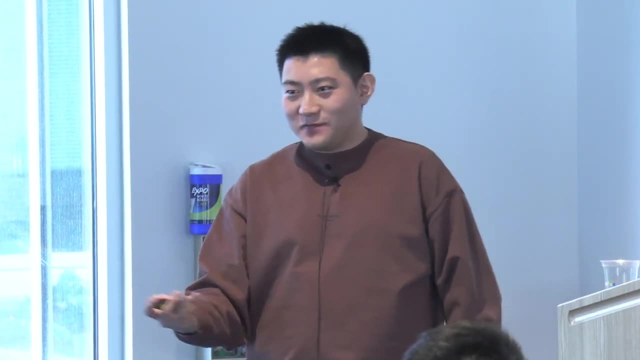 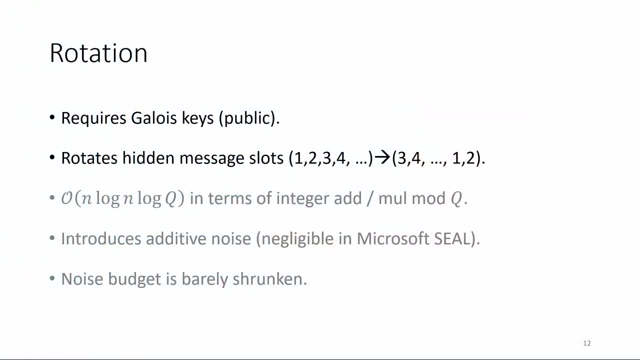 So these five functions should be enough for you to build a, let's say, polynomial evaluation or some basic algorithm, And in fact most of the schemes are just built based on those five operations. We actually have one more, Since we are encoding a vector of numbers. you might want to rotate the slots of those. 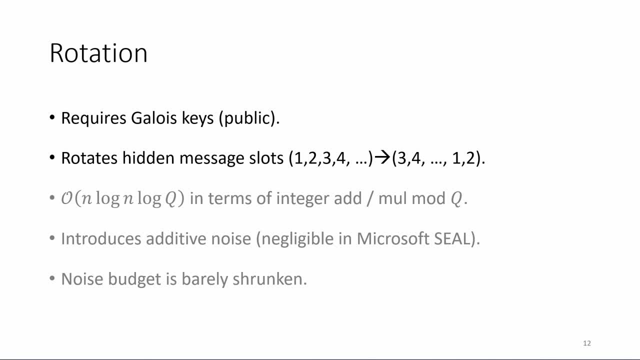 numbers. Let's say I give you one, two, three, four, But you also want to have two, three, four, one or some other kind of rotation. There's a five-function. Okay, So this is a faster way to do rotation on encrypted data. 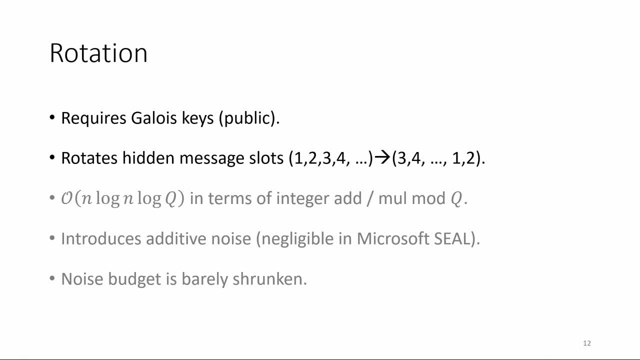 In CO you can find functions like rotate, rotate column, rotate matrix. those functions rotate vector And what it does is just change the order of these slots And it requires something called the Galois key. It's also a public key. 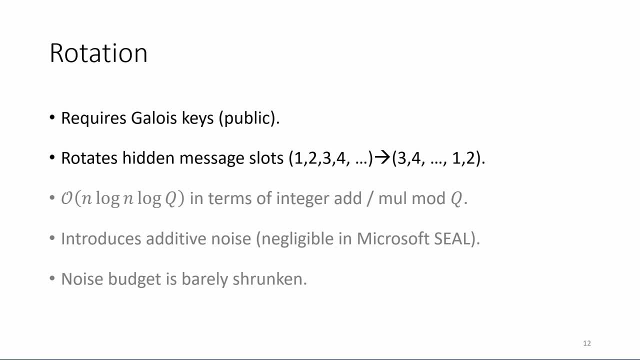 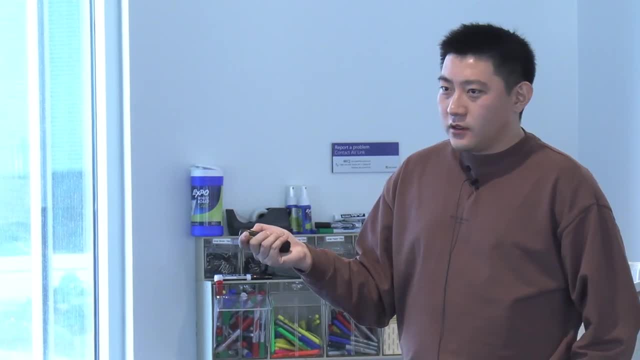 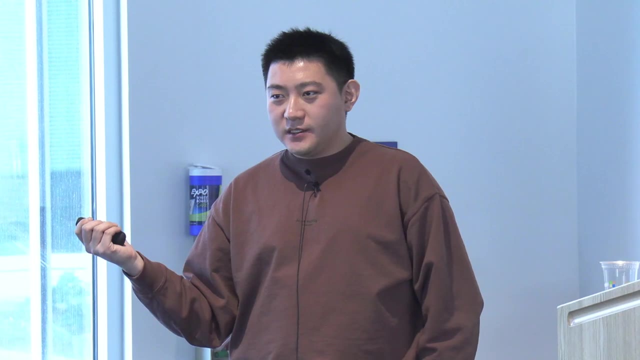 It's like a regularization key. It's just required for the computation to be done. You can have it. No security vulnerability And, as Arun mentioned in his talk, this key can be a little bit large And you might want to consider the storage of this device. 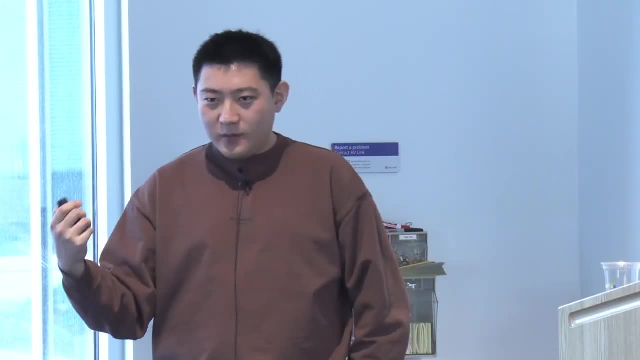 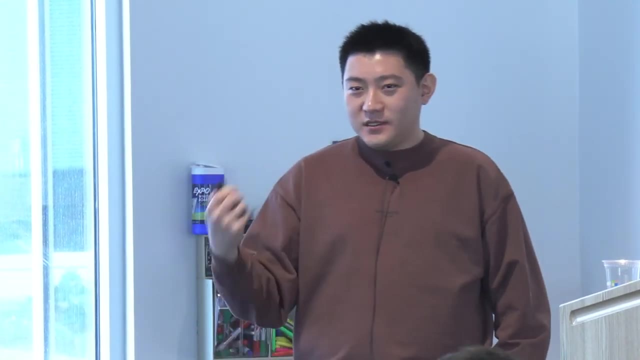 That was a very interesting talk. when people don't usually think about 50 megabytes public key is a problem in a home of encryption work because we start with gigabytes of public key. Now it's just 50 megabytes. It's super tiny. 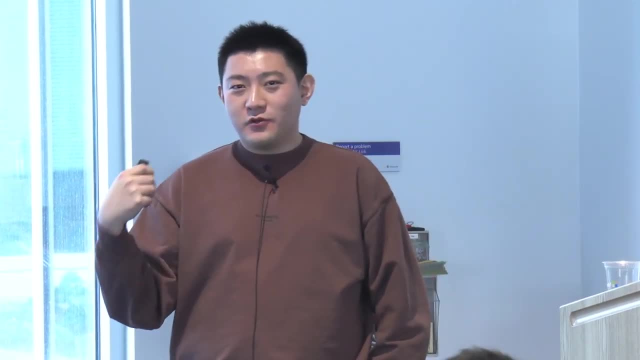 But in fact when you are doing like a multi-key operation, it's just 50 megabytes. It's super tiny. So if you're doing a like event, for example in your computation, you need to think about. 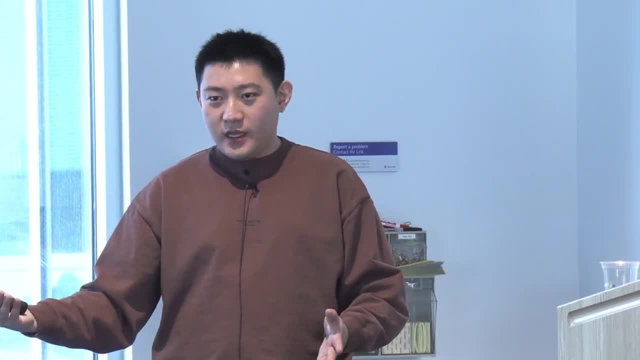 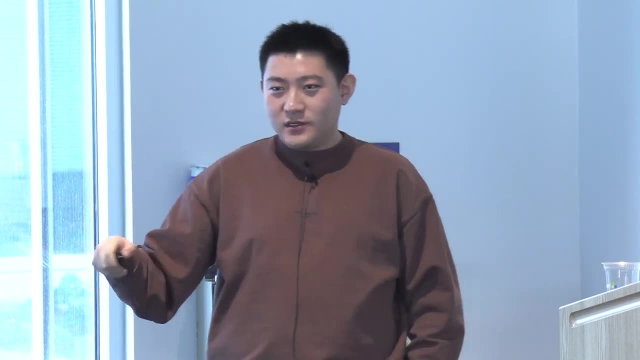 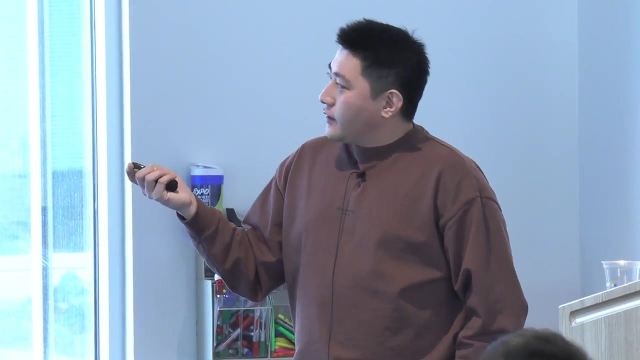 real-life example. You want to think about the user's case. Let's say someone has a computer offshore. You need to send a lot of data to it. You need to consider data size, And this is something to consider. Like this key can be large. 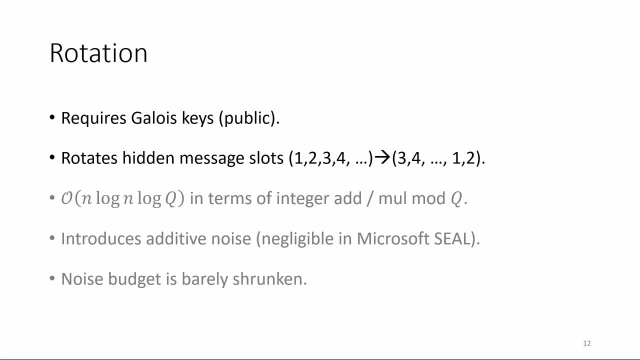 And now you also have rotation, Kind of we have the complete set of operations we have. If you're thinking about computer arithmetic, you can think that We first define addition, multiplication and bit shifting. So based on those three you actually have the modern computer. 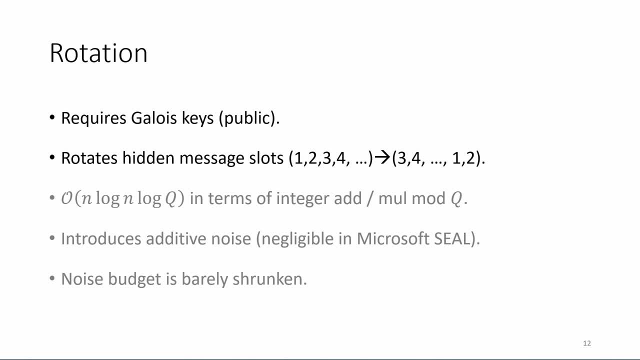 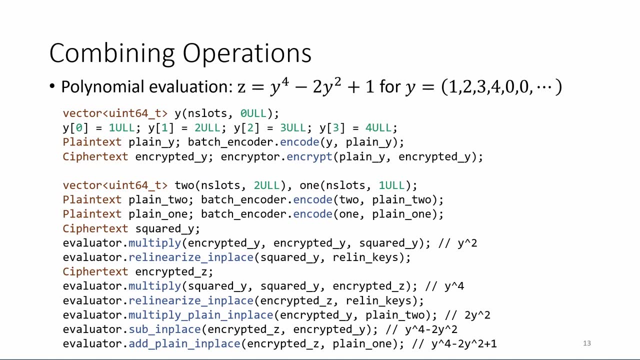 And here, same These operations, we can build very complex algorithm. Let's combine some of them and run it to code. So suppose I want to evaluate Y to the 4 minus 2Y squared plus 1 for this sequence, for this: 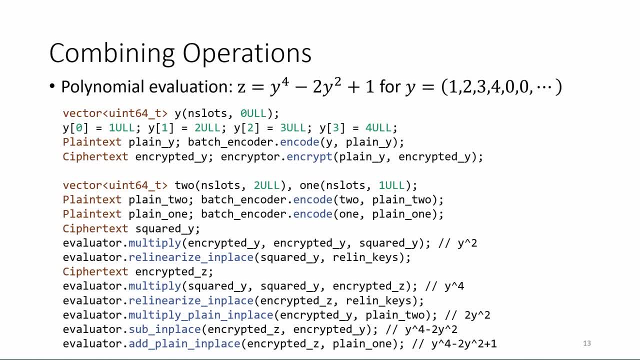 vector of values. What you do is spin. First you create a slot of n slots of zero, filled with zero, and put one, two, three, four at beginning, so we have y. Then you just encode y to a plaintext. 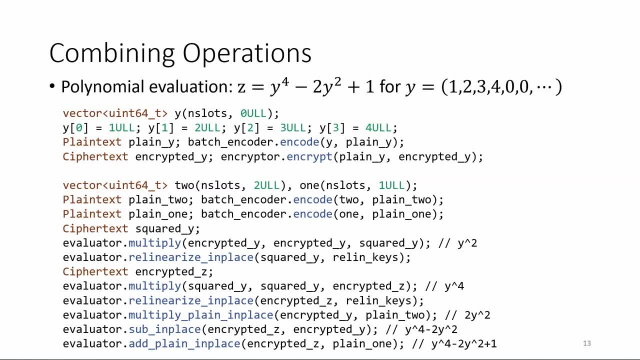 encrypt plaintext y to encrypted y, and that's done with encryption And the following. let's say I have a tool, a vector of all twos, we have a vector of all ones to you know, just to mark these two constant terms. 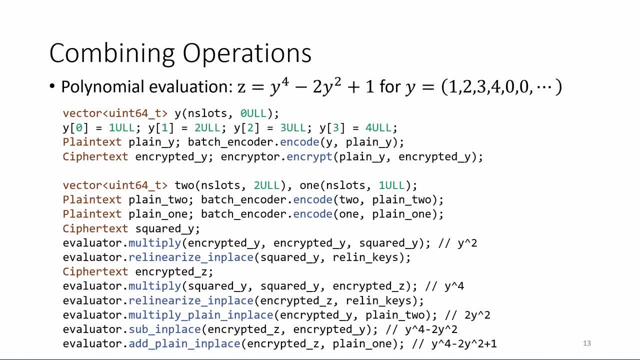 They can be encoded to plaintext two and plaintext one, so they become polynomials and they can compute with the separate x, y. Let's start with computation First. you have squared y. you call this multiply to himself. so multiply y and y becomes y squared. 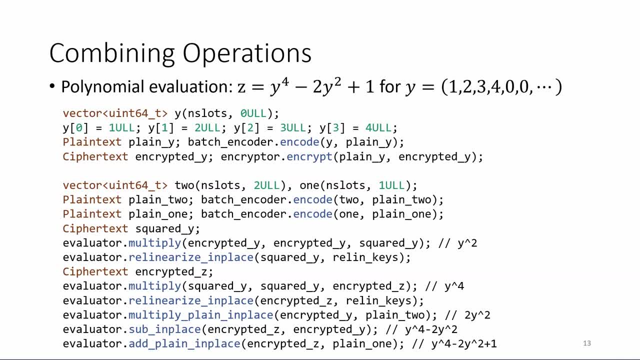 And the realization is required because you want to reduce it from three polynomials to two polynomials. And then I want to multiply y squared with y squared, so I get y to the fourth and also reduce the polynomial to only two And you multiply, plaintext. 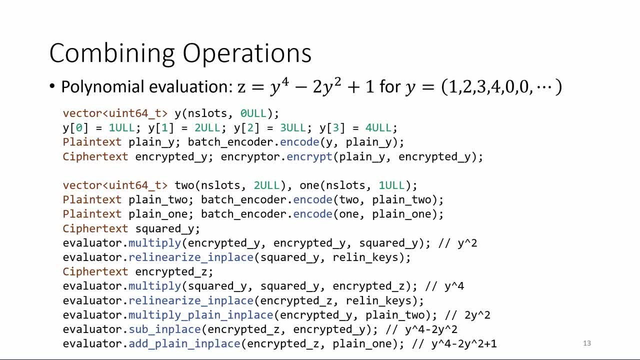 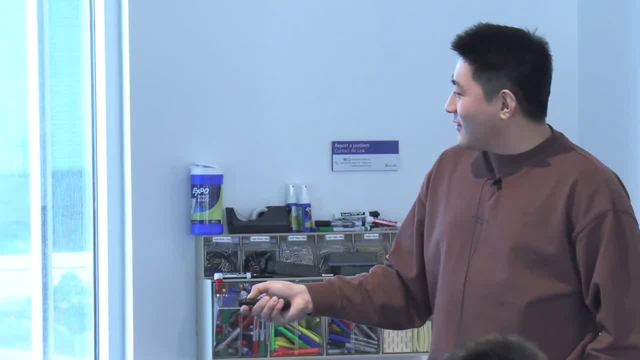 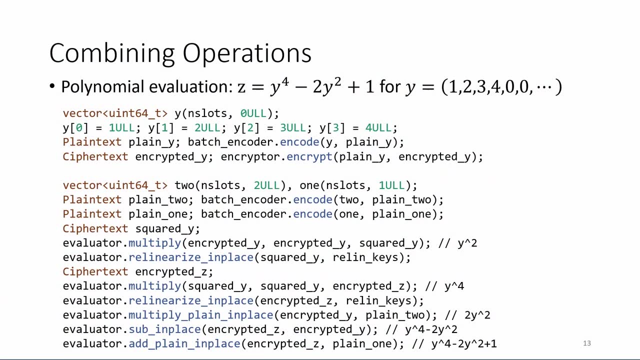 So this is encrypted. y is now y squared. Oh sorry, this should be y squared. Oh yeah, that requires some debugging, So I didn't write this code, So this should be y squared. You multiply with plain two. you should get two y square. 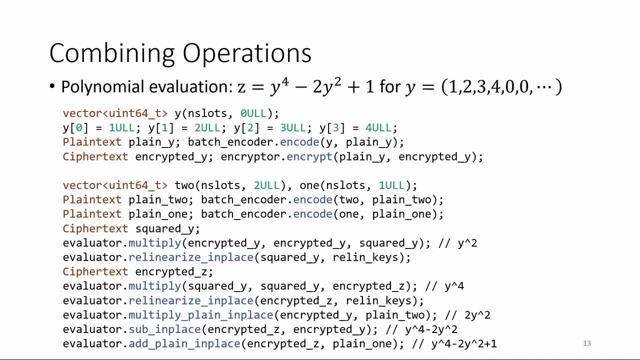 Let's say the result is stored here and you can subtract it from y to the fourth. So here it subtracted this value from encrypted Z. So in Z now you have y to the four minus two y square, and then you further add one to it. 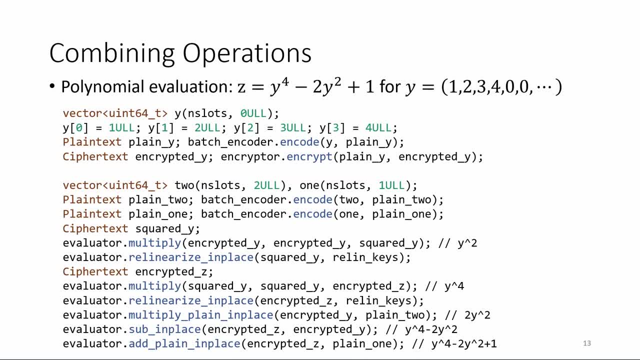 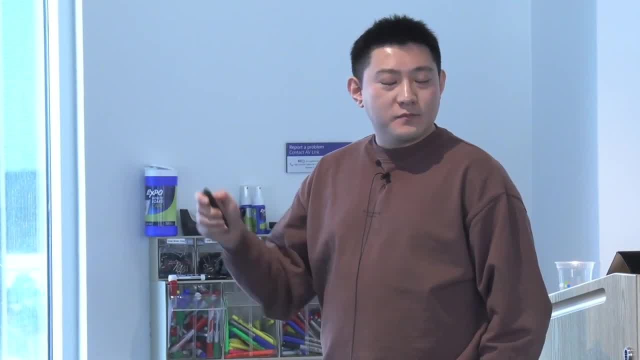 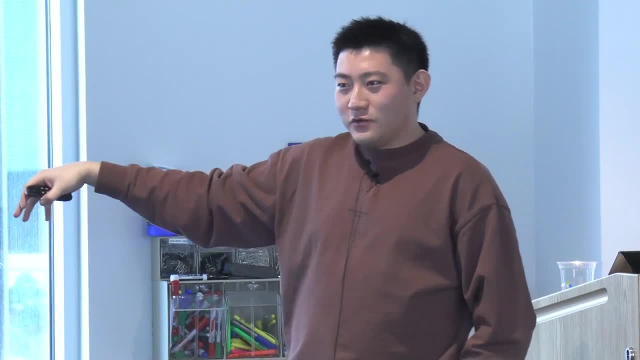 so you get the final result: Sure Question: Yeah, Later. I'll explain it later. So I'm trying to get around parameter selection, because to write down this code you don't need a parameter selection, So you can just write down the code, It's nothing. 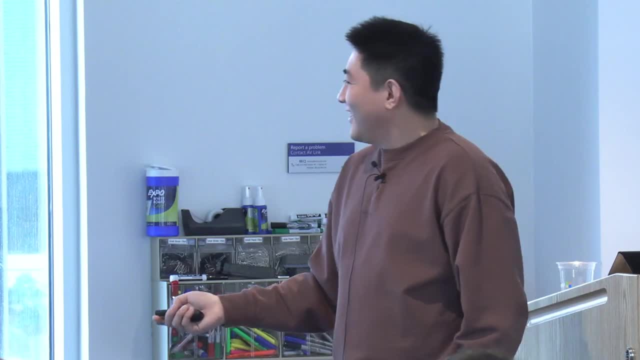 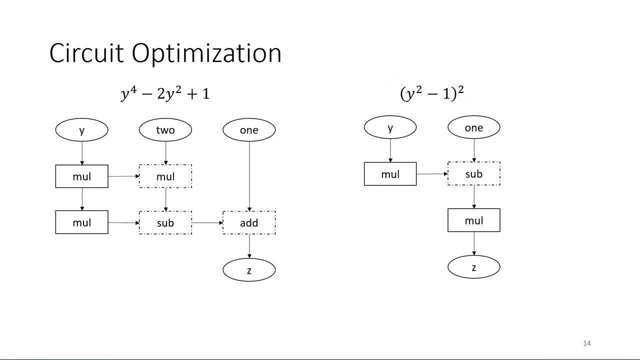 For me. I didn't even run the code. You caught me, So actually there's a better way to do this computation. You require some circuit optimization to get a better algorithm. So both sides achieve the same thing: computation. However, the right-hand side is much simpler. 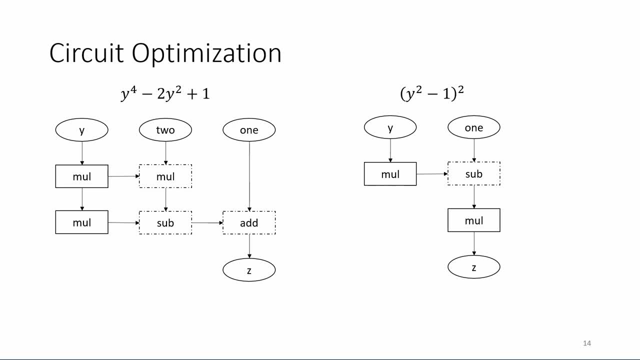 You see you have two less operations. We need to explain the definition of circuit here, So give you a polynomial or some function. There are many algorithms to achieve that functionality and one of the algorithm might have the minimal depths. By depths I mean the layer. 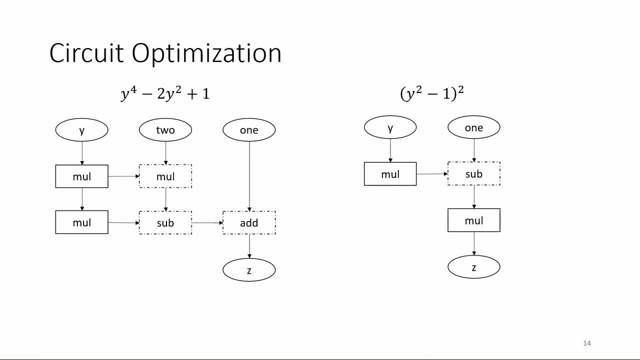 the layer of multiplications, ciphertext multiplications. So these solid box means ciphertext, ciphertext multiplication. This is just ciphertext, plaintext multiplication, which we don't care that much. This ciphertext, ciphertext multiplication is very important. We always want to minimize the maximum path of these multiple multiplications. 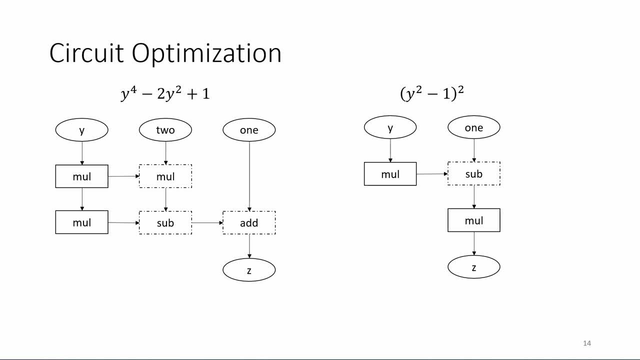 For example, in this graph, this is the depths two circuit. This is the first level, This is the second level. So you will hear the level, the depths and circuit a lot. I don't want you to get confused. 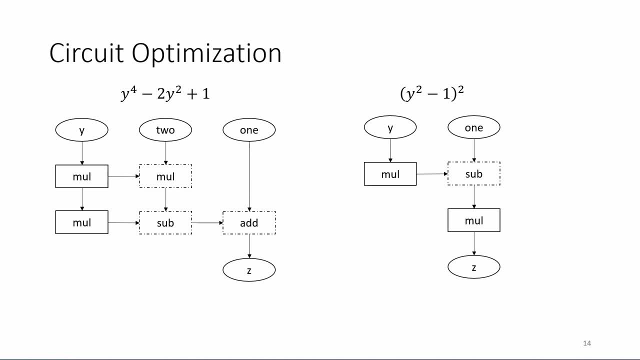 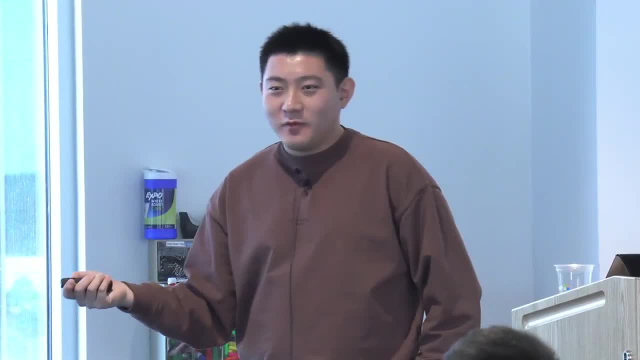 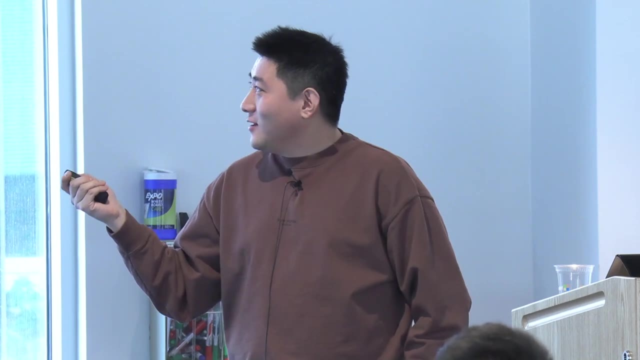 This is also a depth two circuit, but it's simpler because you have less computation. This is some optimization that usually cannot be done by a compiler. You are responsible to write better code using these, because this requires polynomial factorization. you need Wolfram. 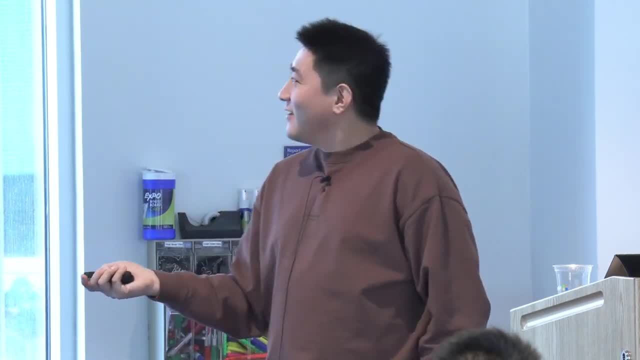 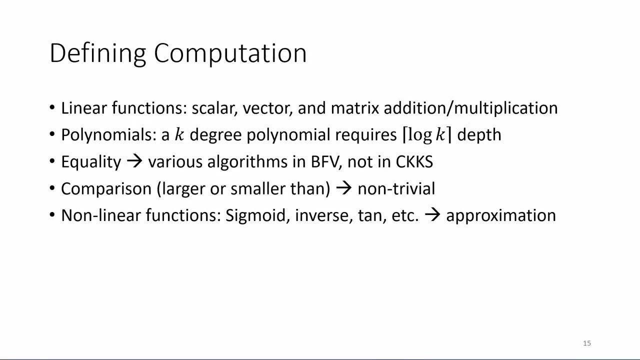 Alpha, which is not part of any compiler. So far you know how to write a simple code. What else we can do for computation? We can have linear functions, scalar, vector matrix, addition modifications. Those are fine, easy in a home of encryption. 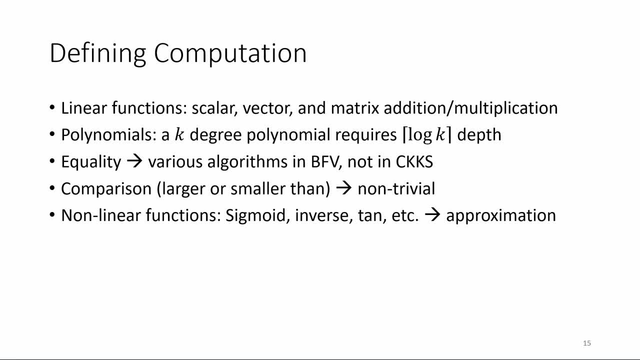 You can have polynomial evaluation: K degree polynomial. It usually requires log-d, log k. depth Equality check can be tricky. There are algorithms to achieve that in BFV. It's not possible in CKKS because CKKS is approximate. 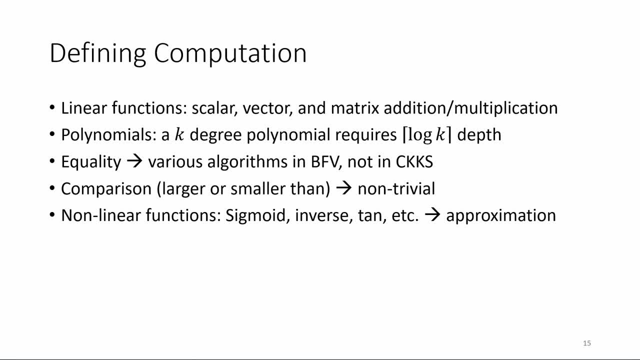 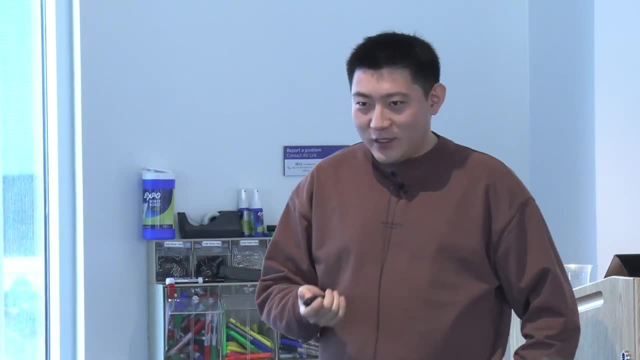 You don't get kind of equal. You always want to get equal. Comparison is hard. Comparison is hard because when you're comparing negative one and one module of five, it doesn't make sense. When you're comparing 0.9999 and one, they look similar. 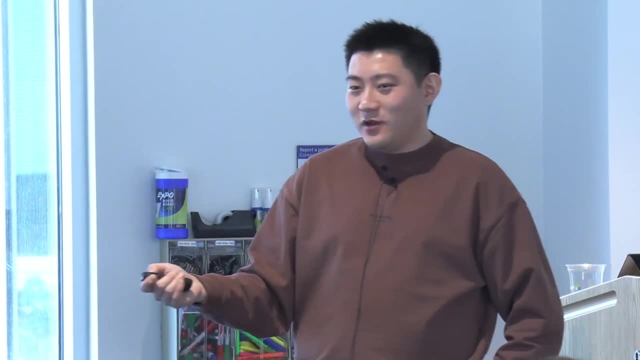 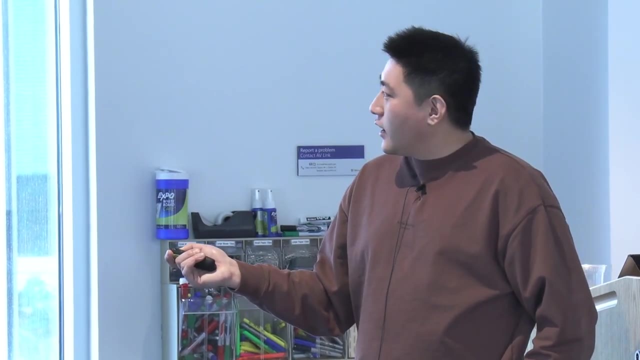 You don't even know whether they are equal or not. How do you know which one is larger, which one is smaller? So this comparison is kind of hard but it's not undoable. You can approximate the result with some height degree polynomial to achieve. 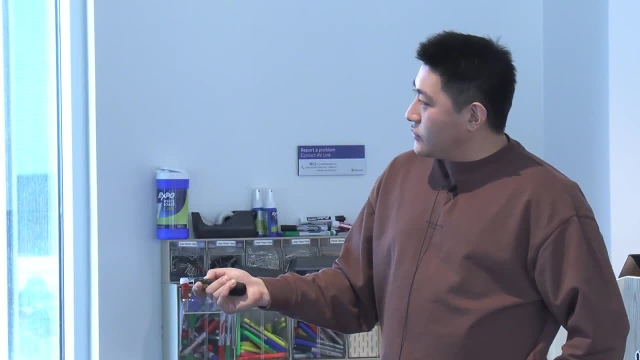 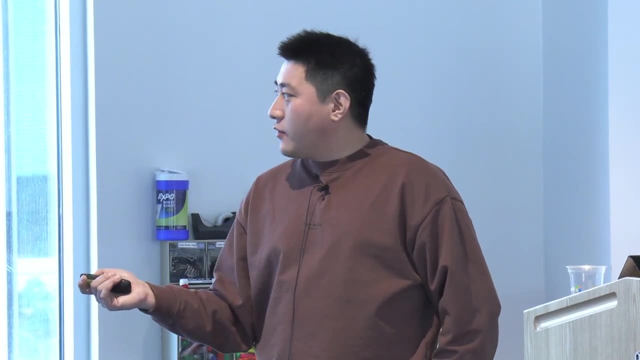 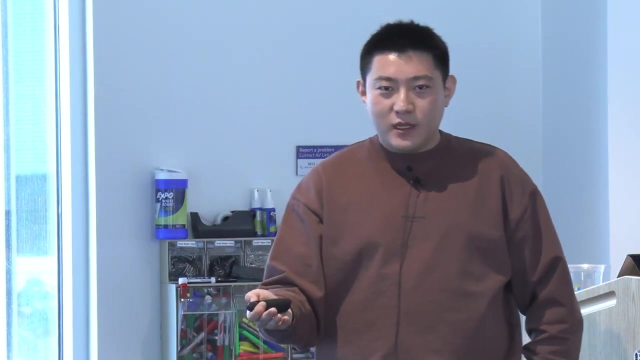 approximation of the result. That technique applies to nonlinear function too. This is sigma, Sigma, inverse, tangent or other functions. You can always approximate these nonlinear functions with a polynomial. If any one of you has ever used the MATLAB, you have the curve fitting those things. 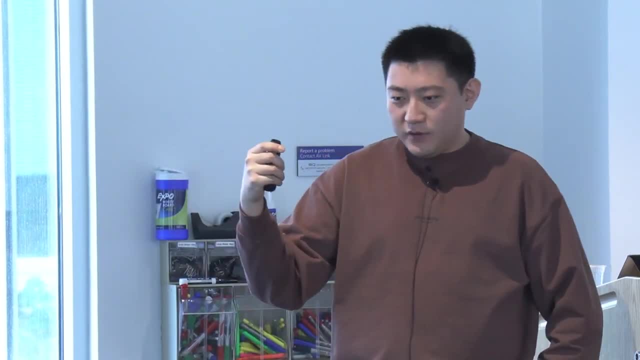 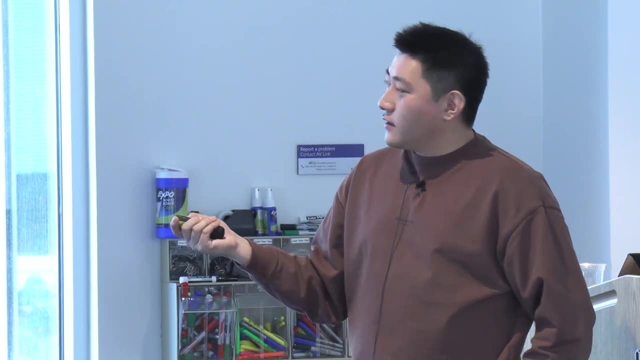 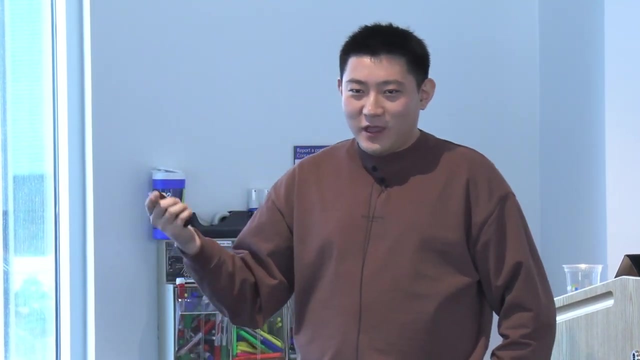 It gives you a seven degree polynomial to fit the curve. So you express approximation of the curve with a seven degree polynomial, which is HE friendly. So fundamentally HE can do all the computation, just with different cost, with different effort. So if anyone asks you that can HE do something. 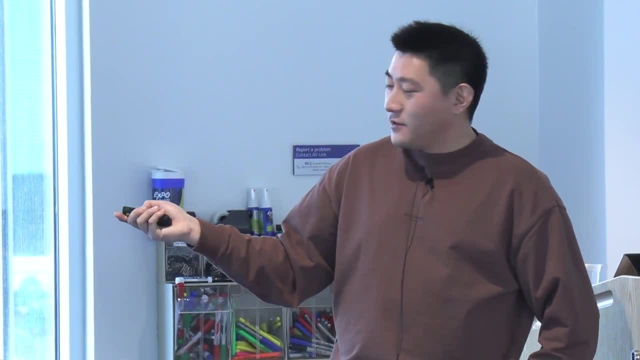 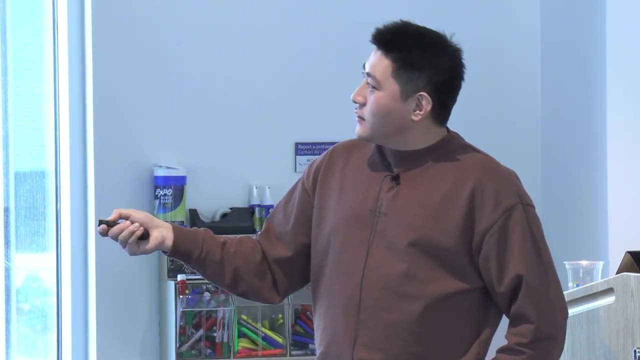 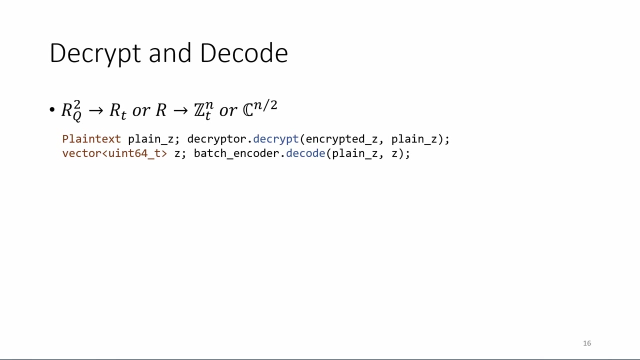 or I heard that HE cannot evaluate nonlinear function. you say that's not true. And finally we get decryption and decode. Decryption and decode. just first, decryption map the pair of polynomial to a single polynomial, which is plain text, and then decode it to the vector. 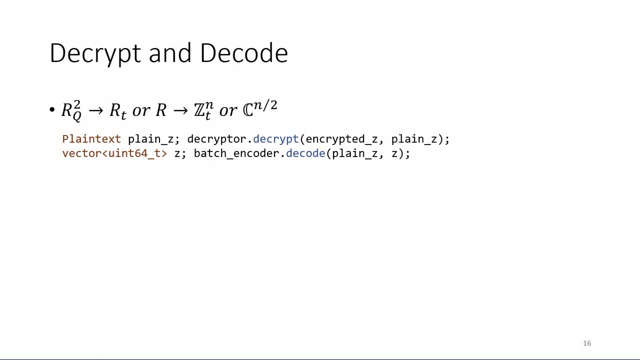 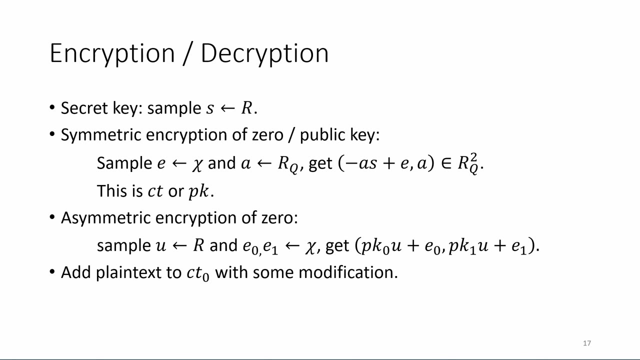 And there's your result. So we decrypt z. calling this, You decode plain text z. calling this, You get the result stored in z. So super simple, two lines. How does the encryption decryption work? We can get a little bit more in detail. 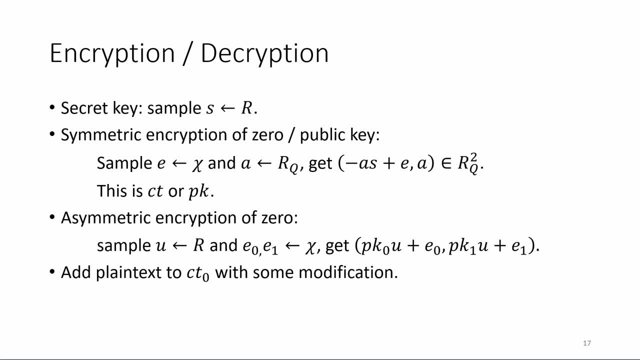 Basically you generate a secret key which is: s It's a polynomial from a ring, Then you usually secret key can be just a ternary polynomial means the coefficients are minus one, zero or one. They are very simple polynomials. 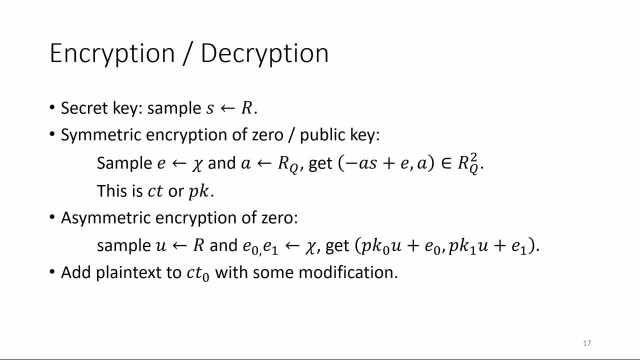 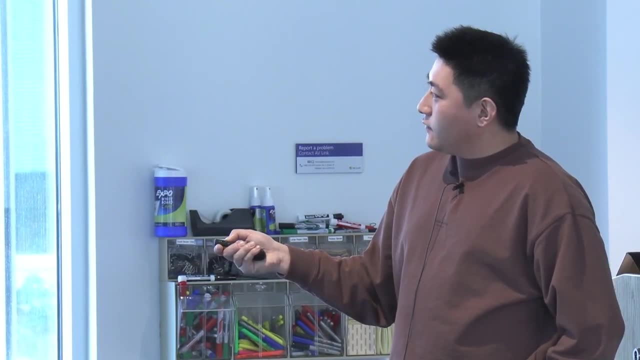 You can read it actually. For example, we can support symmetric encryption of zero. You just generate an error. e- it's also a polynomial from a discrete Gaussian distribution is: give you a random looking ciphertext. You also sample a, which is uniformly sampled from RQ. 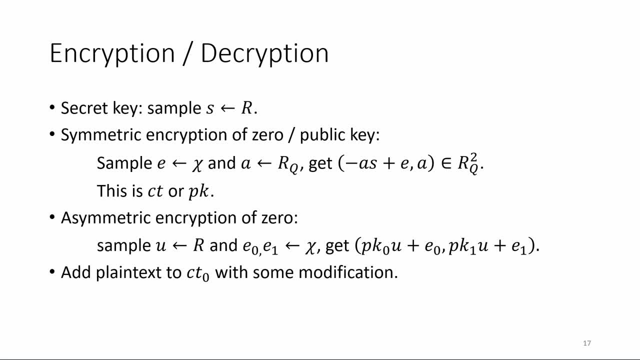 So a is module Q polynomial. You publish this thing. This is minus a times s point zero, Plus e some polynomial arithmetic happening here. You get the result And the second polynomial is just the a. So these pair of polynomial is a ciphertext. 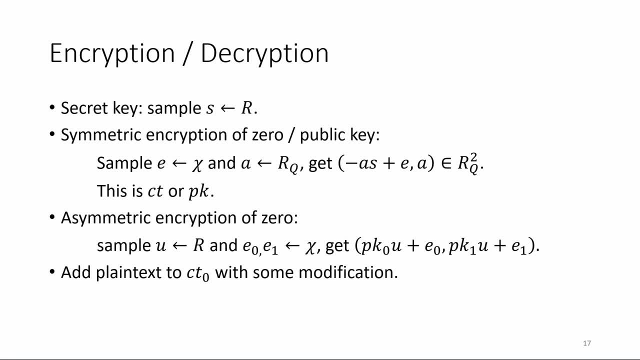 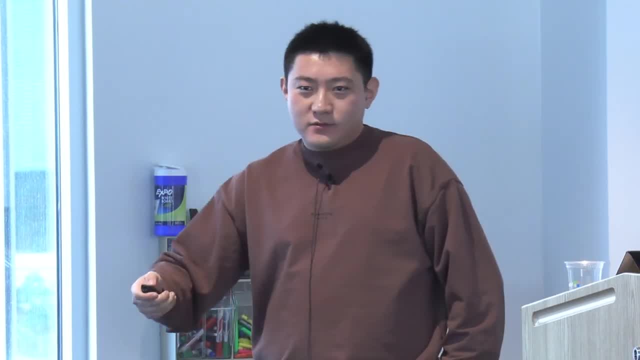 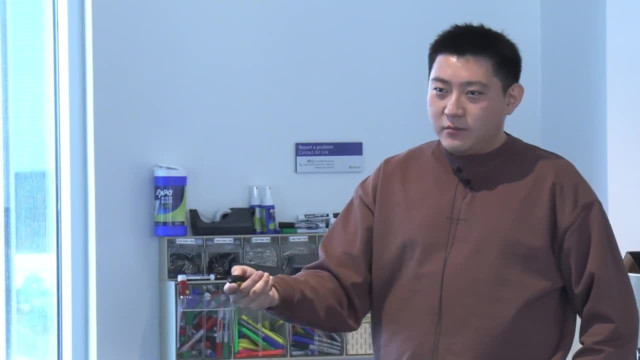 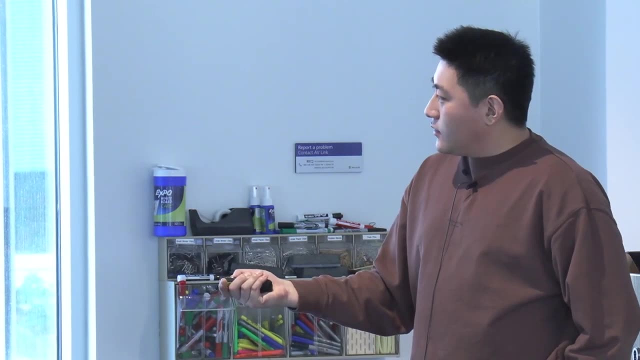 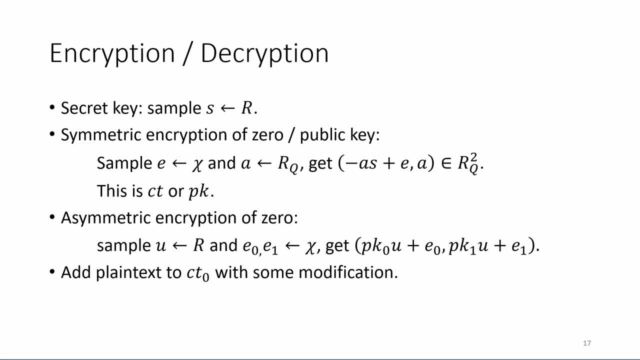 is two polynomials: pk0 and pk1.. You sample a? u from the same distribution here. that is a polynomial ternary. You multiply it to two polynomials here And you add two new errors, And this is your asymmetric encryption of zero. 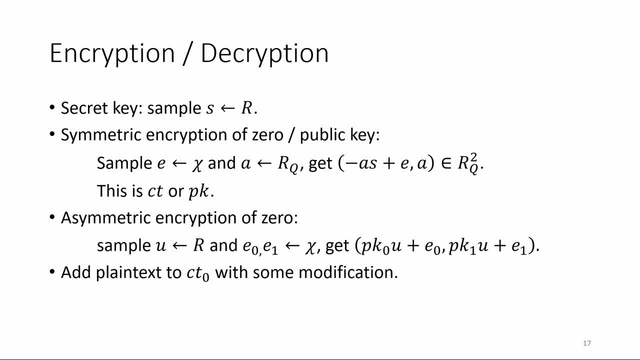 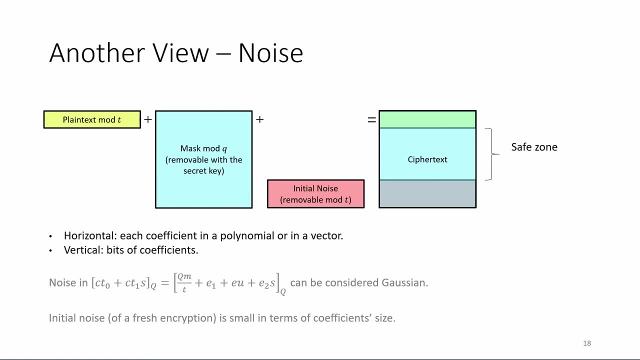 And when you want to encrypt some true value, you just add the plaintext to this part with some modification. Then you have the ciphertext and encryption of some true value. Another view is that this is your plaintext. This is the mask module Q, for example, A times S. 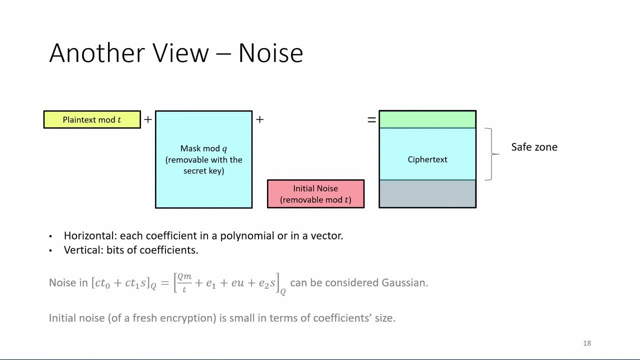 This part is removable with the secret key during decryption, But it's a huge noise. So horizontally, this is degree 0 to degree n, n minus 1.. Vertically, this is, let's say, the least significant bit towards the most significant bit. 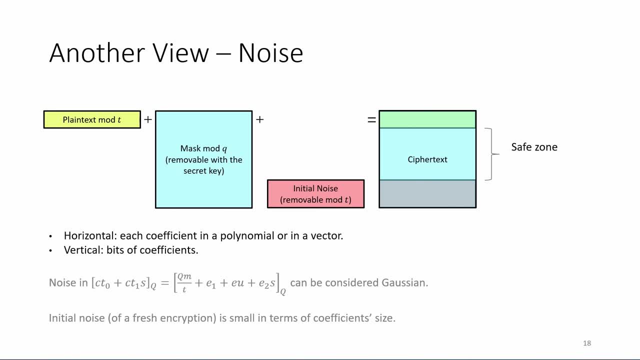 So here you should have log Q, here log Q's bit, And this is the 0th bit of your coefficients. So let's assume this is a polynomial And you can see this is like a large error. You are just masking the whole message space. 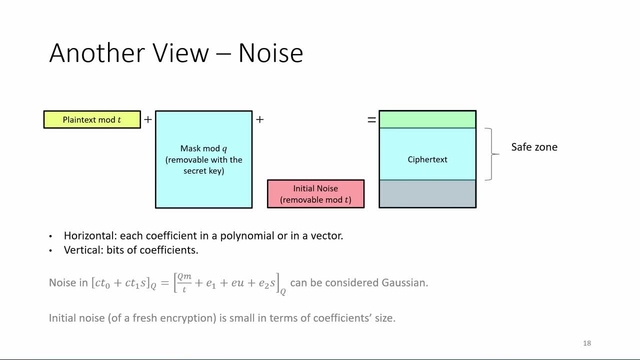 OK, So you can see this. All the information are randomized and masked with this thing. You also have some initial noise which is introduced with the E. These are considered small. What you do is you lift your plaintext by some constant factor. 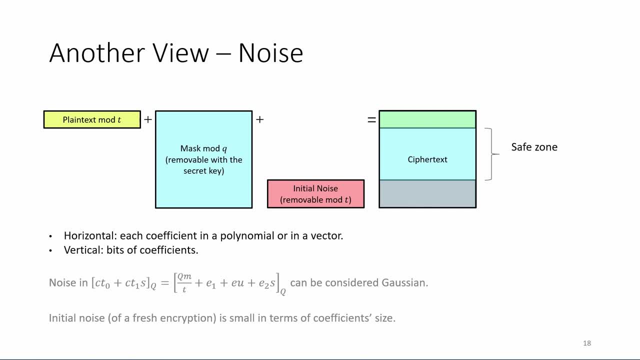 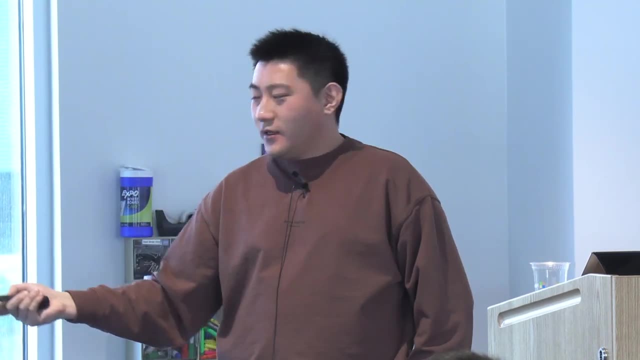 Let's say this is a BFE encryption. What you do is you calculate Q over T, something close to that. Let's say your T plaintext modules can be some BFE 1,000 or a small value. The Q are usually large, a few thousand bits. 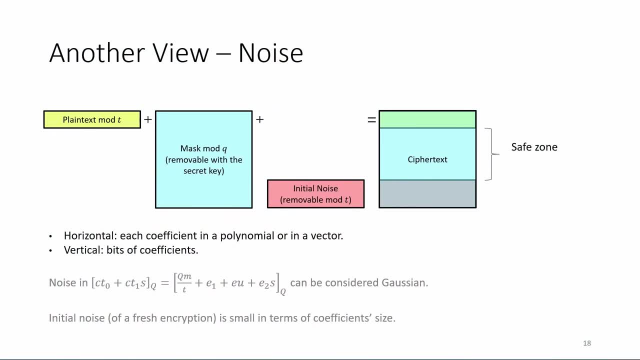 You get a very large ratio here. You scale your plaintext up by this ratio to raise it from the lower bits to the higher bits and you add everything up. you get this. You can see there's a safe zone here that separate the message from the noise. 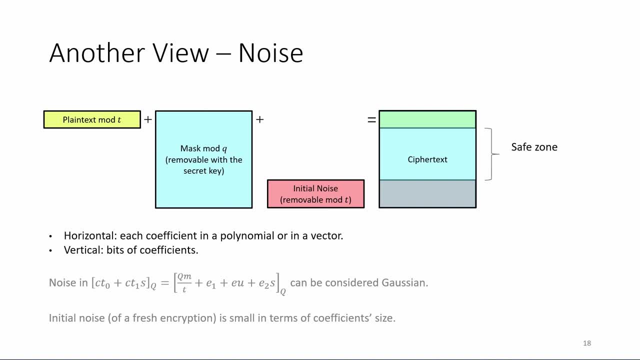 and this gives you correct decryption. If you lose this, if the plaintext and the initial noise start overlapping, you start to lose information. In BFE, decryption will fail. In CKKS, you lose precisions Along with the computation. this noise will grow. 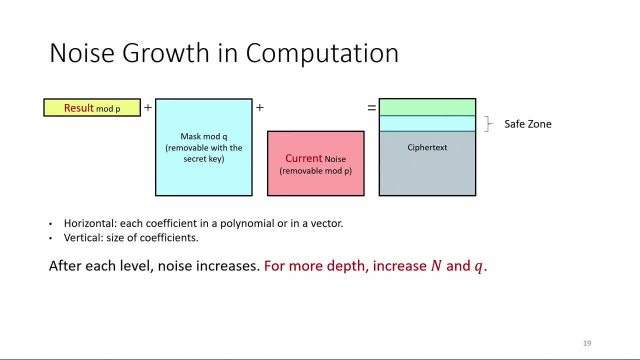 This mask is not a problem because they are always removable with the secret key, but this noise will keep growing until eventually will destroy the safe zone. At that moment, your decryption will fail. Multiplication introduce the most noise. That's why we want to minimize the depth. 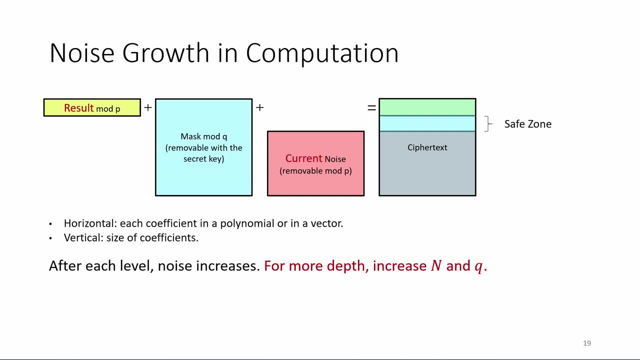 Cyberdeck-Cyberdeck. multiplication cause a lot of noise. You want to do them in a tree-shaped rather than in a chain. Let's say, if you calculate the y to the power of four by doing y times another, y times another, y times another y. 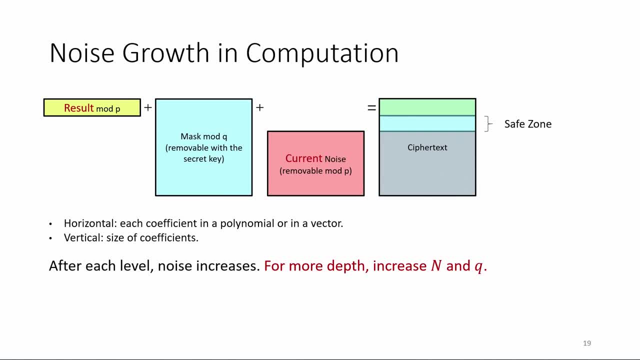 you will end up with depth four circuit. If you have more noise, my code might fail. The decryption might fail because the depth is much larger. However, you cannot always do things with two depths, so you need to have more depth. You just encrypt n and q. 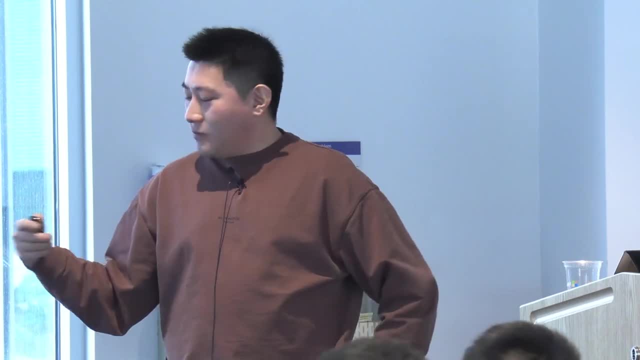 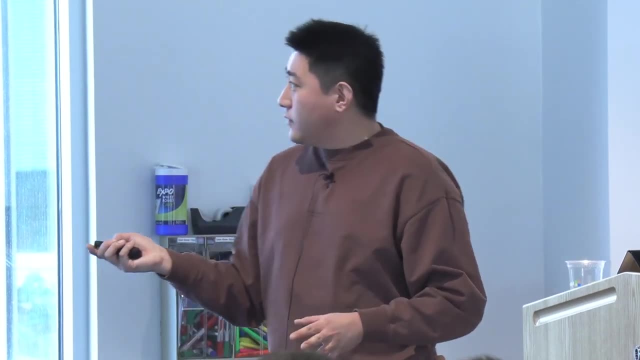 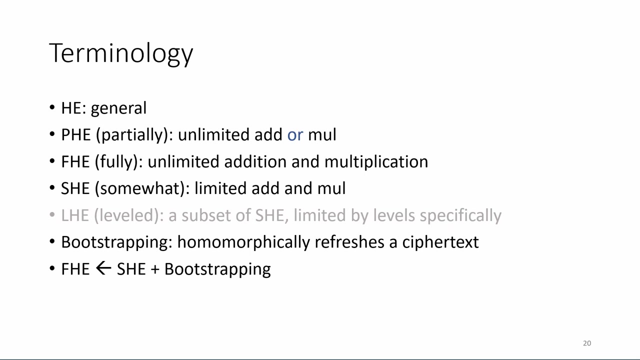 Once you know the depth, you should encrypt n and q to meet those computation need. I will explain how to choose n and q security to meet security need. Here are just some basic terminology. You might got confused a lot of times. I'll just leave it here. You can check it online. 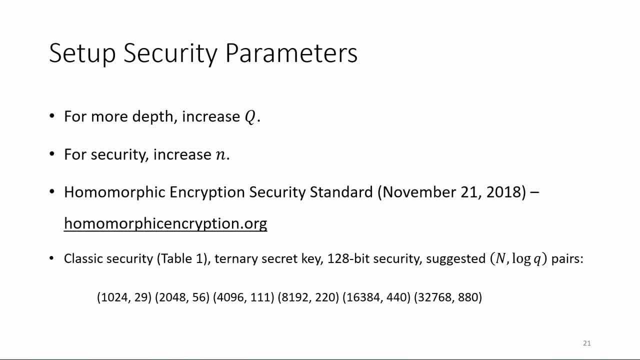 So how to set up these security parameters. We are going back to the beginning. If you want more depth, you should increase q, because you need to draw the plain text or the ceiling away from the noise. So you increase the vertical space by increasing q While you're. 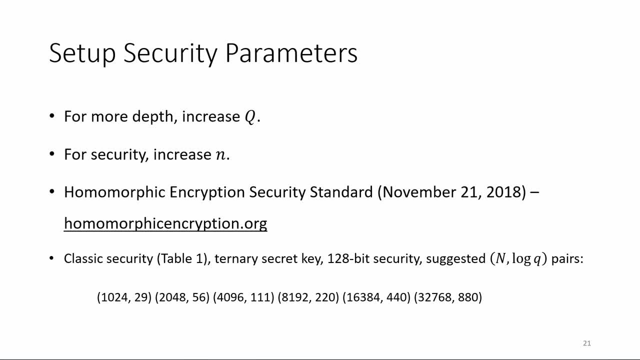 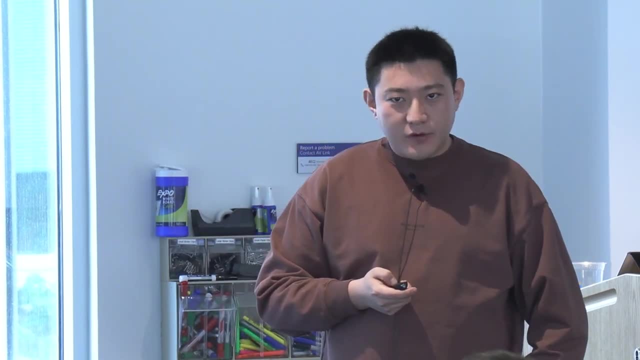 increasing. sure Is there a way to find the minimum q that it needs? Usually it requires some attempts. It's hard to just calculate the minimum q. There are a lot of papers doing noise analysis. It's very hard to do. 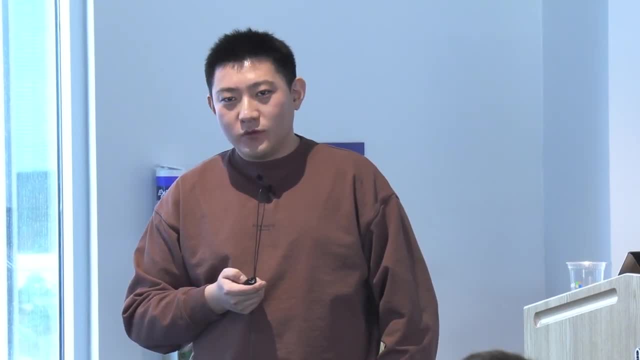 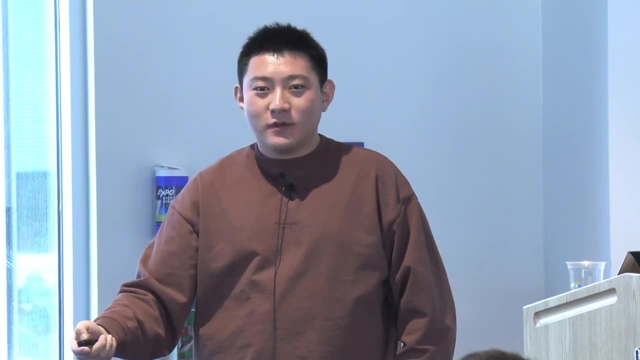 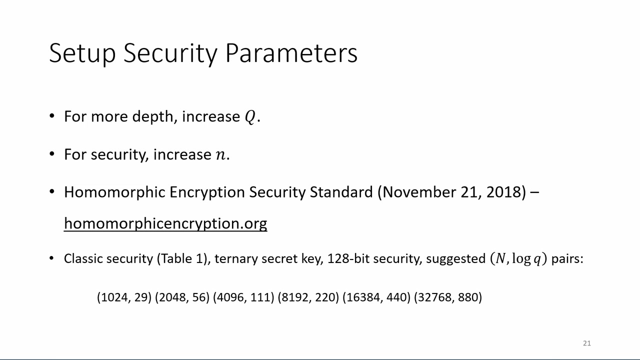 Usually the best way is just to start with the q, try to evaluate the circuit. If it fails, increase q. and if it fails, increase q. That's the easiest way. Then, after you decided on q, you need to also increase n, because the security definition. 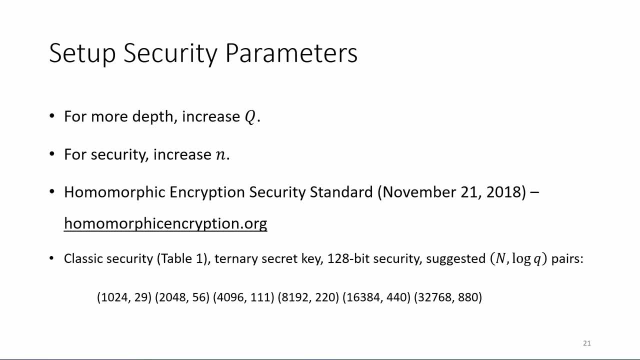 is for a given n. the larger the q is, the less secure the scheme is. So to make the larger q secure, you need to increase n as well. You can always choose parameters according to homomorphic encryption security standard. On this link you can find that: 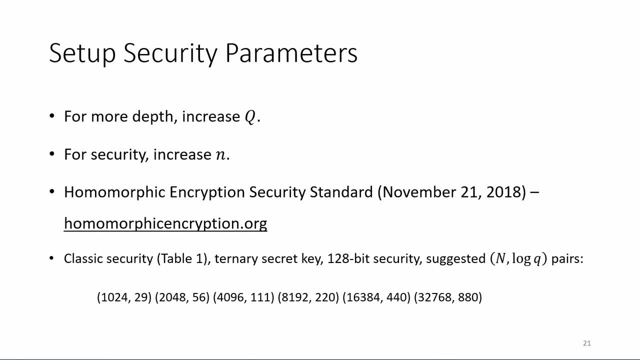 For example, in the table one you can see you have classic security ternary secret key 128-bit security. suggested pairs are: n is 1k and the log q is 29.. You just need to find a 29-bit q. 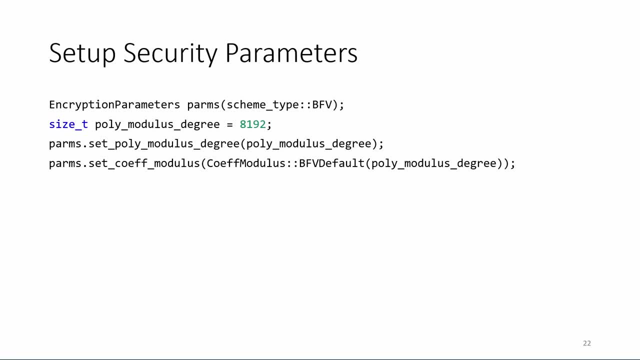 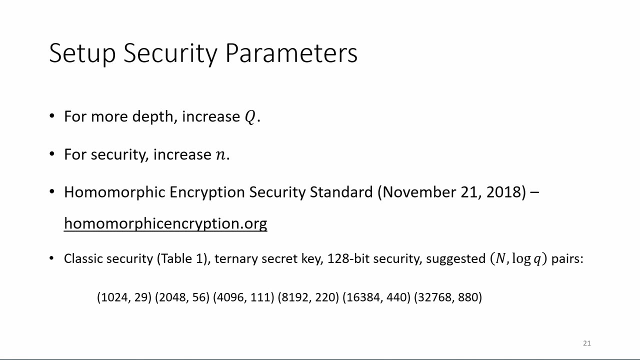 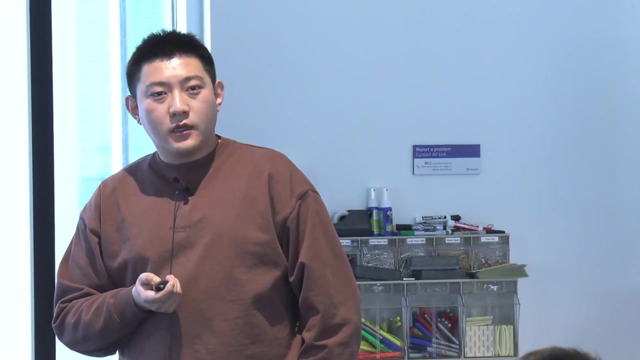 These are just four lines to set up the security parameters. First you choose the scheme, then you choose the degree and you choose the default Default q. using seal I mean log q, q to be a power of two, Let's say two to the 29,. for example, 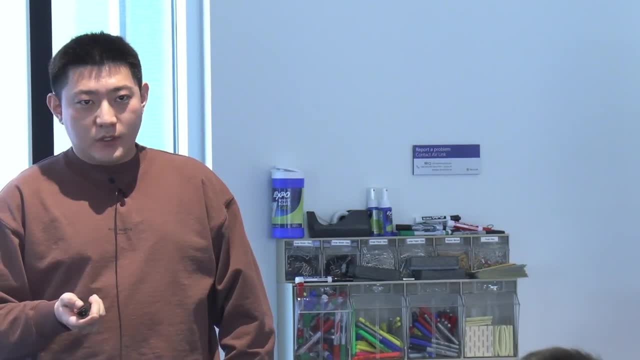 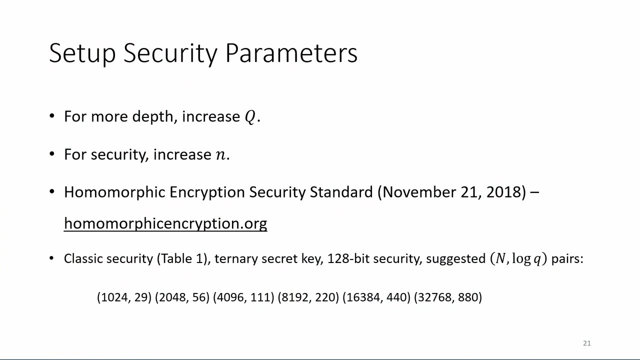 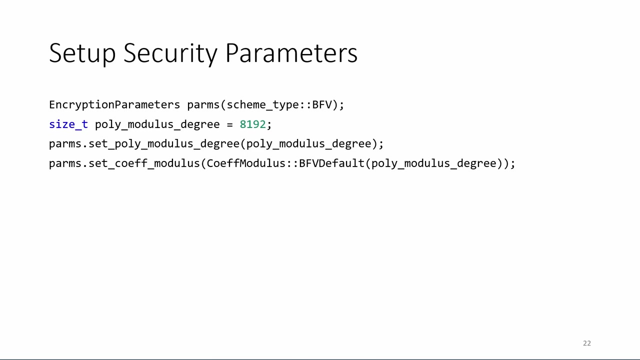 Yeah, You can take q to the power of two. You can use a power of two, but I need to explain in the future- next, I think, a few slides more. You will see that we don't use that. So this is very easy to set up secure parameters if you want to. 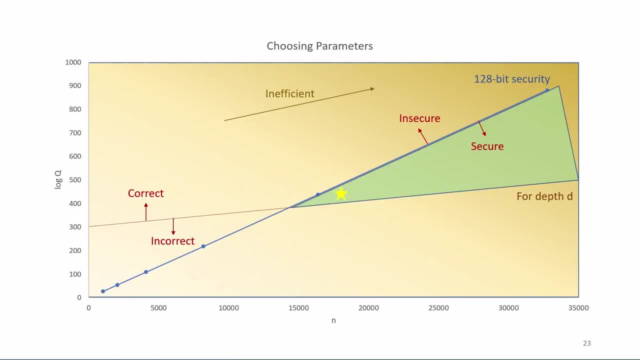 use some default parameters from seal. Well, this is a better view to choose your parameters. Let's say this: n. this is log q. the y-axis is log q. This blue line marks the 128-bit security threshold. Above it is insecure. 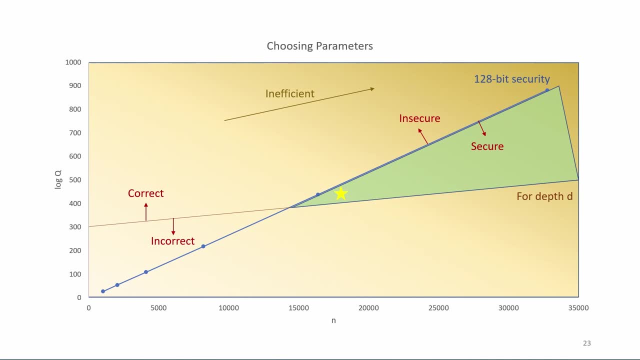 For a certain depth or a certain function, a certain circuit. this brown line marks the correctness. When your q is larger than these, you get correct decryption. You are looking for parameters from these triangle and usually when q and n gets larger, 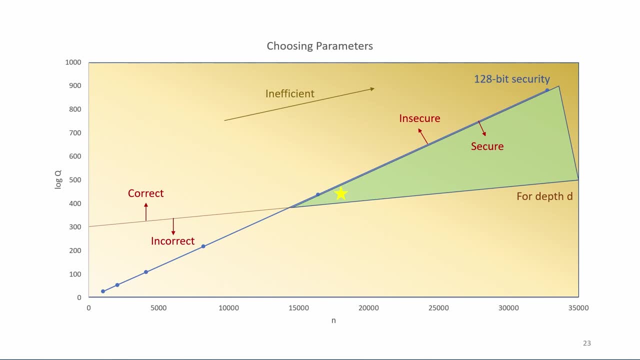 the program gets more inefficient. So this is the optimal choice. How do you according back to that questions? you probably will start with a q here and turns out it's not correct. You increase q to something here- turns out it's correct, but there's a space to reduce it. 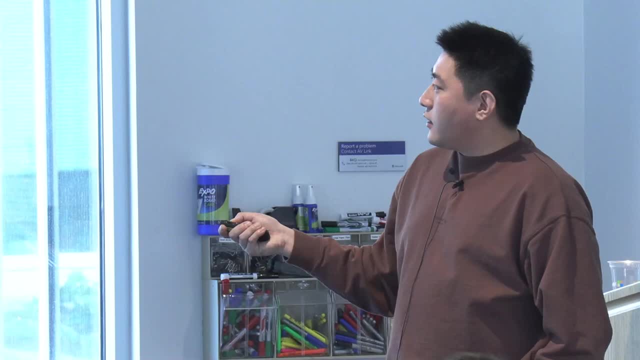 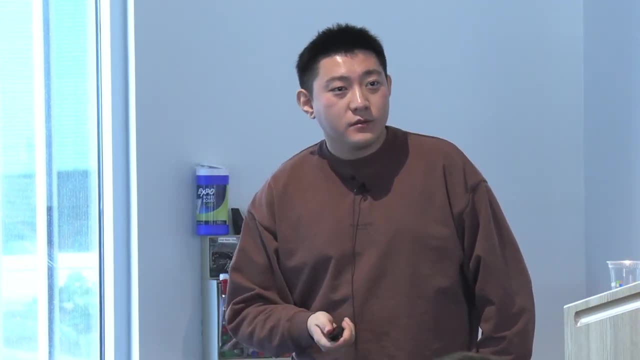 then you reduce q to somewhere here. Okay, Using the same n, you reduce q to somewhere here. Now you get the optimal parameters. Decryption will fail. You don't get the correct decryption result. Wait, you can't say correct. 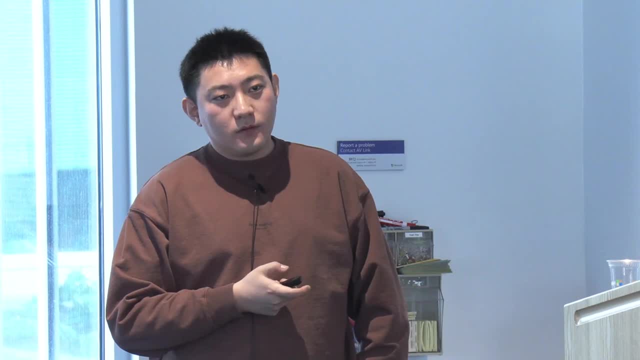 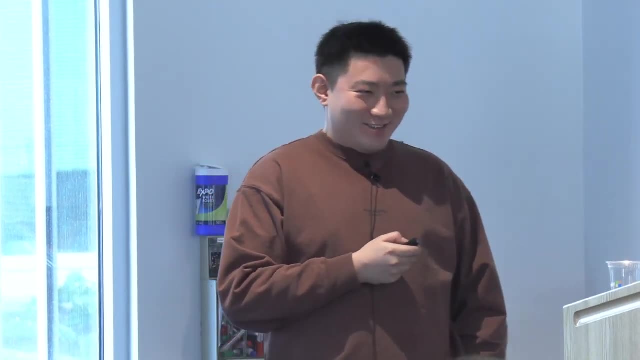 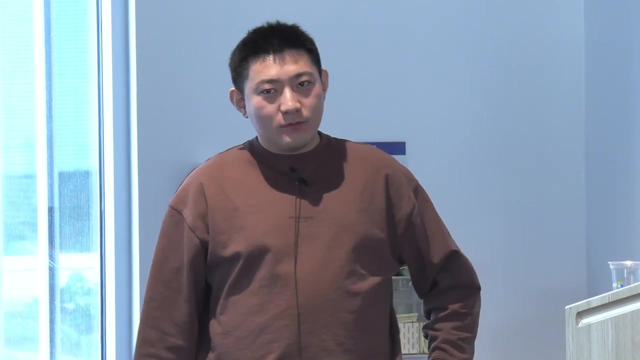 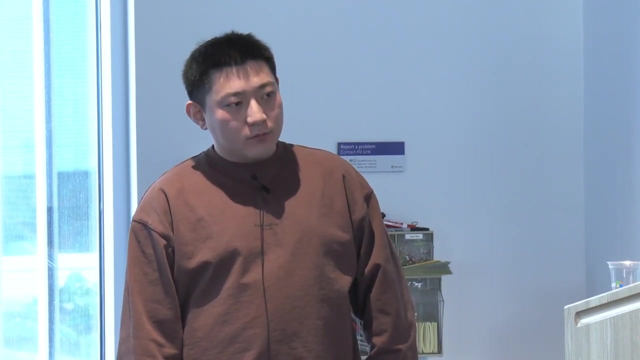 Good question. Most of the time, I wanted to make a comment on that question. So, going back to 2014,, we published a paper with how to compute the correct parameters. so q and n noise starting from d. So if you have the depth, 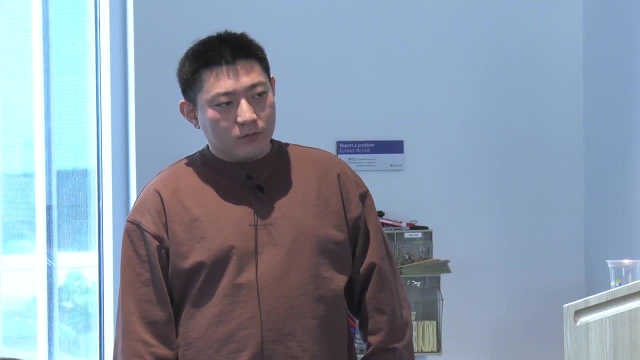 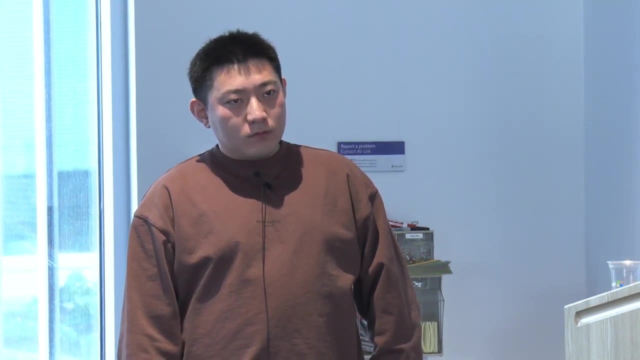 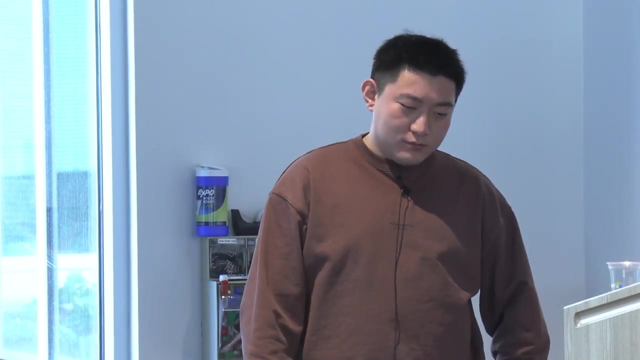 like you know what you want to compute, we gave an algorithm. you can mirrors it and compute the q and the n that you should use. So the only problem is- And so it'll mean- that her parameters will be like overastimate of what's necessary- 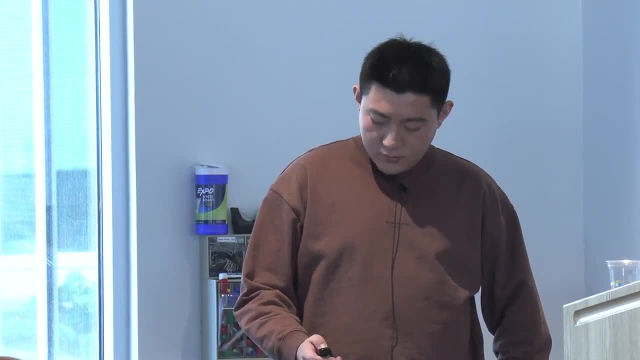 And if you're really interested in performance, you might want to do a little better than that, which is, I think, why you could also do this. just try and you know, and it works, it's nice. You could also do. I think that you know you could also do it as you catapult these features in the software and then you could combine them. 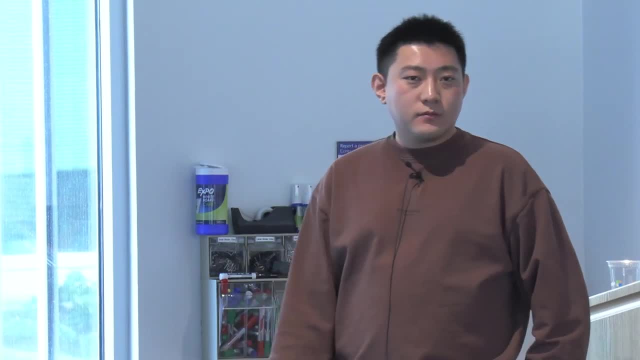 You could. you know you could also do I mean with QN, and you could do Q and N in the crease until you get something. But if you want going to your last question, if you want to ensure that you will get correctness, 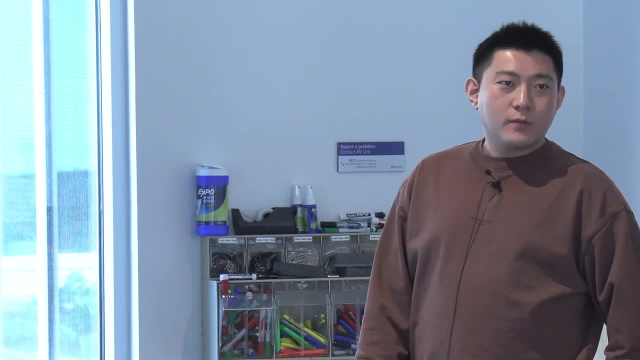 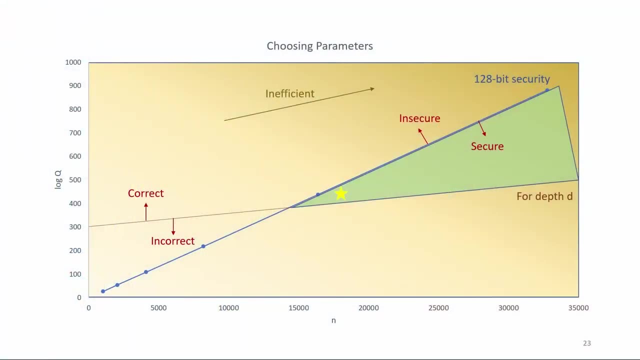 in security. these are all within it. It will give you a few of the parameters I think you probably using that. you can find another brown line here that give you the guaranteed correctness, which also give you a little bit worse parameters. 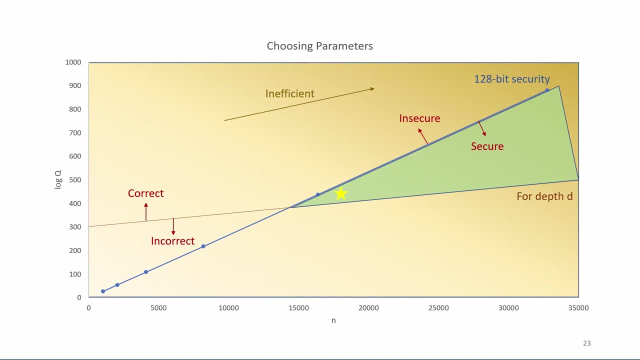 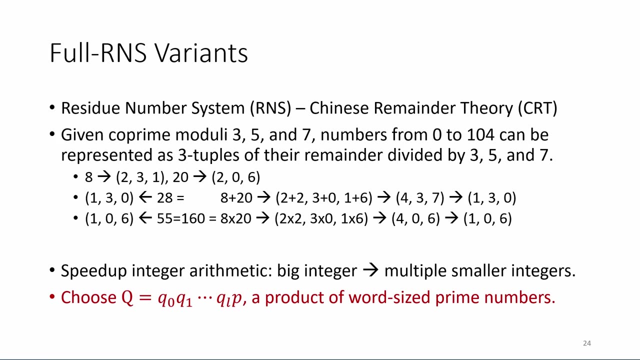 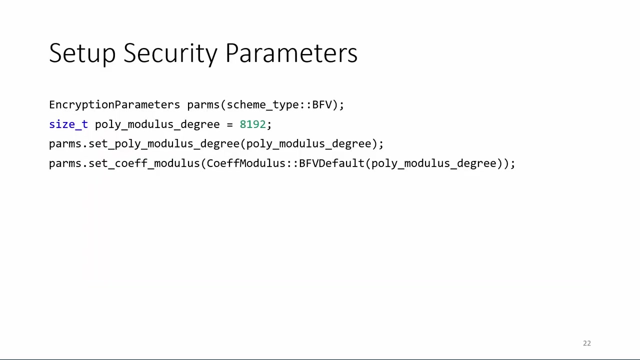 You can further find parameter within this letter shape area. So I'll start explaining what's the form of Q we are using. So the previous code: you only choose a default parameter to set up the coefficients. So, compiler, That's the part of CL. 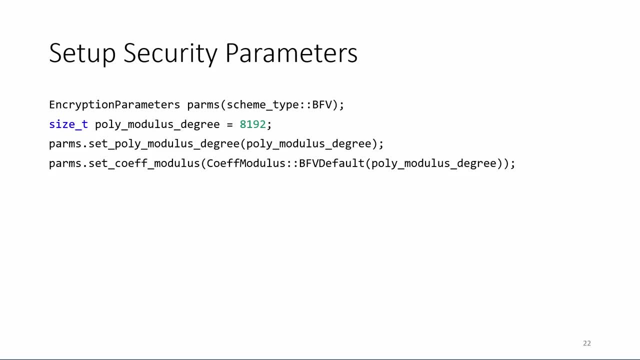 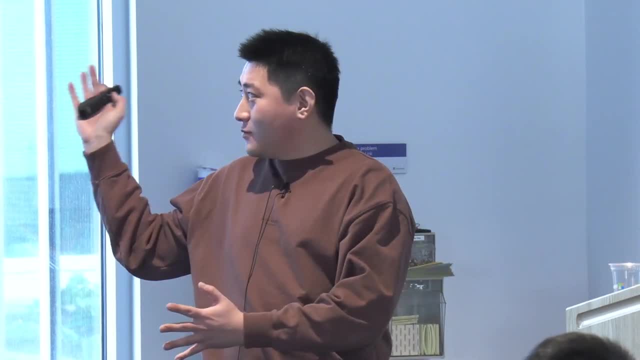 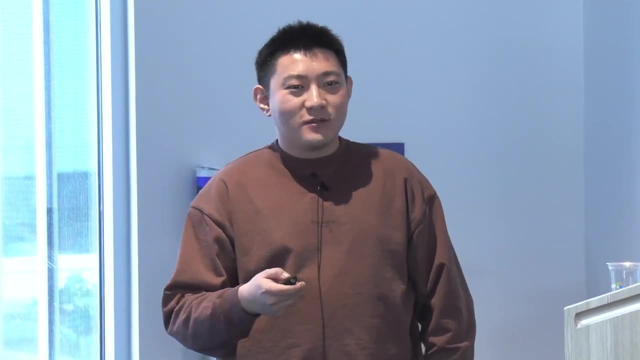 That's our plan actually. So, for example, I think you know and we can talk about that- we are working on a compiler that optimize all these procedures for CL. Focus on vector instructions. You have, Matt Roshan, right, Roshan. 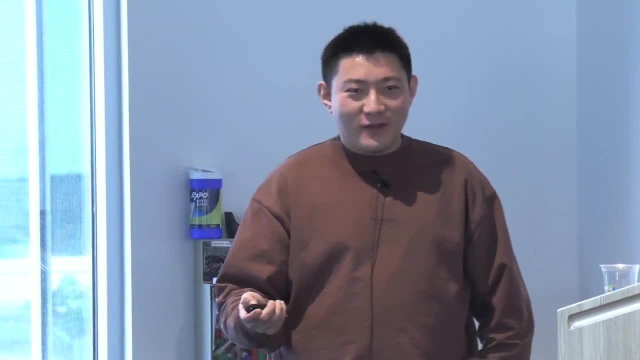 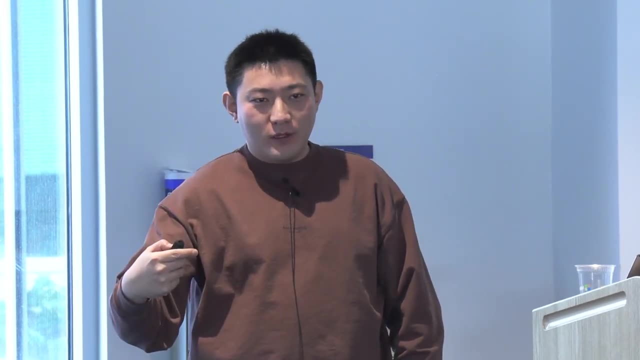 An intern last year. We'll be working on that and we can get rid of a lot of these parameter settings. Just rewritten. write your code. the compiler can work it for you. It does not get you the optimal, but in most of scenarios. 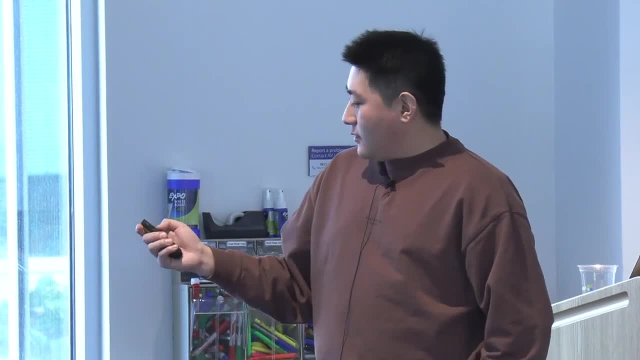 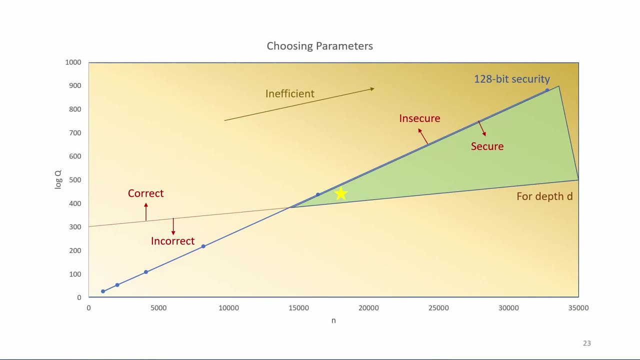 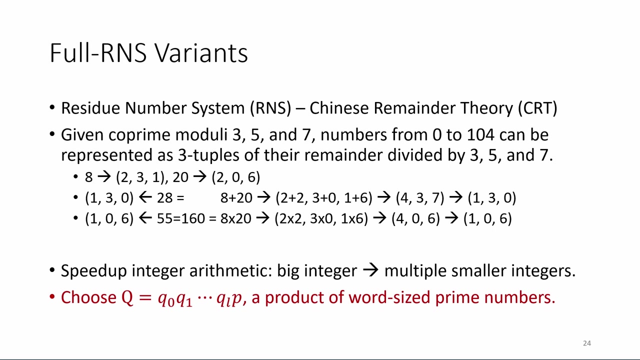 it's pretty good parameters, But again, that doesn't include the polynomial factorization. So then what's the form of Q? So we need to talk about this full RNS variance. We need that in later talks. So RNS is residual number system. 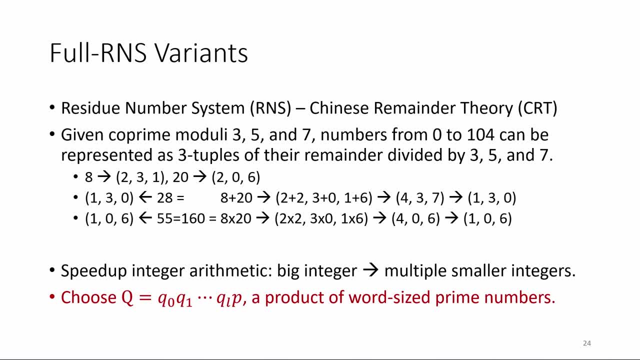 or it's similar to Chinese remainder theorem. Basically, you represent the large integer with a set of smaller integers. For example, if you have co-prime module i, three, five and seven, you can represent numbers from zero to 124.. 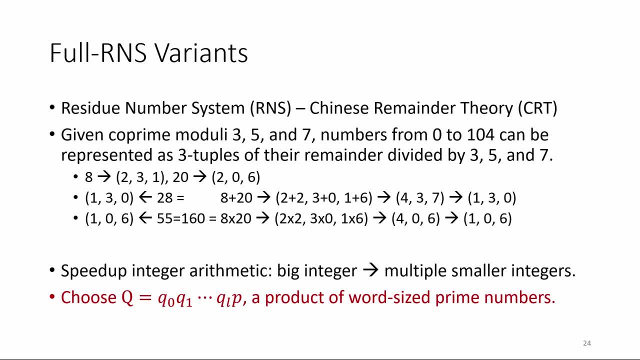 Each one will be represented by a three-tuple of the remainder divided by three of them. So, for example, eight becomes two, three, one. Next module three, module five, module seven: twenty becomes two, zero, seven, Six. Addition are done element-wise. 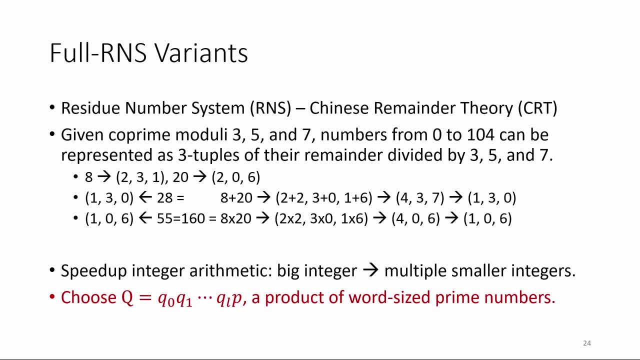 By doing this from here, you get one three zero. If you just calculate the mapping of 28, you also get one three zero. So this applies to addition and multiplication. By using these we break large integer arithmetic into. 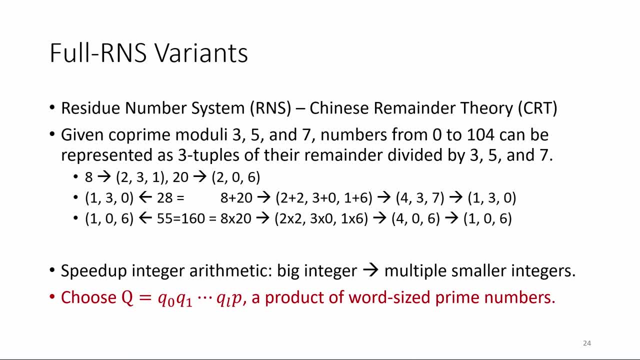 a set of smaller integer arithmetic and gives you a lot of speed up. This is very important. Most of the RNS schemes are better than their original RNS schemes. Consequently, we choose Q as a product of smaller word size, prime numbers, As you can see before from these parameters. 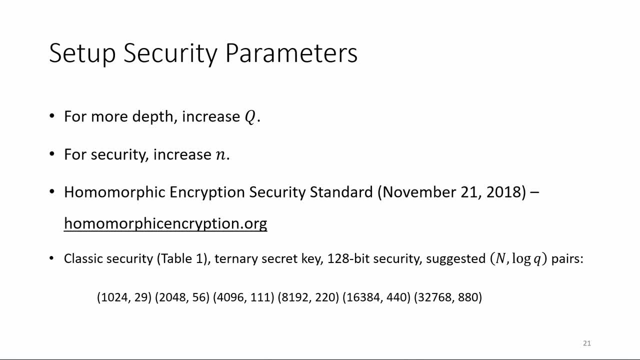 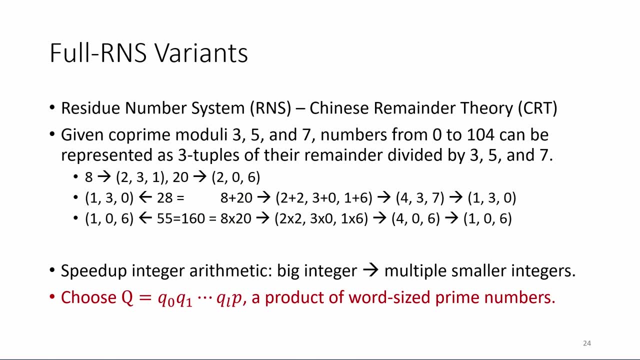 Q can be a few hundreds bits large. Computer cannot process that without like a number theory library or hyper-extension library, But we can use RNS system to achieve that and it's very efficient. The consequence is we need to set up QIs and P. 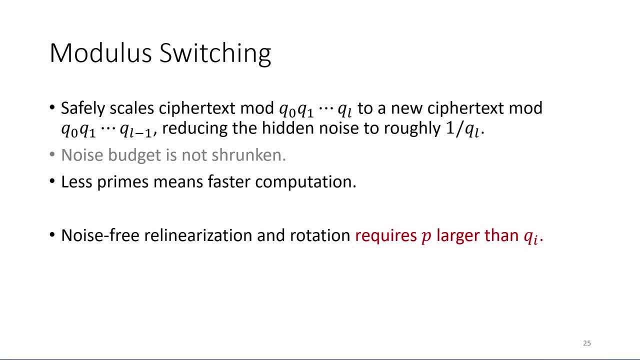 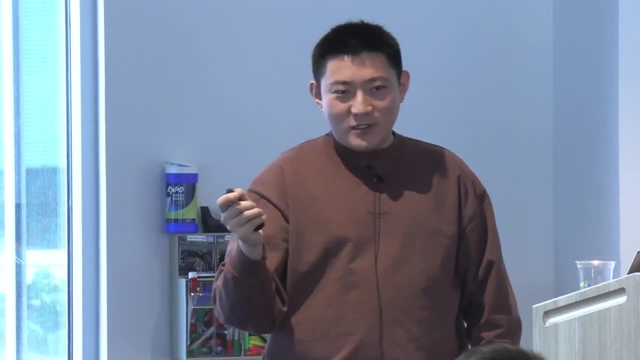 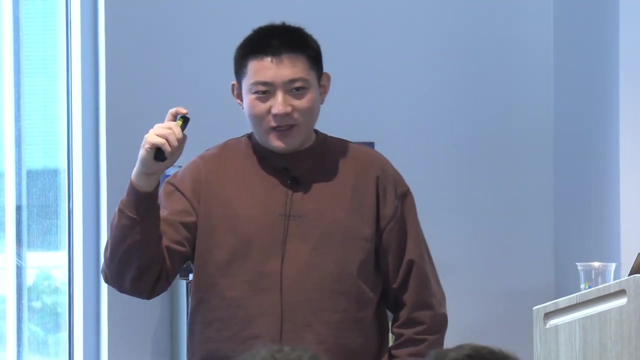 There's also another operation here during the computation that you can discard something, a prime, from that Q. So your subtext got smaller in terms of coefficients. It's a safe operation. You can discard some of them, Your computation gets faster. The safe zone is preserved. 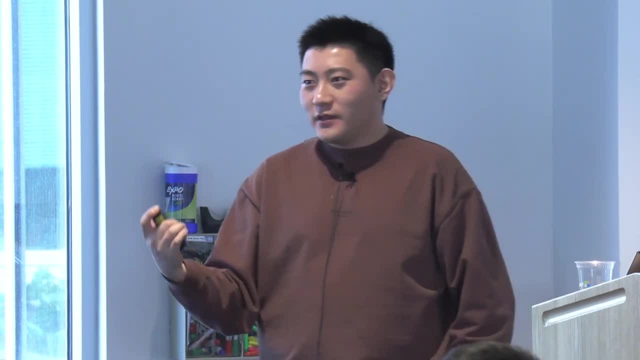 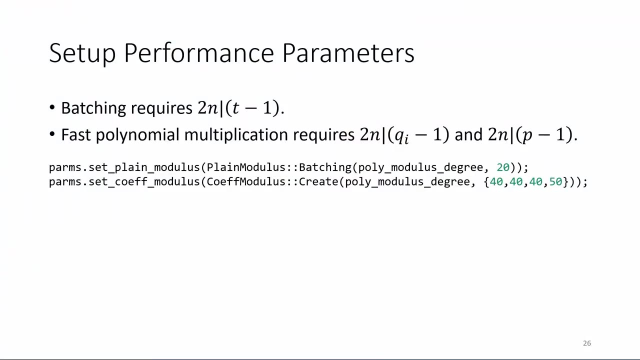 And it's very beneficial to get better performance, And we'll need that in the future, like slides in future sessions. So then, how to set up the performance parameters Before we are just using, let's say, set co-op modulus, BFE default. 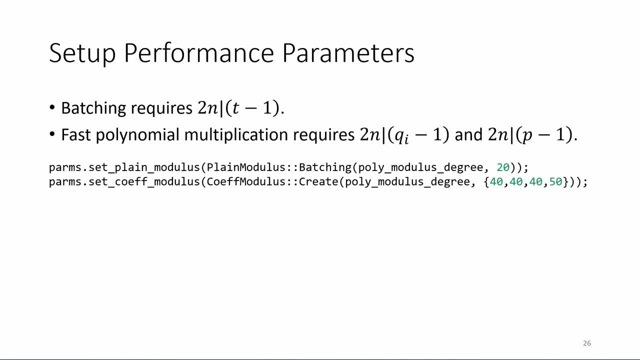 That was the previous example, But you can do something better by giving four prime numbers. You can either write in four prime numbers here as a vector, or you can just tell the CO to create four prime numbers. These four prime numbers have 40 bit. 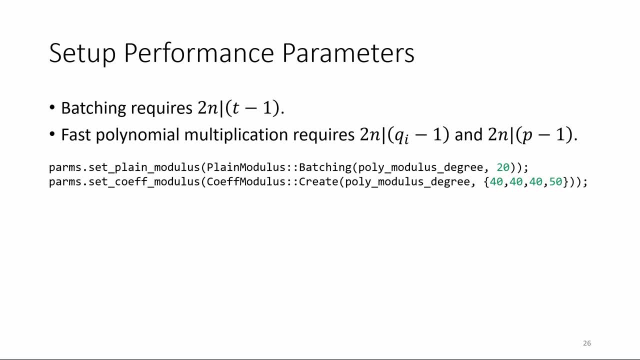 40 bit, 40 bit and 50 bit. This is very simple. You just tell CO: okay, the Q size cannot be more than 270 bit. So I choose four primes in total of 170 bits And you just pass these four values to the function. 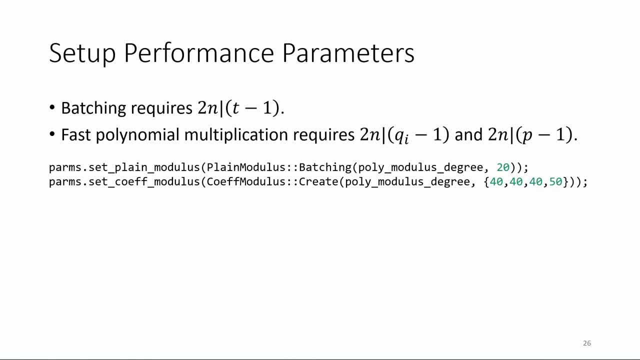 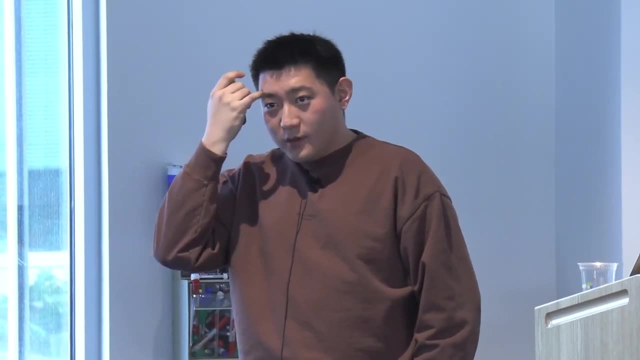 and it creates four primes for you. There are some requirements. The last one is with largest, so that you have less worry about noise during some operations. Just always make it the largest. If you choose four of the same size, I remember CO will choose the largest for you. to put it here: 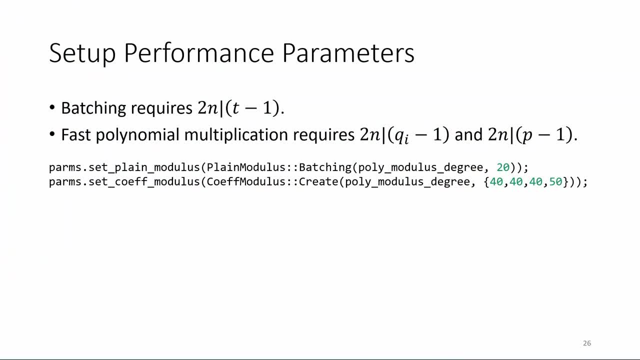 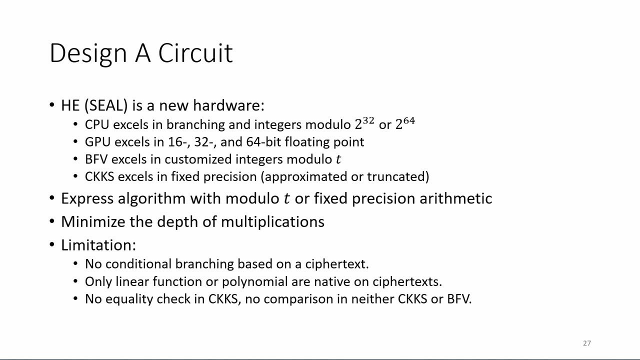 So that from here, we don't need to worry about what the primes are. You just need to worry about their bit size, And this is important to use in CKKS For efficiency. This is just some basic idea To summarize everything. let's go back to the same correct order. 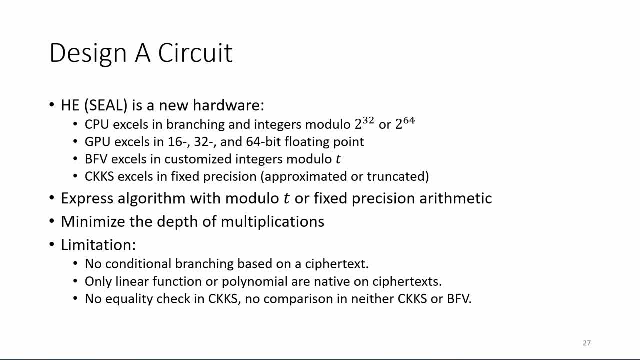 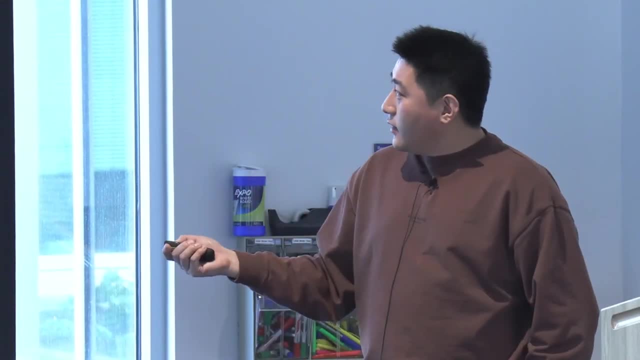 You start with an idea in your mind to do some algorithm and application function. You need to write it down as a circuit, HE-friendly circuits. You should think HE as new hardware rather than some encryption or arithmetics. fine, So CPU. 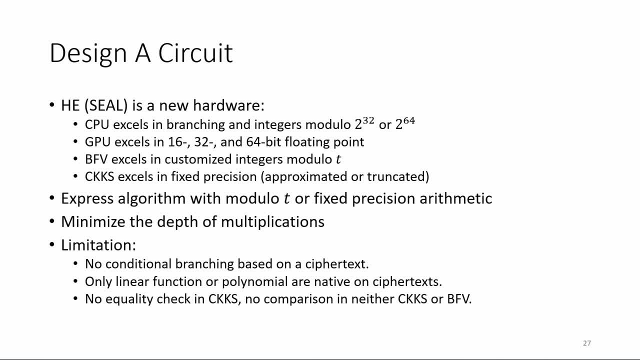 works on instructions and good at branching and integers module to the 32 or 64.. GPUs are better at half-precision, single-precision, double-precision, following points, And BFB just is good at integers module, T or arithmetic. CKKS is good with fixed precision or truncated approximated computation. 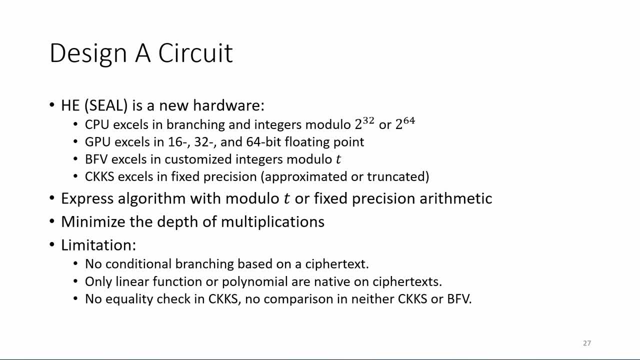 You just write your algorithm in a different way And then you express the algorithm. with these, You get the minimal depth. Based on the depth, you can choose your parameters, And there are some limitations here. Of course, you cannot do conditional branching based on. 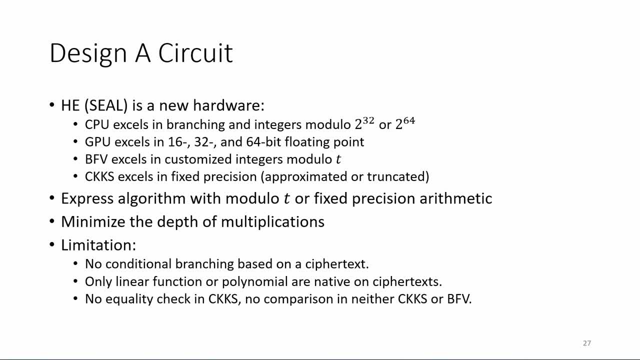 the ciphertext, because you don't know the ciphertext, You don't know the secret. But there's another way to achieve something similar, which is a practice question. You can solve it later. Also, these two also nonlinear functions or also not polynomials. 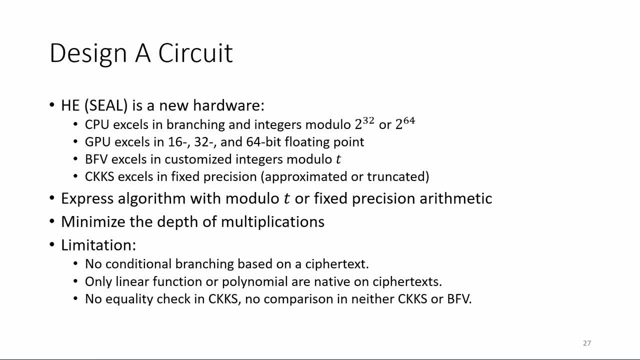 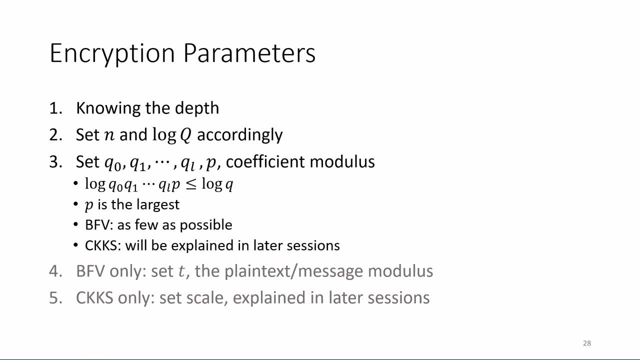 they require some approximation, which will be explained in the last talk today by Hao, And then you set up the secure parameter, set up the performance parameter. This is not required if you are calling some default parameters And then you're done with parameter settings. 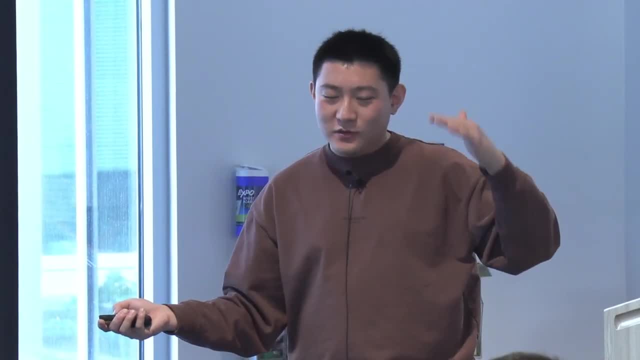 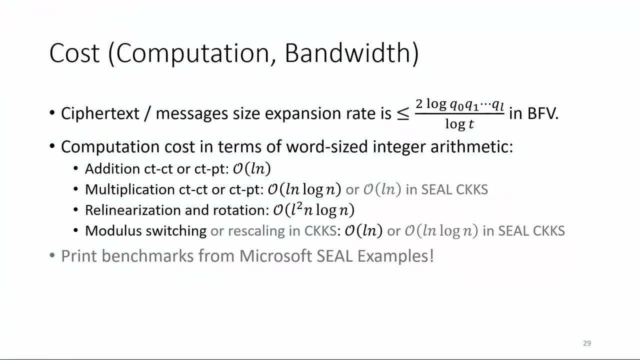 You will construct some classes in seal, but those are simple. simple. You'll show that in demo in two sessions after this And then you can define your computation. You can write down the code. When you write down the code, you need to remember: 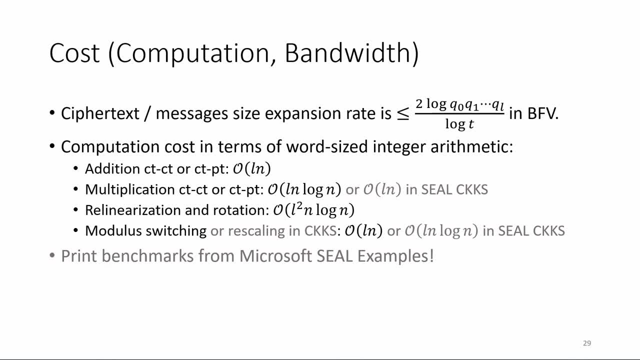 that each function have different cost. Here is just a syntactic view of the cost, based on the number of prime numbers you have and the degree n. You can see the multiplication and the linearization rotation are kind of heavy So you might want to avoid using a lot of them. 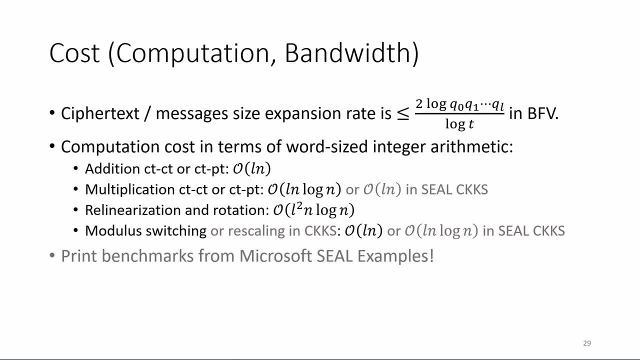 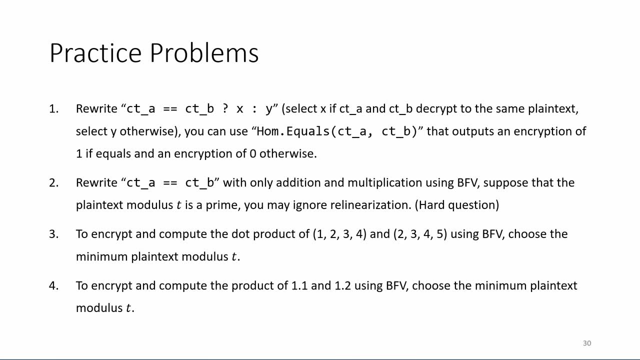 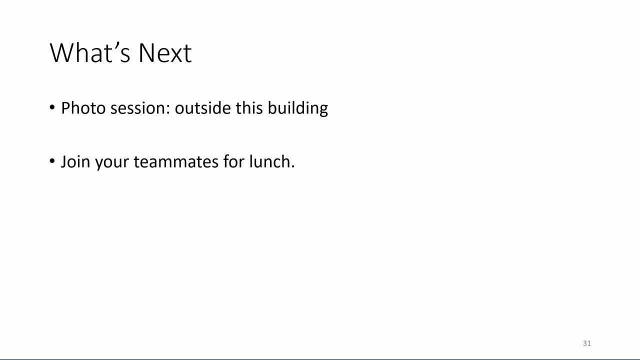 If you can get rid of one of them by introducing two additions, you should do that, And here are some practice problems And you can just try to solve these questions. If you have questions, just ask me And these slides will be available online. 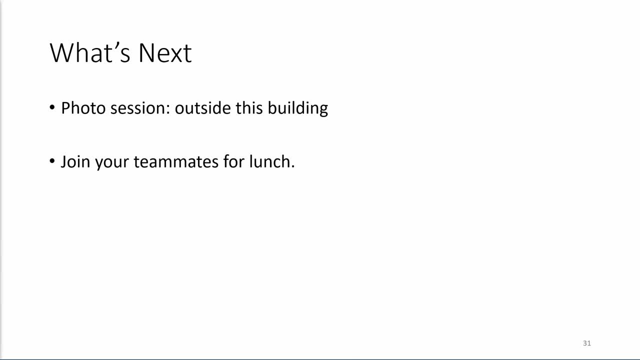 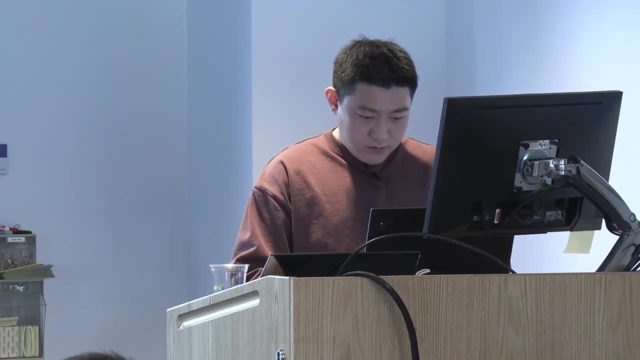 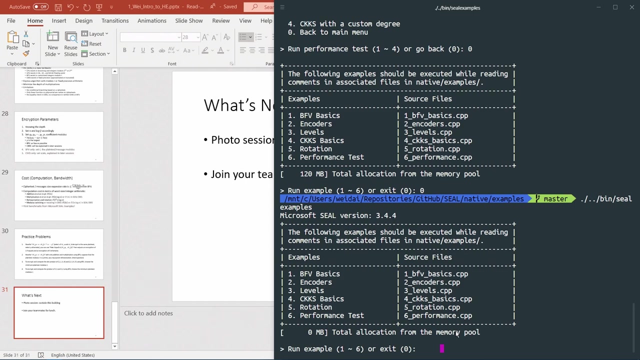 Actually, before that, I want to quickly show that how to measure performance. benchmark result in seal. So I'm running a seal example. Oh, it doesn't present. Okay, So here I'm running seal examples. If you just call this six example. 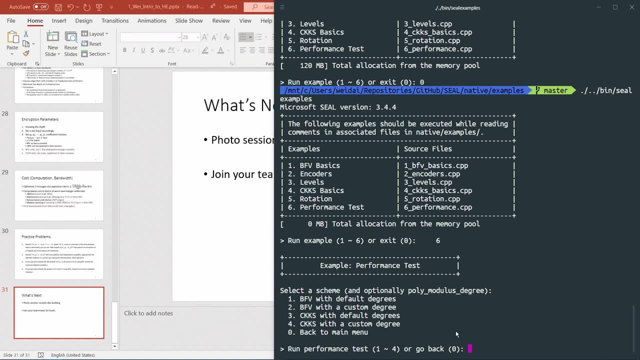 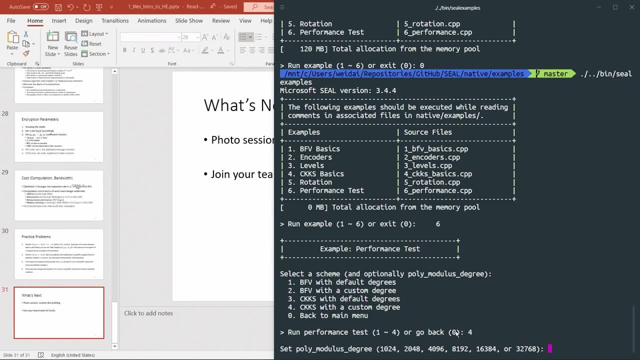 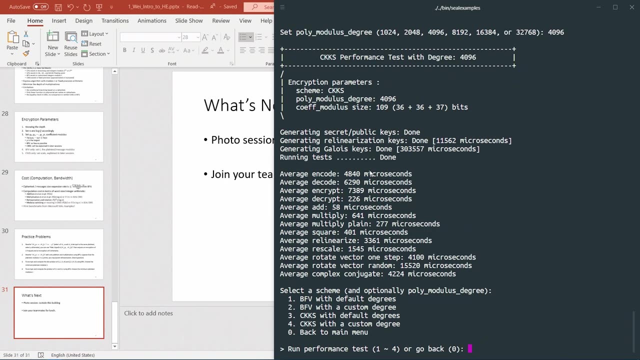 you want to select a way to measure the performance. Let's say I want to measure CKKs with the custom degree. It asks you to type in a degree, let's say 2096. It just print out the cost. I'm measuring it on a Linux subsystem. 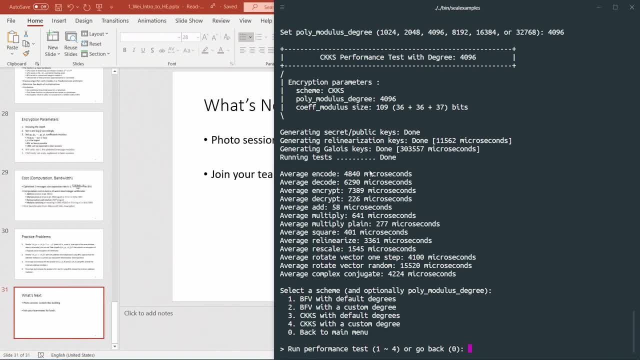 which is not the best platform to measure performance, But you can see it gives you all the results in terms of milliseconds And microsecond. you can just use them to estimate the cost And you can see multiplication linearization are fairly slow compared to additions.